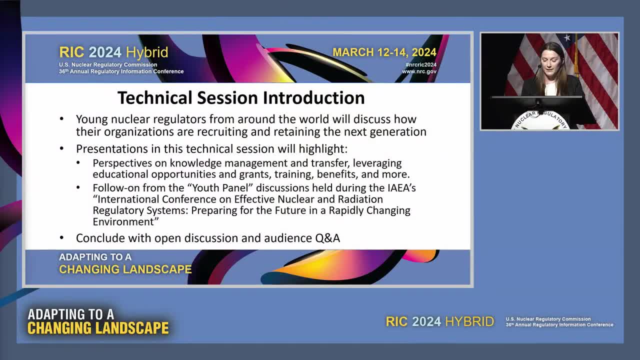 The session will also be held in person as a master of the RIC program. The presentation will highlight knowledge management, leveraging educational opportunities, training benefits and more. This discussion will also continue the conversation from the youth panel at the IAEA's International Conference on Effective Nuclear and Radiation Regulatory Systems. 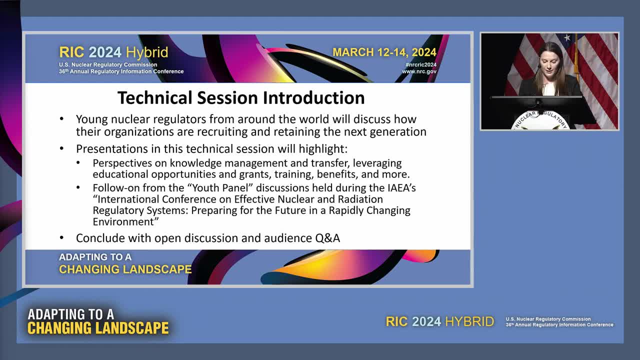 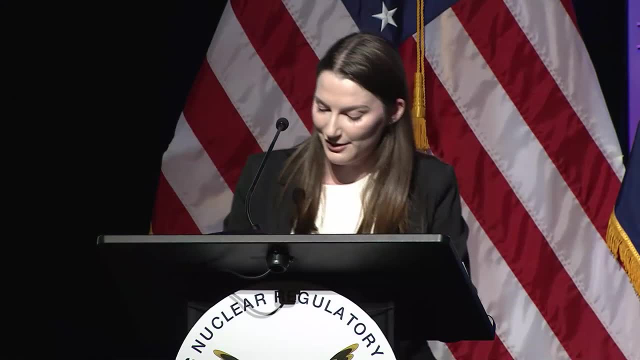 preparing for the future in a rapidly changing environment. We will begin with presentations from all the panelists before the Q&A part of the session. Now I would like to introduce our panelists. I'm Miranda Ross, a materials engineer at the NRC in the Office of Nuclear. 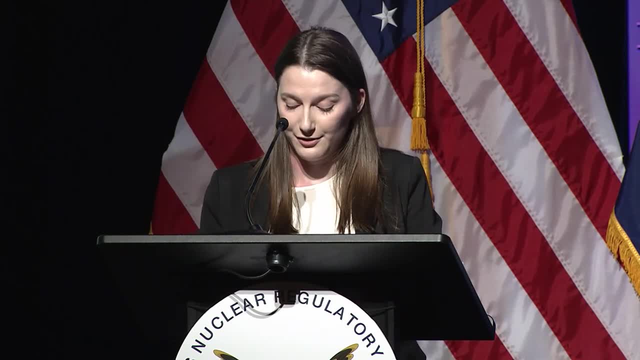 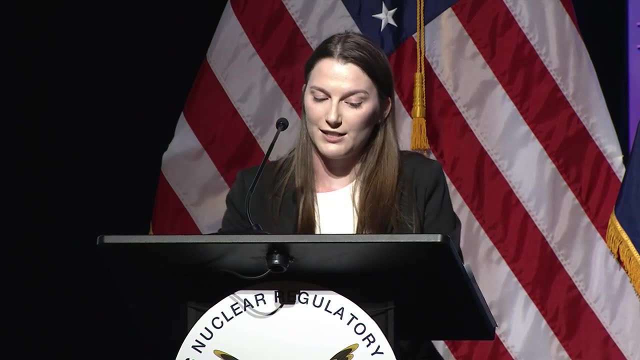 Reactor Regulation. For this session, I have the dual role of leading as the session chair and contributing my insights as a panelist. I will also provide information on the NRC's initiatives for recruiting and retaining young regulators. Joining me today is Ms Nicole Allison. 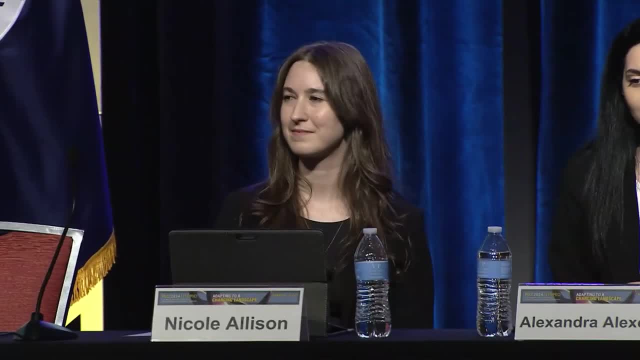 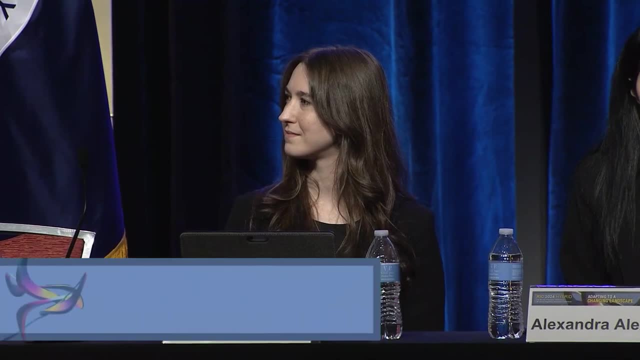 who serves as a nuclear non-proliferation officer at the Canadian Nuclear Safety Commission, CNSC. Nicole began her career with CNSC in 2017 as a technical co-op student. Her current role as a nuclear non-proliferation officer began. 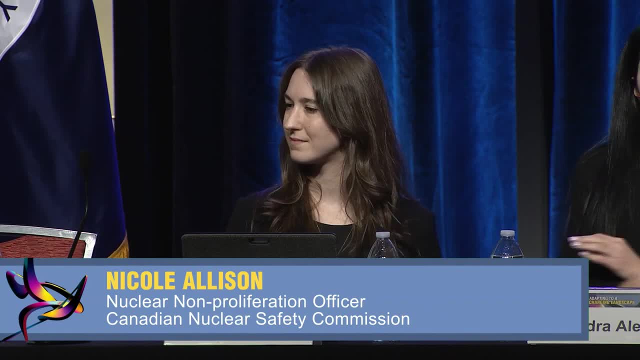 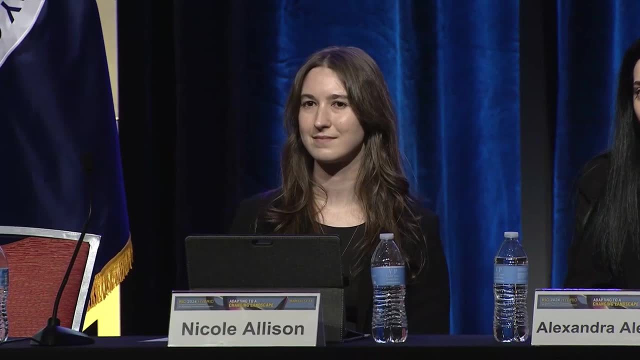 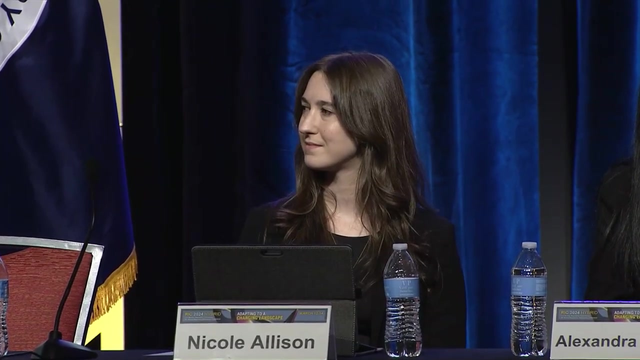 in 2019, following the completion of a nuclear engineering undergraduate program at the University of Ontario Institute of Technology, where she earned a Bachelor of Engineering in Nuclear Engineering. Nicole's work includes conducting risk-informed reviews of import and export license applications for proliferation-sensitive nuclear commodities. 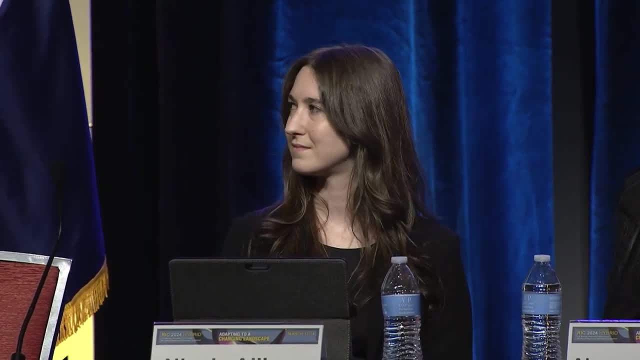 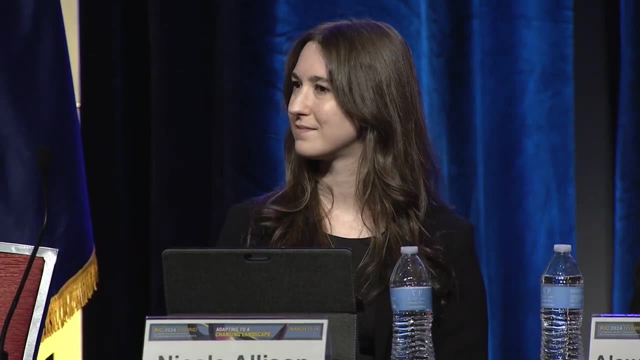 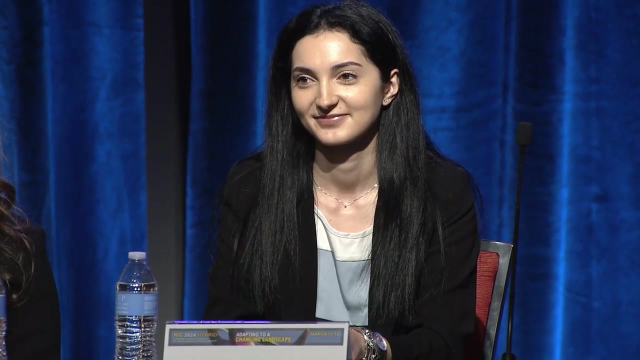 supporting the implementation of Canada's bilateral nuclear cooperation agreements and providing technical advice in various international non-proliferation fora. Next will be Ms Alexandra Alexoia, a junior nuclear advisor from the Romanian National Commission for Nuclear Activities Control, CNCAN. 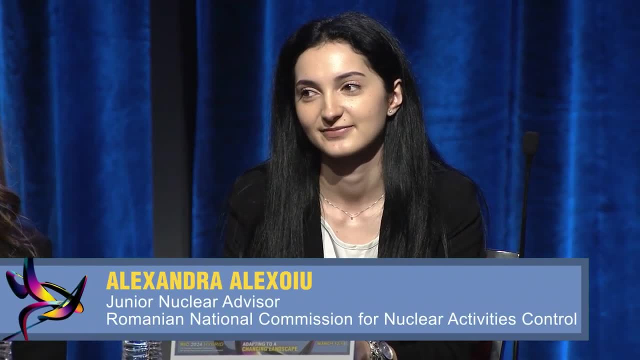 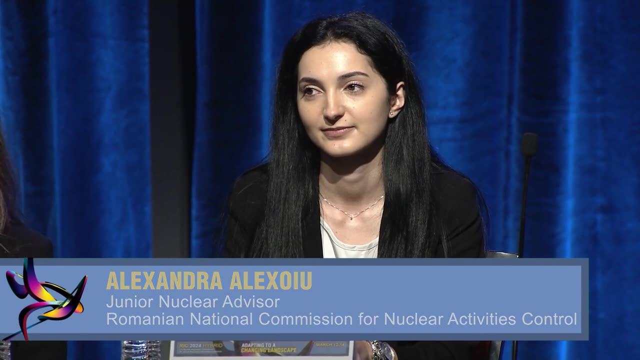 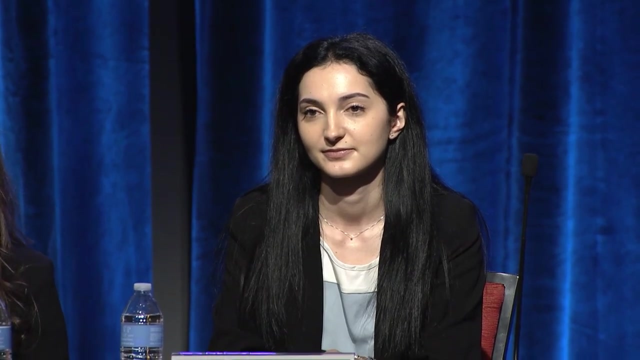 Alexandra began working as a nuclear nuclear officer in the working as a junior nuclear advisor in 2021.. Her work is in the nuclear fuel cycle division, radiation protection, radioactive waste and transport section, where she works on regulatory reviews, licensing and control of radiation protection activities, waste management, including. 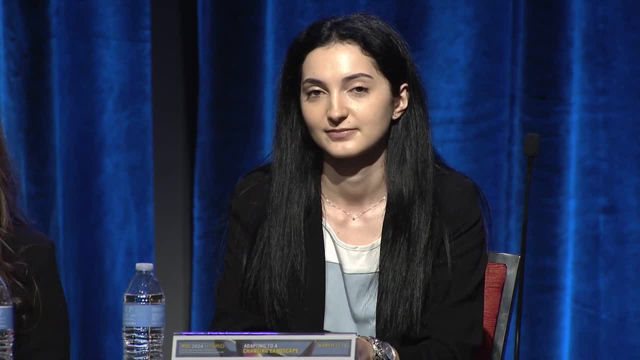 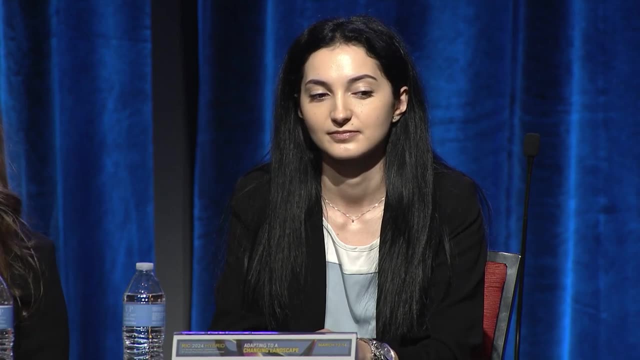 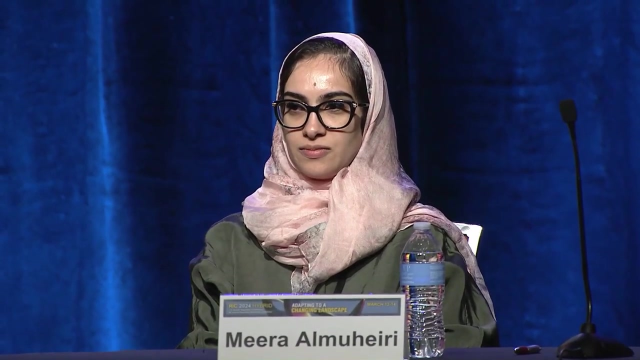 spent nuclear fuel and transport activities for installation and activities within the nuclear fuel cycle. Subsequently, we will be joined by Ms Meera El-Mahiri, a specialist inspector from the Federal Authority for Nuclear Regulation. Meera is the first Emirati female to work as a nuclear safety. 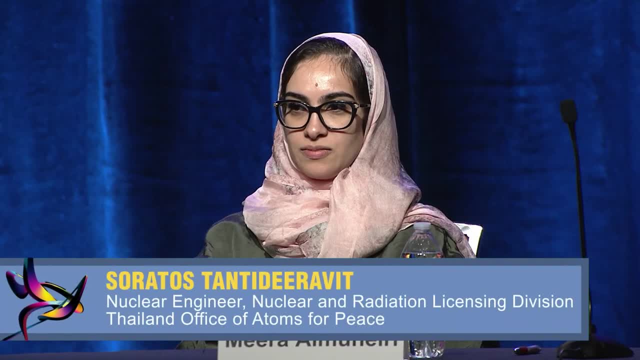 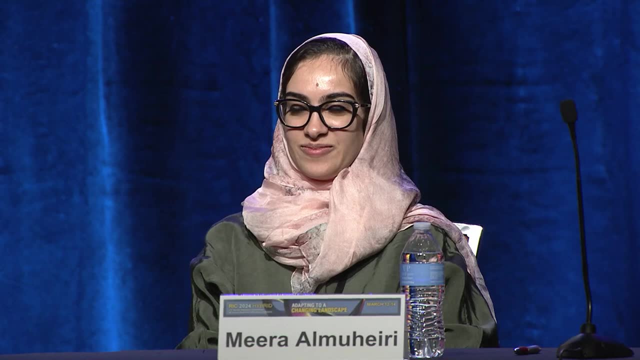 inspector in FANR and one of the youngest board members appointed to the UAE government. She received a Bachelor in Science in Mechanical and Nuclear Engineering from Khalifa University, a Master of Arts in International Affairs from King's College London and an Executive Diploma in Policymaking from McGill. 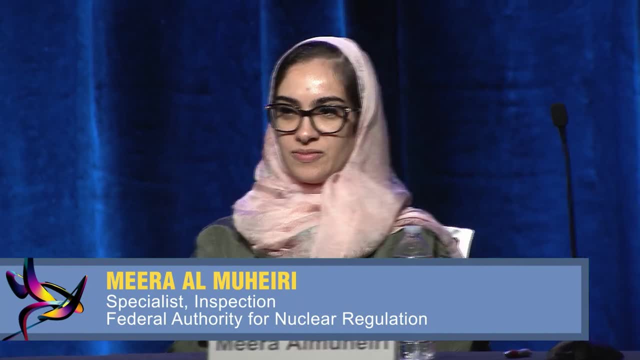 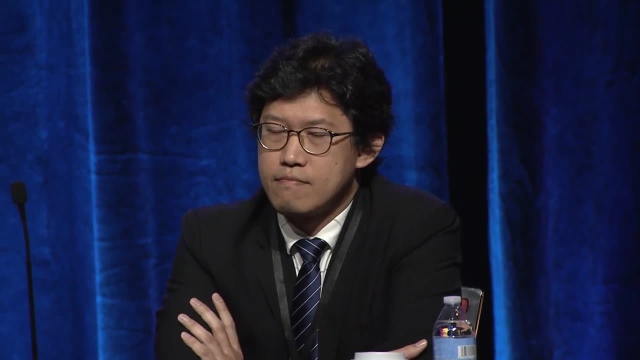 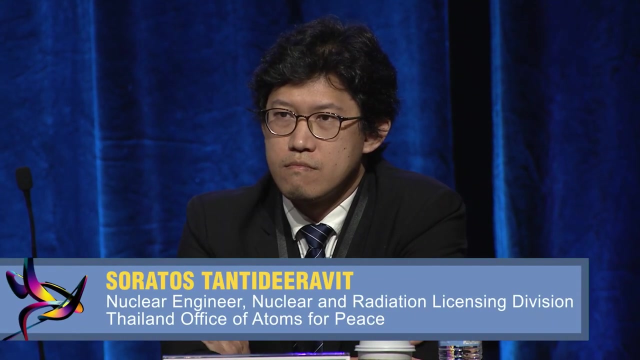 University. Last but not least, we will hear from Mr Souratos Tontadiravit, a nuclear engineer from Thailand's Office of Atoms for Peace. Souratos earned a scholarship from the Thai government for his PhD in mechanical engineering from Imperial College London and started his career in nuclear at the Office of Atoms. 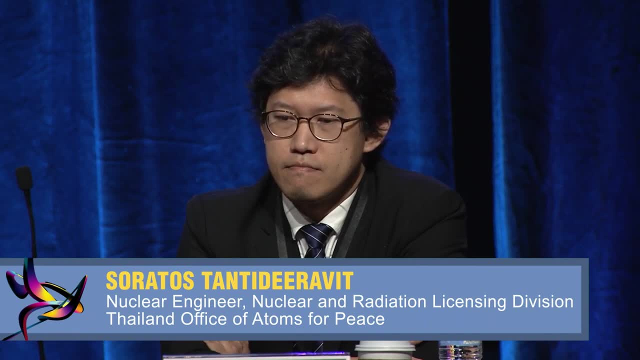 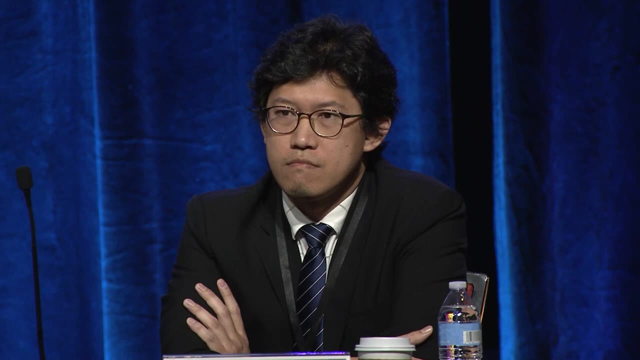 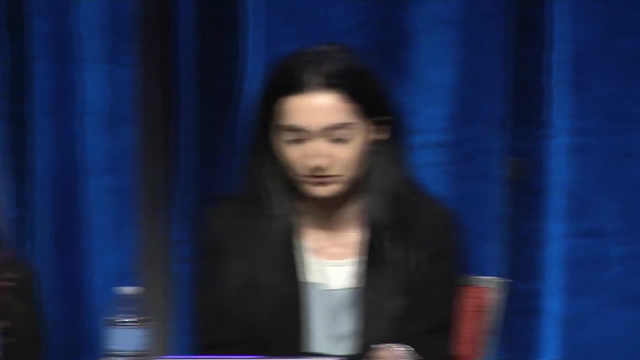 for Peace as an inspector for radiation industrial applications. His current responsibilities as a nuclear engineer in the nuclear licensing group include focus on licensing of research reactors and a national waste management facility. Additionally, he is a trainer of a radioactive source security management course for national 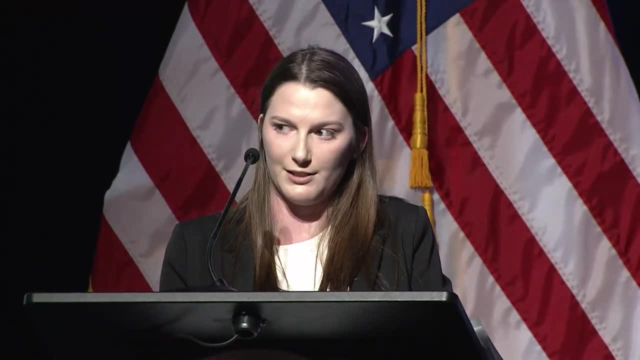 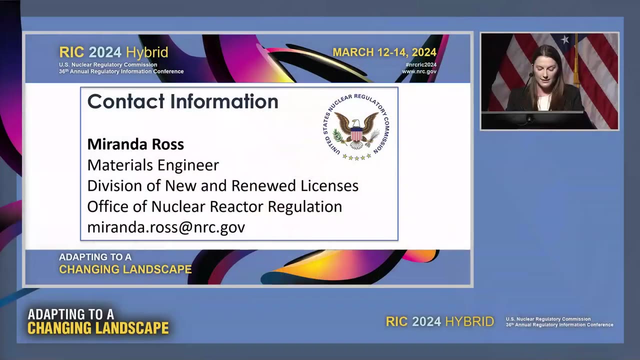 stakeholders and was given the opportunity to lead the national competency building program in the transport security of radioactive materials. As the session chair, I wanted to provide you with my contact information before we begin the presentations. I'll now join the panel and we'll get started with the presentations. 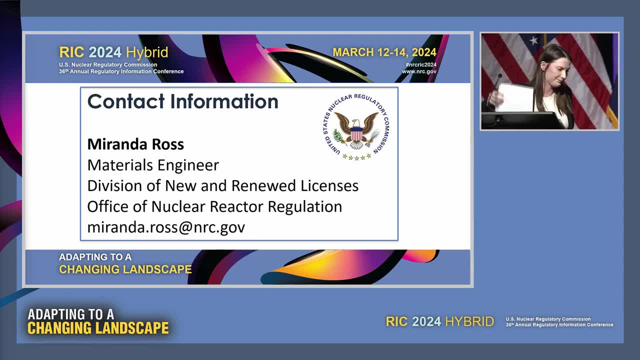 starting with mine. Souratos Tontadiravit, Director, National Stakeholder for Nuclear Safety and Nuclear Engineering. Souratos Tontadiravit, Director National Stakeholder for Nuclear Safety and Nuclear Engineering. Souratos Tontadiravit, Director National Stakeholder for Nuclear Safety and Nuclear. 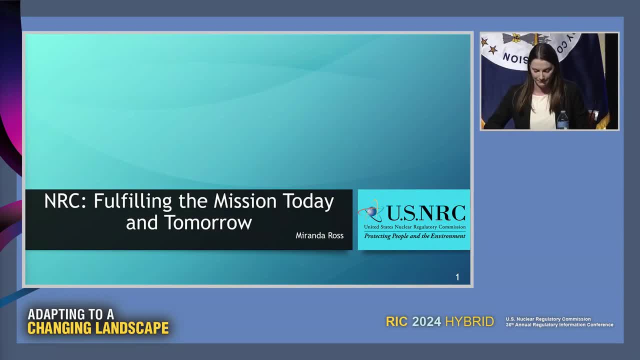 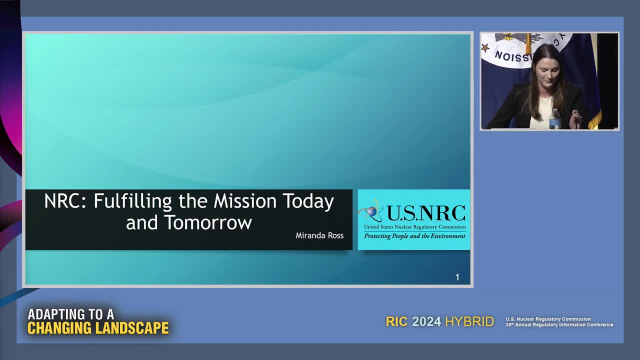 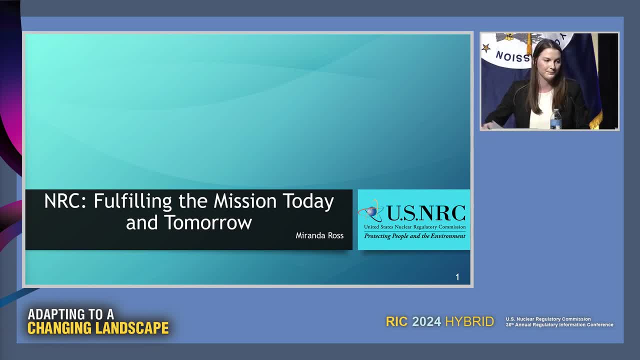 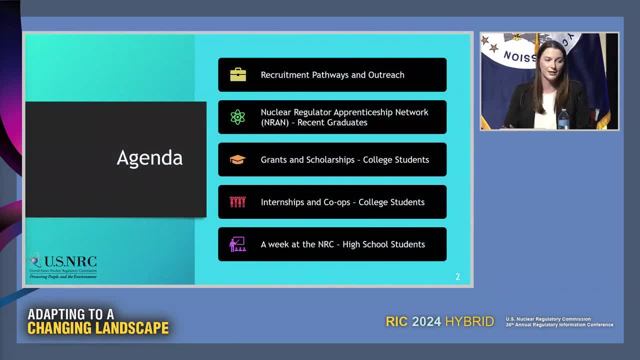 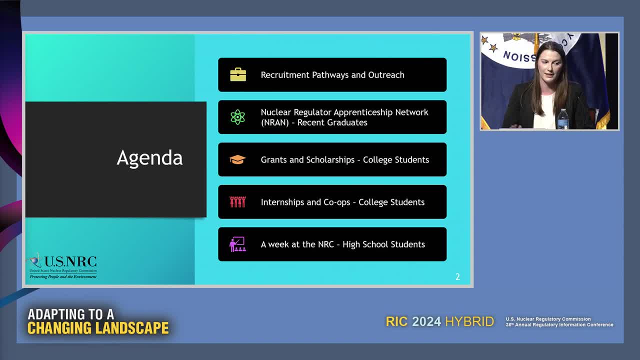 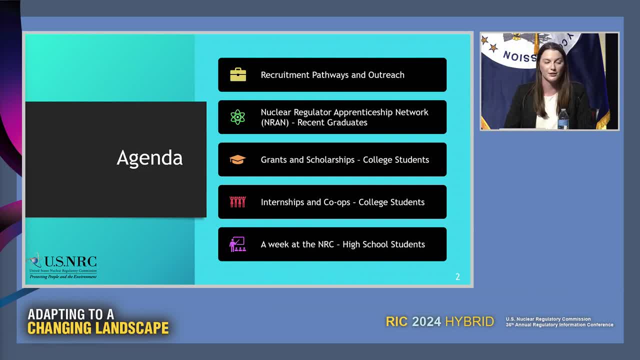 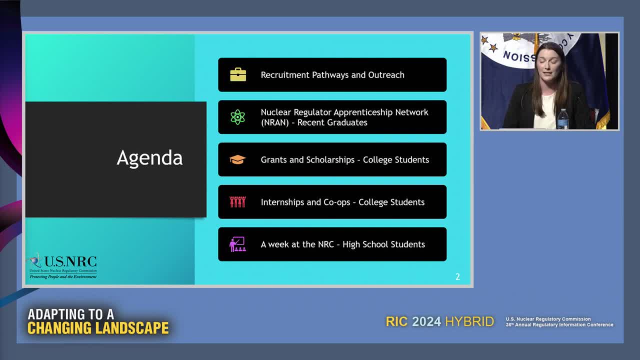 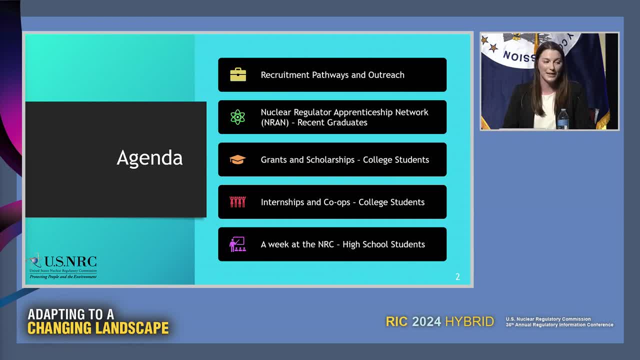 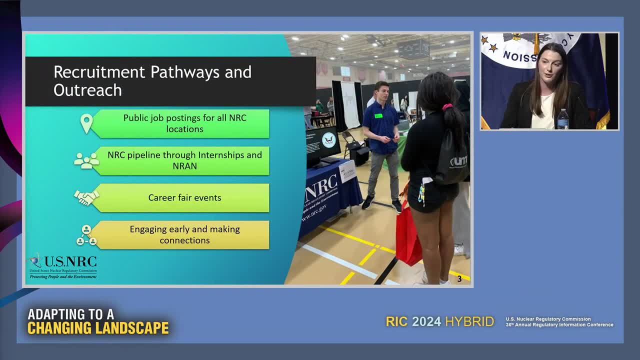 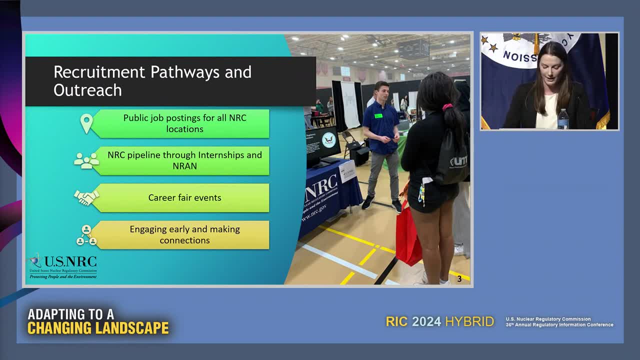 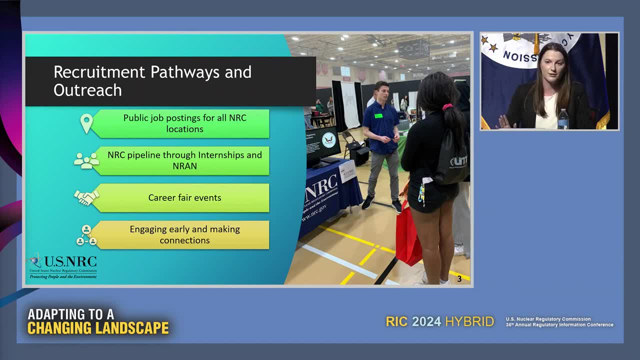 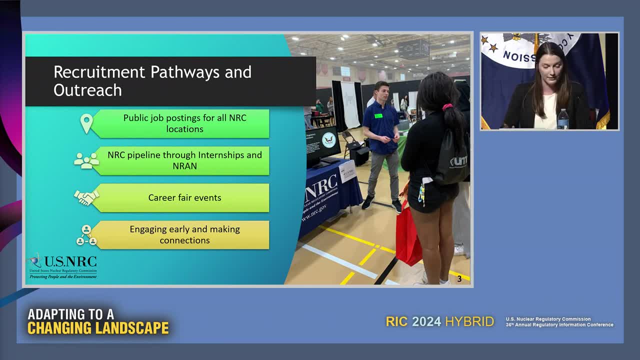 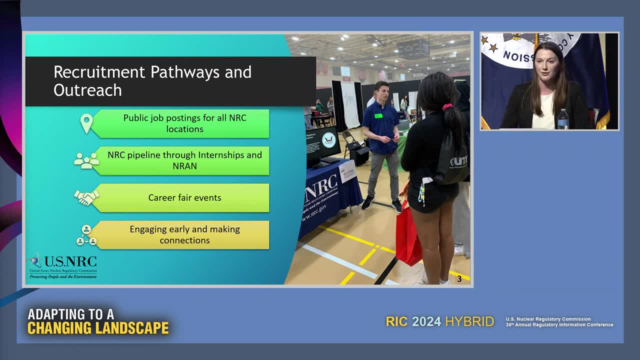 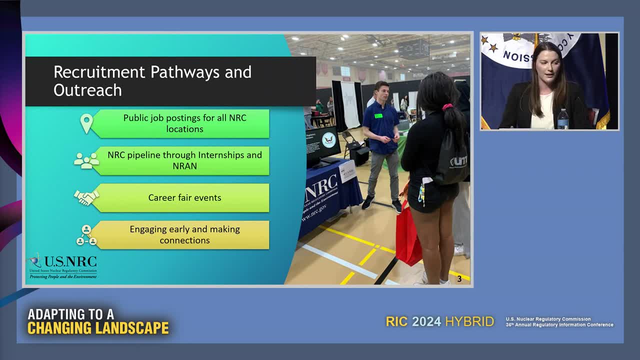 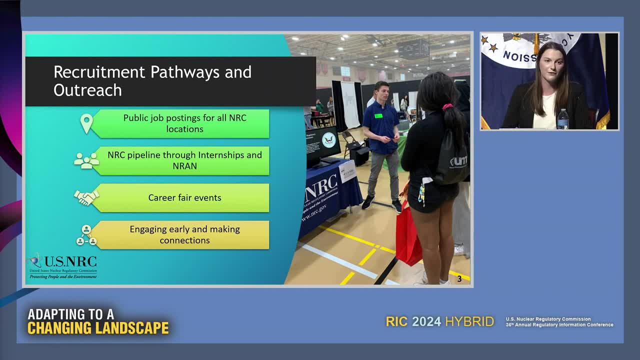 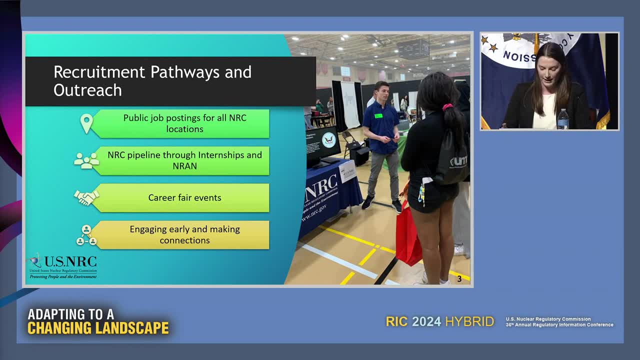 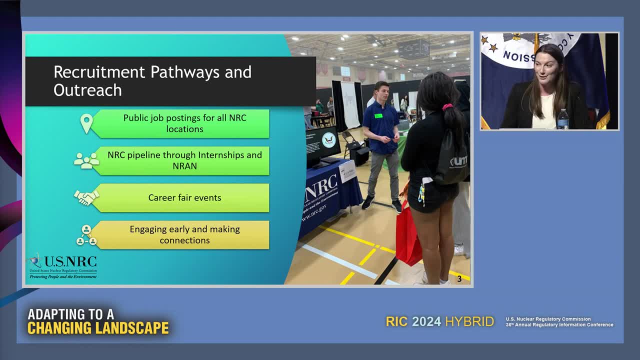 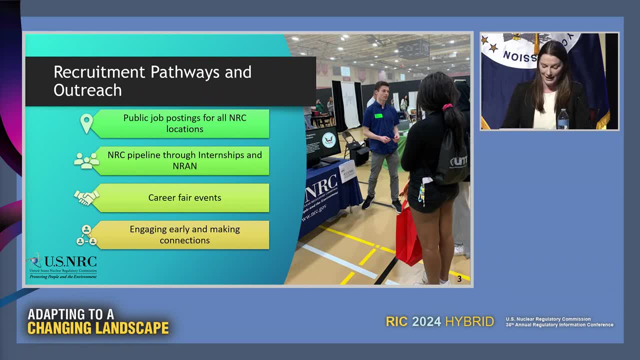 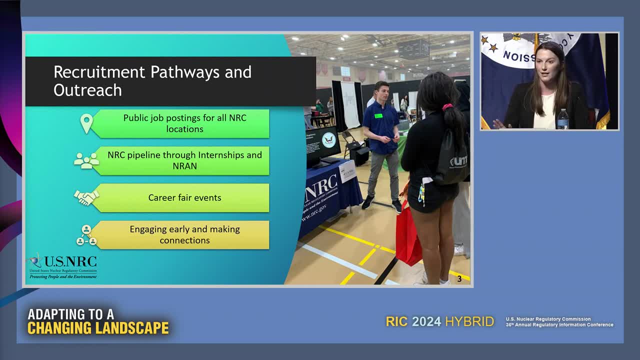 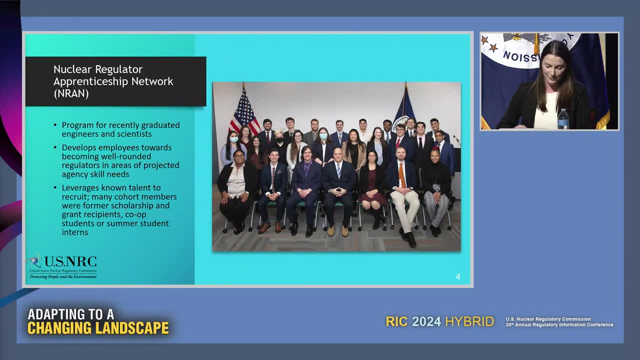 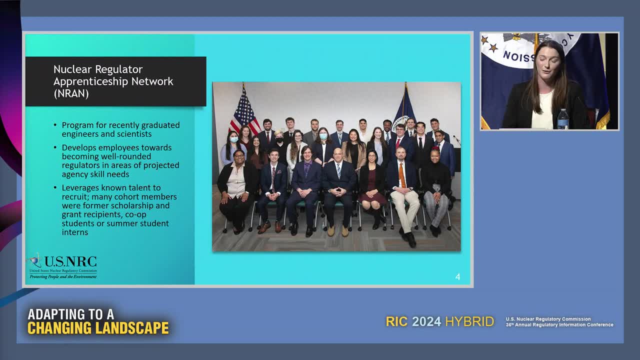 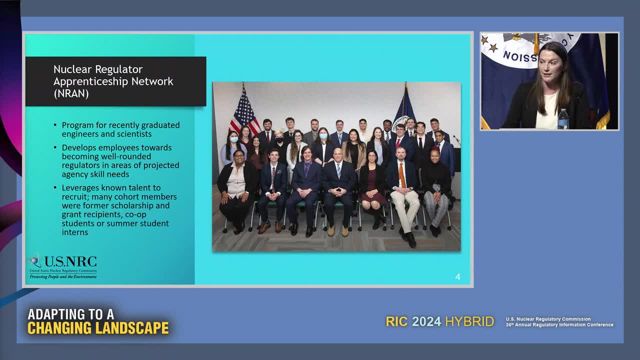 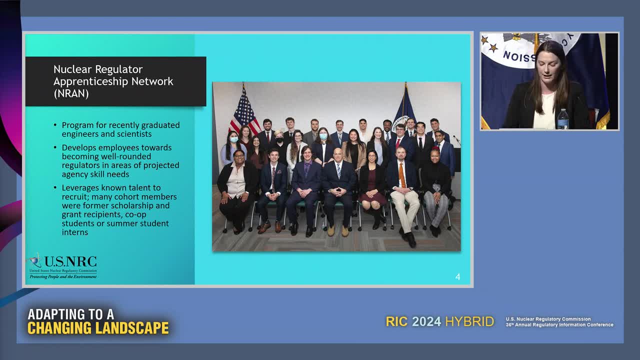 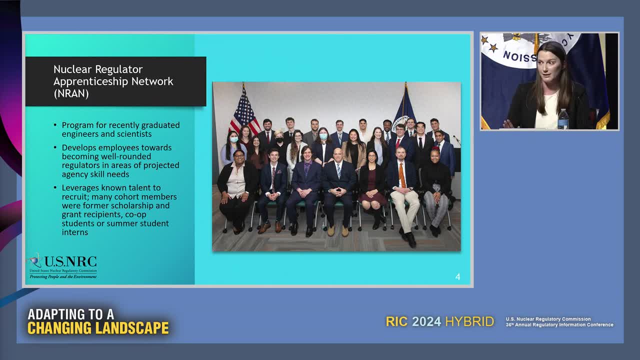 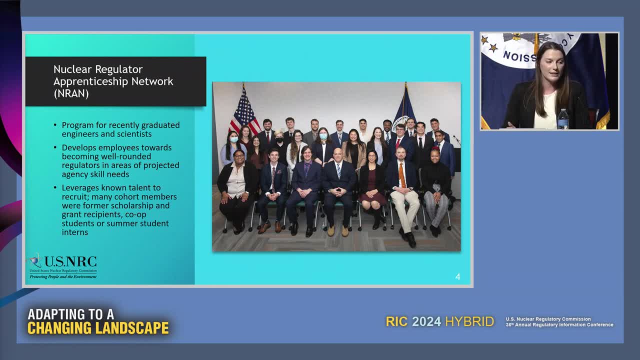 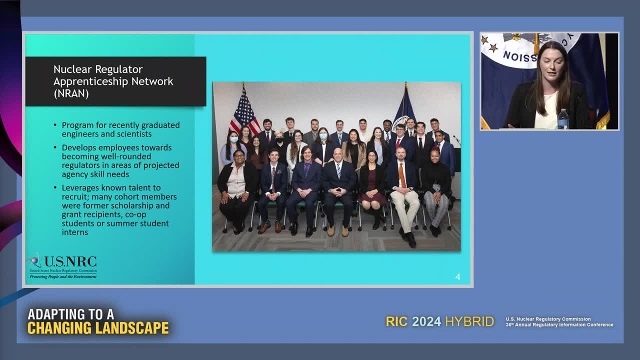 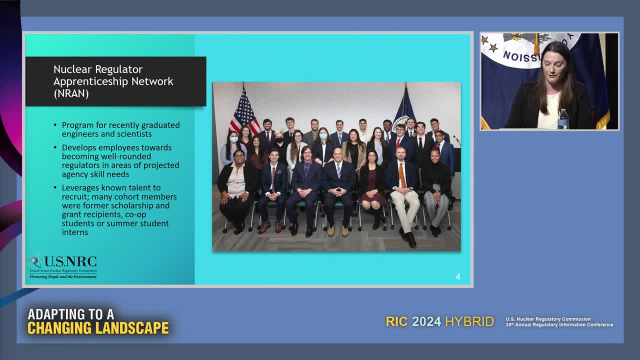 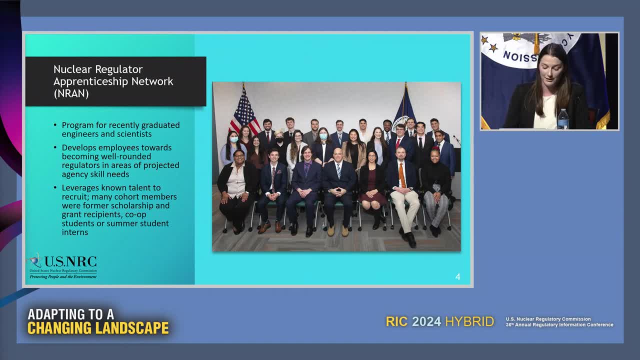 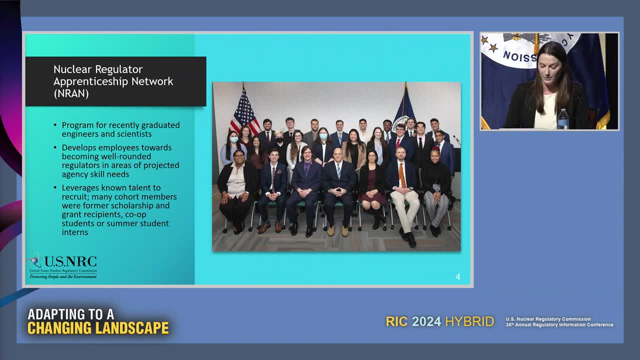 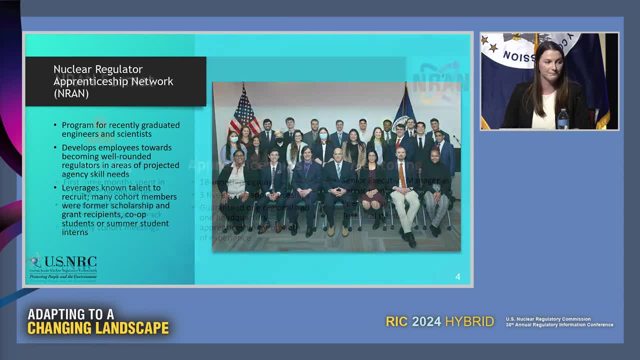 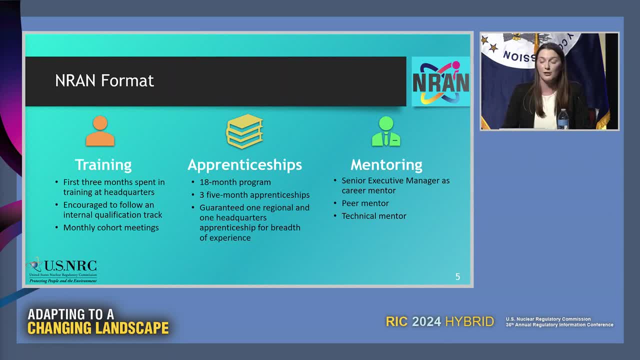 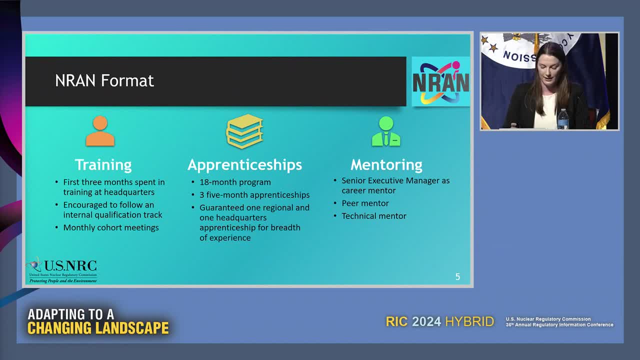 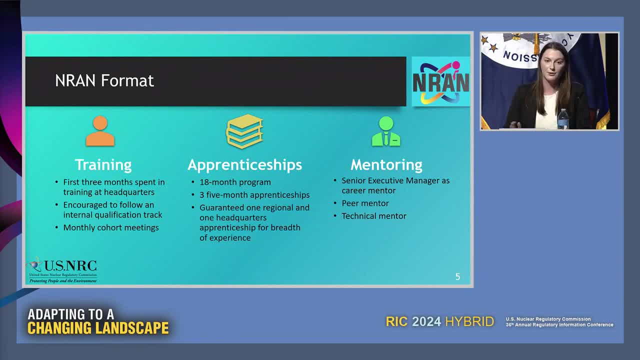 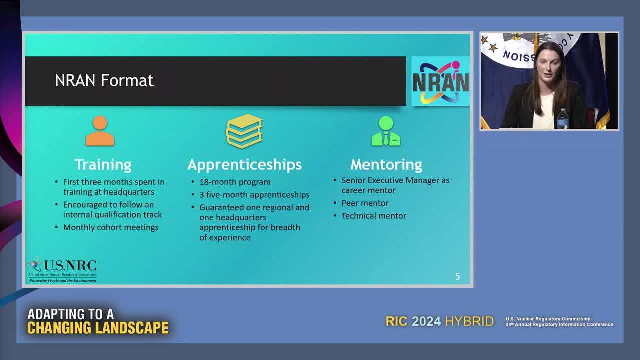 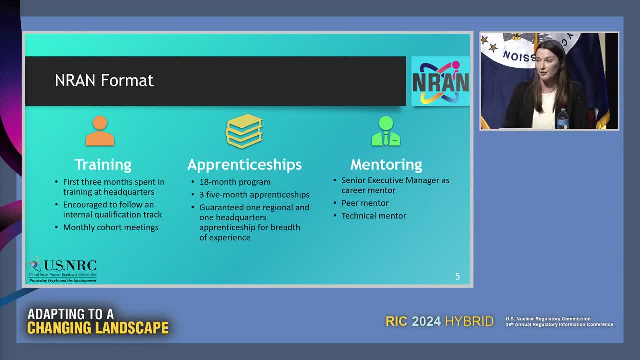 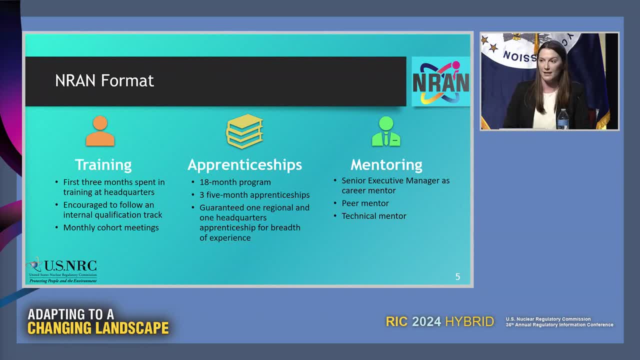 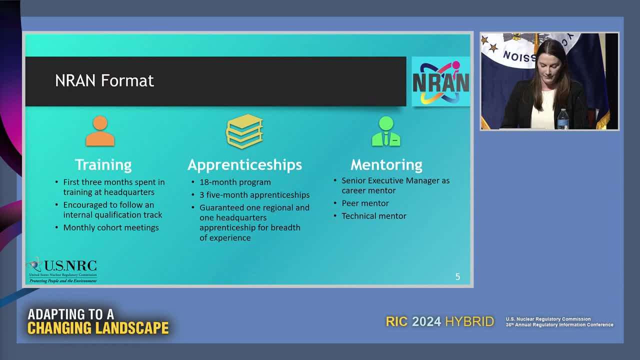 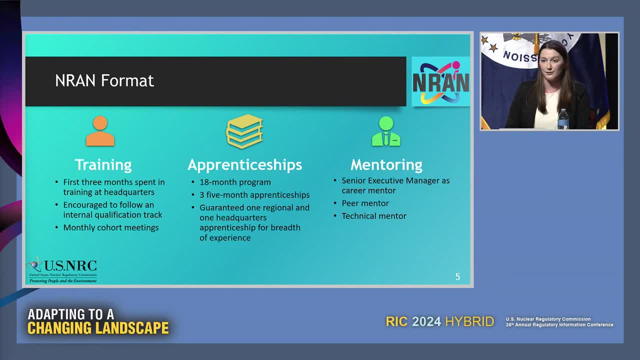 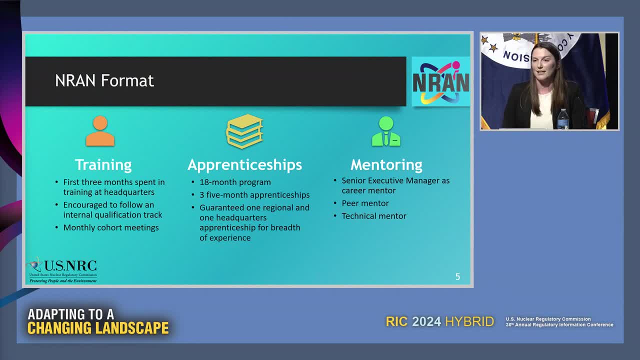 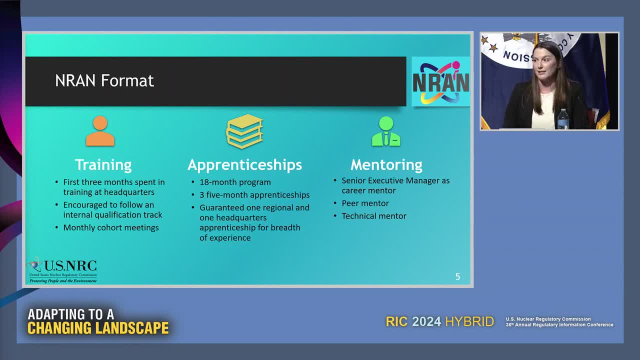 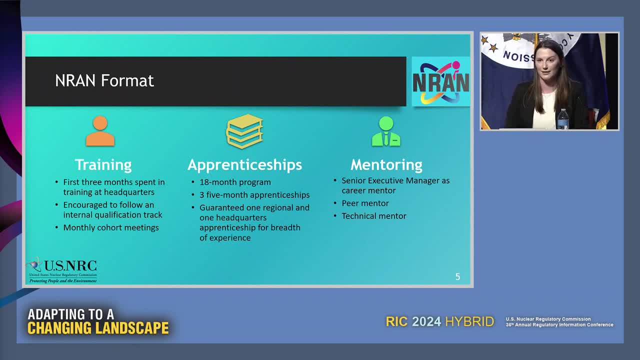 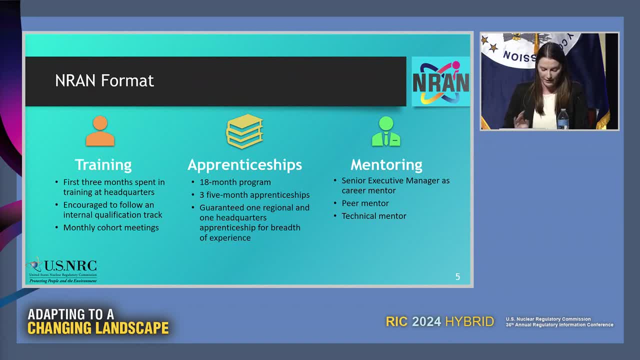 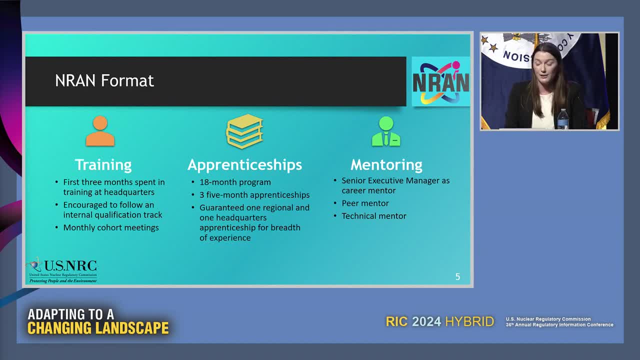 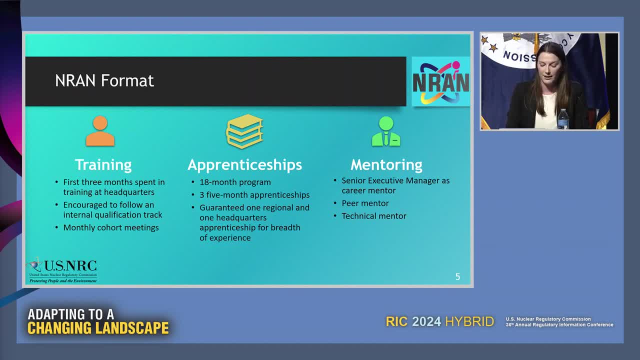 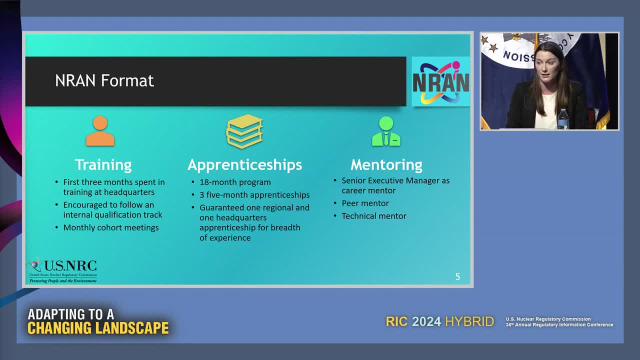 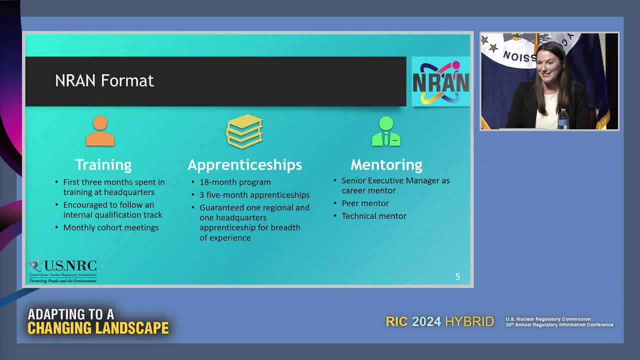 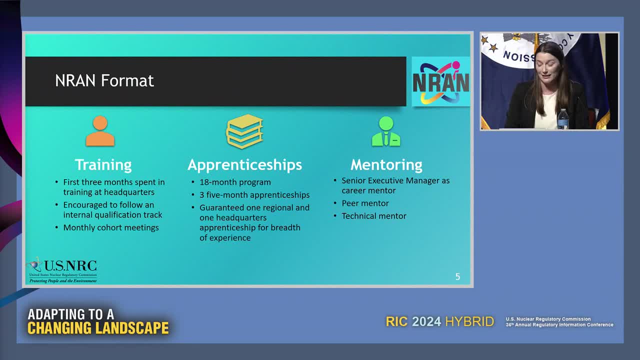 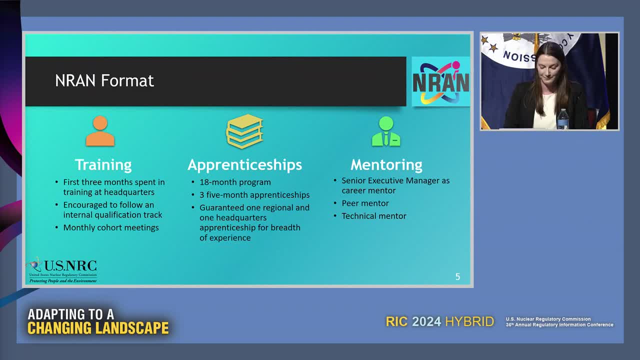 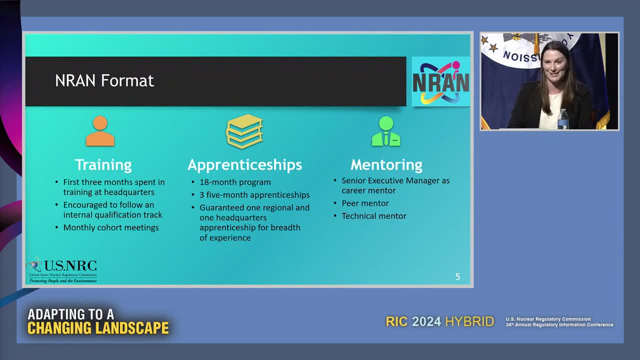 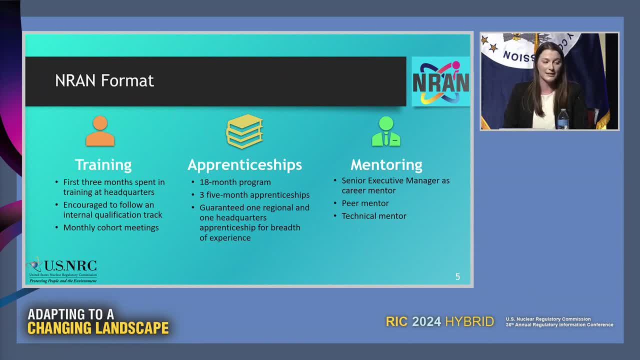 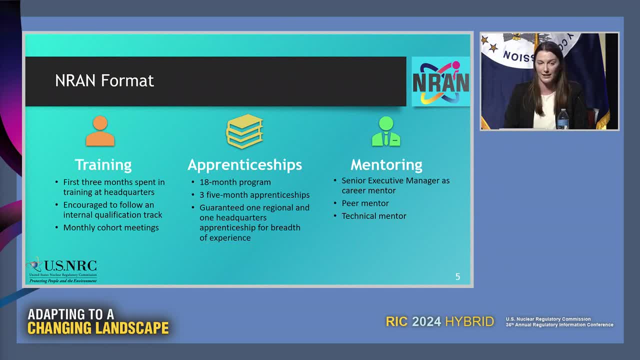 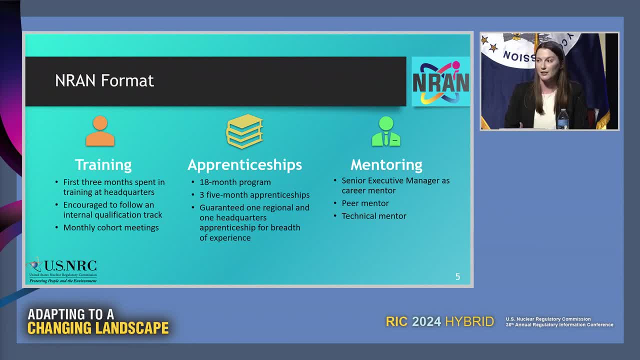 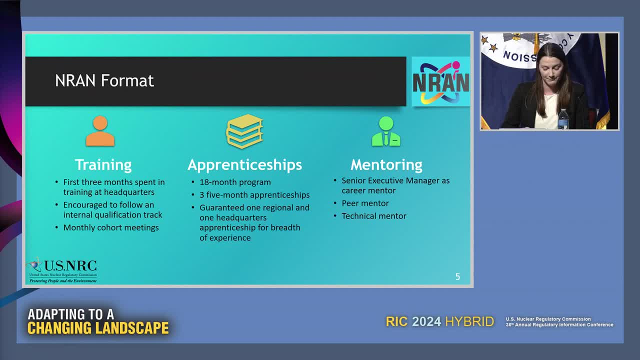 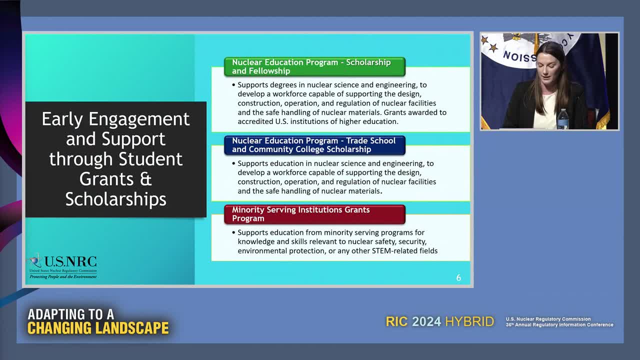 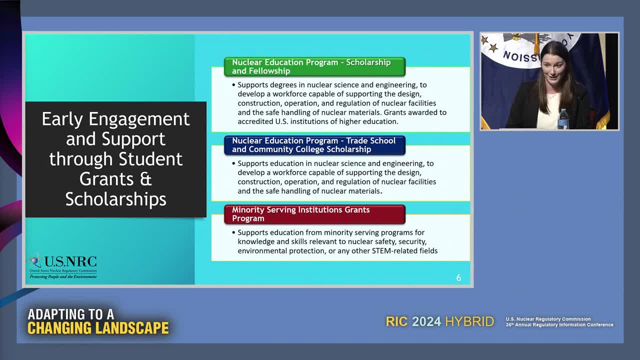 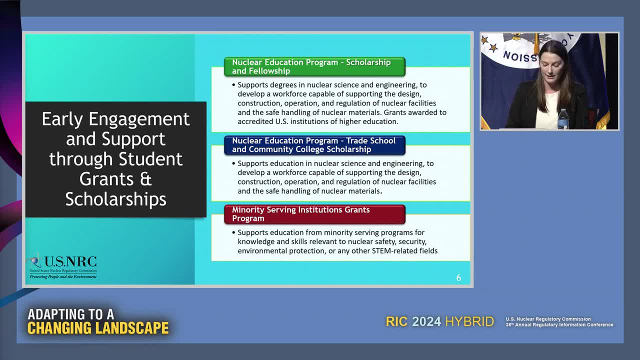 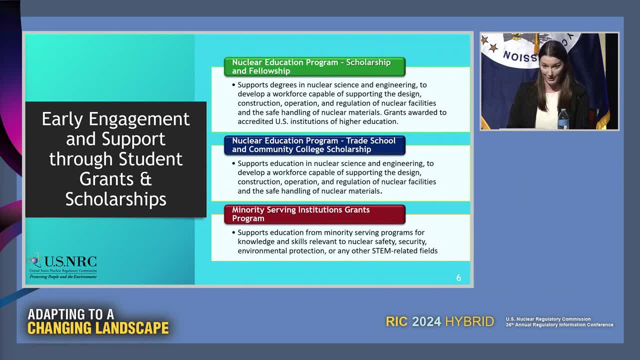 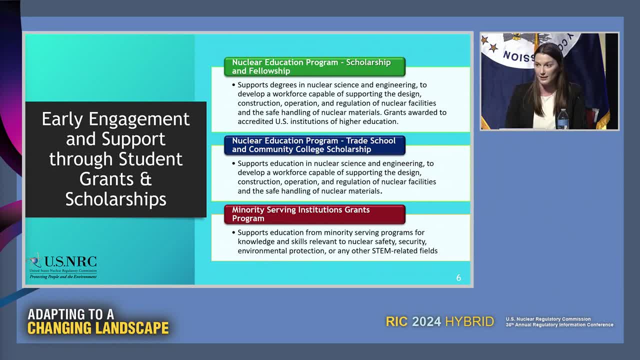 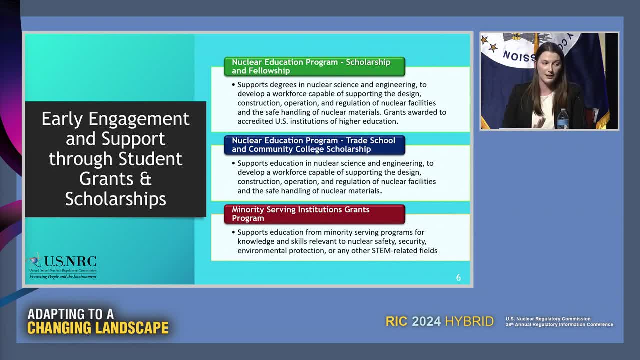 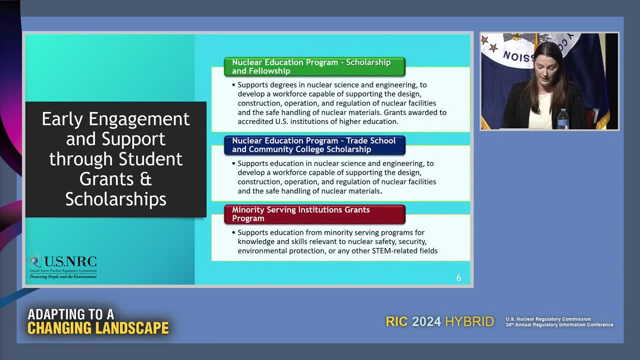 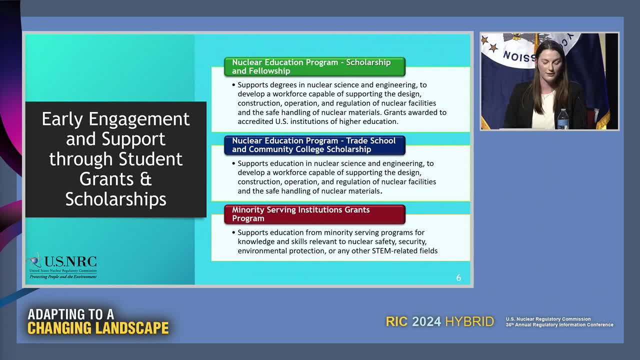 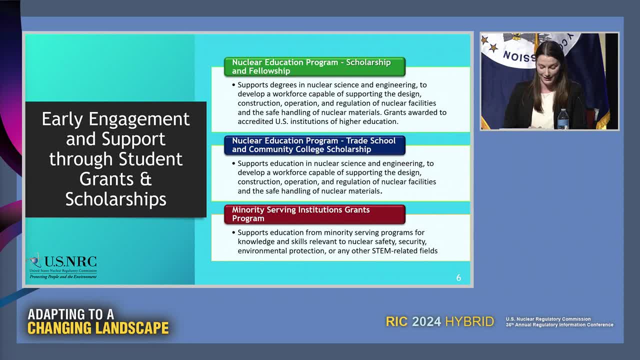 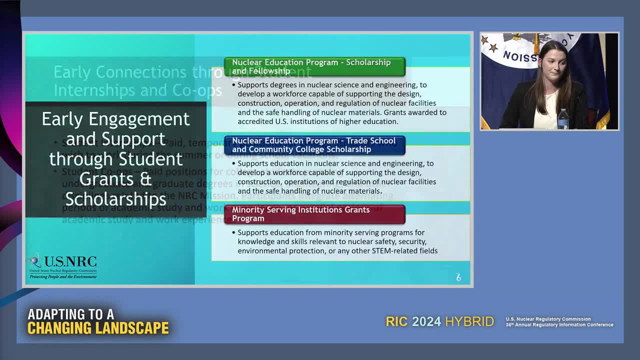 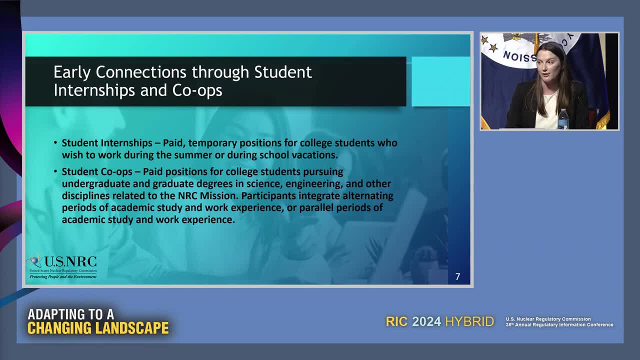 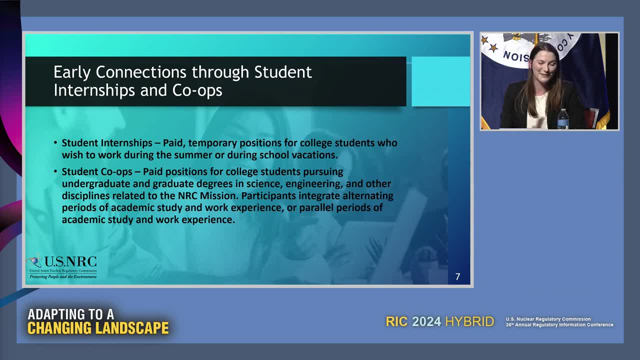 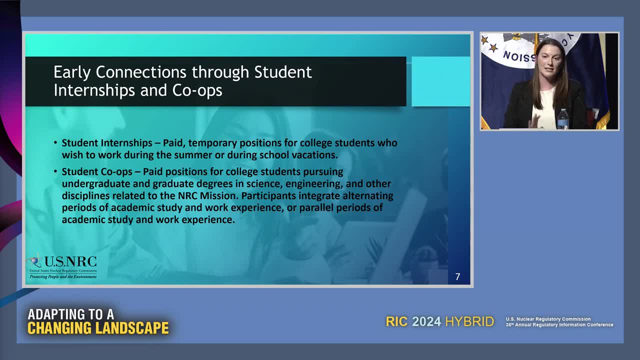 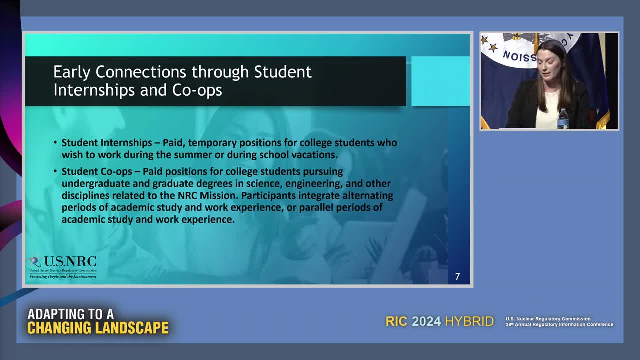 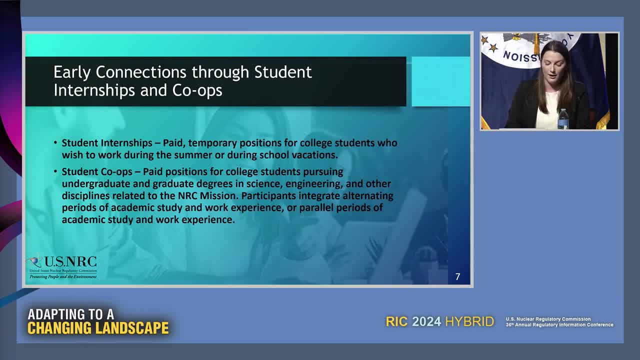 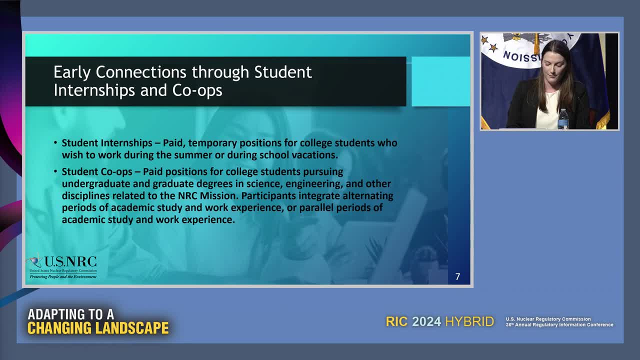 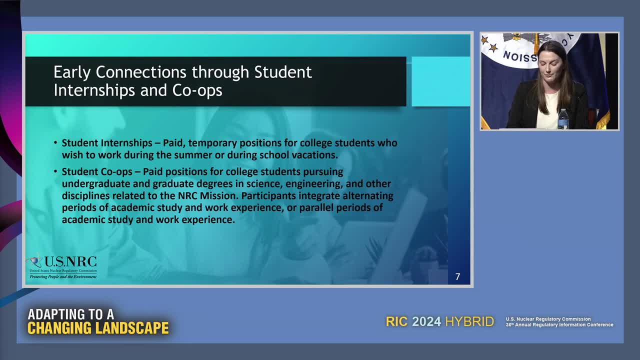 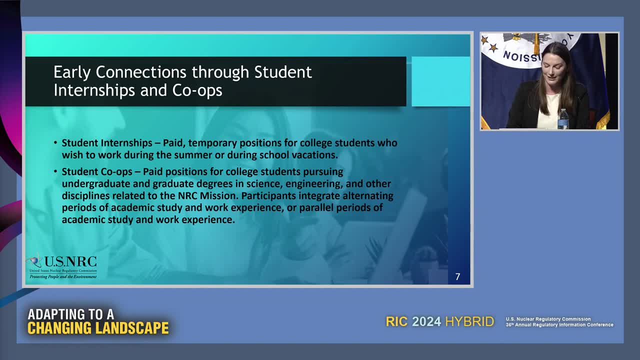 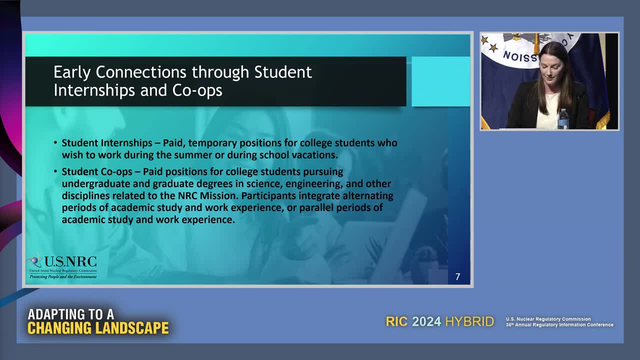 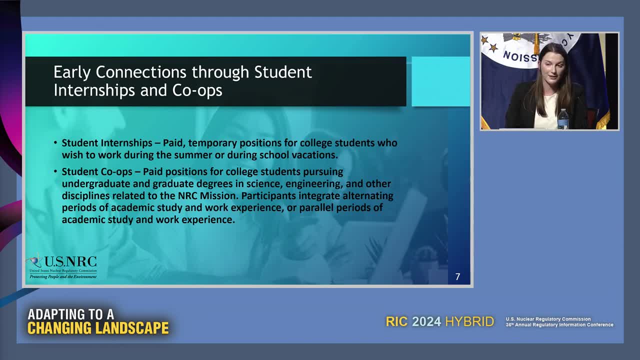 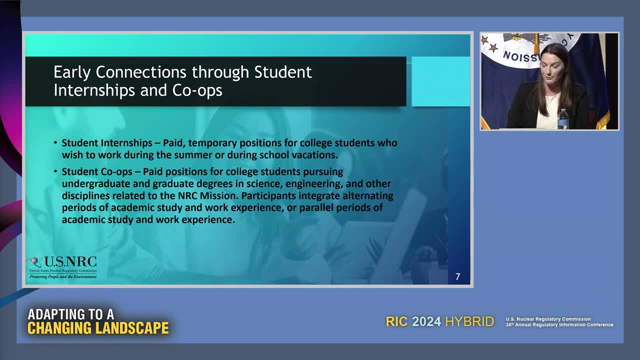 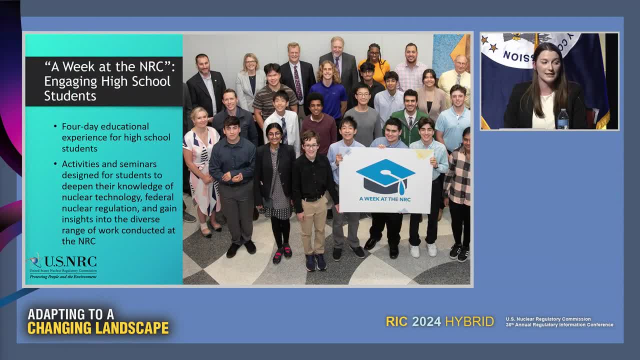 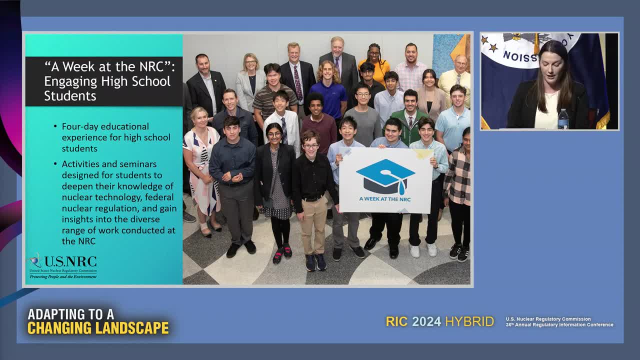 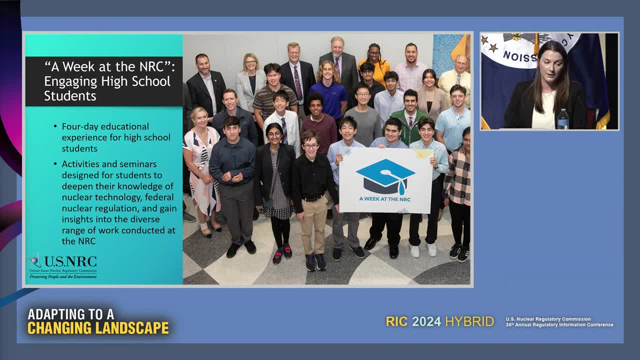 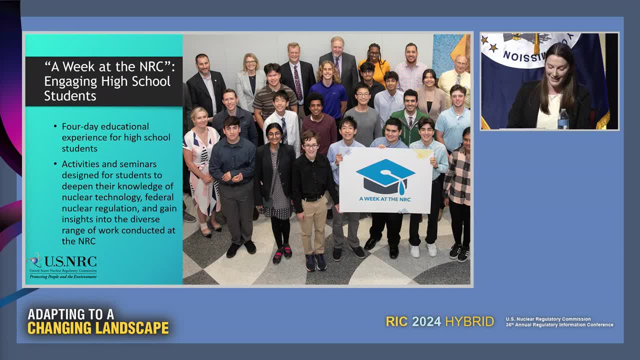 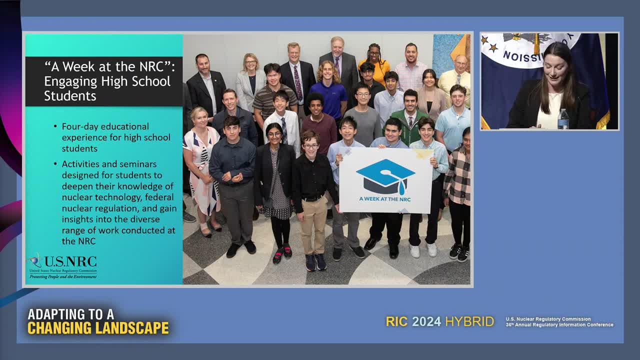 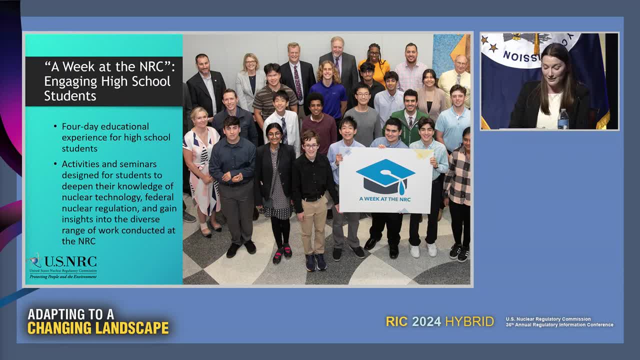 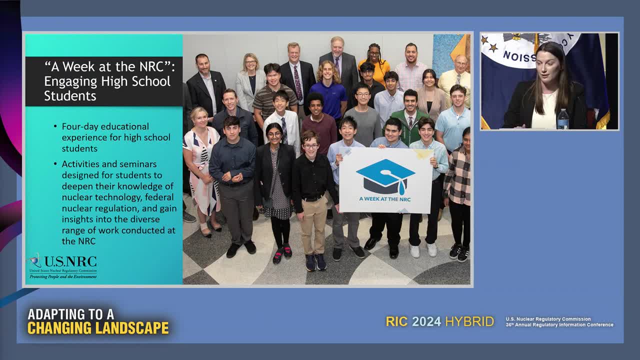 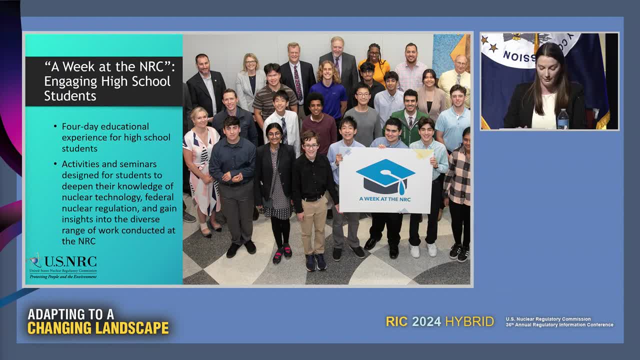 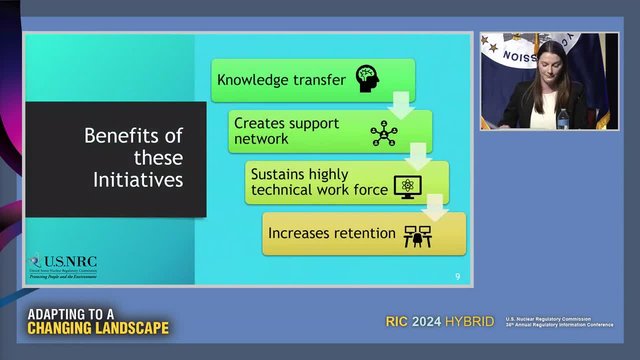 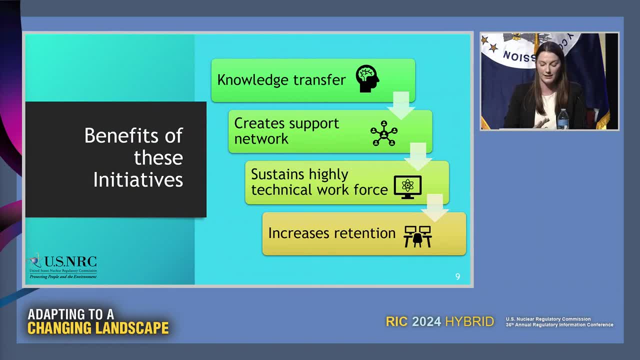 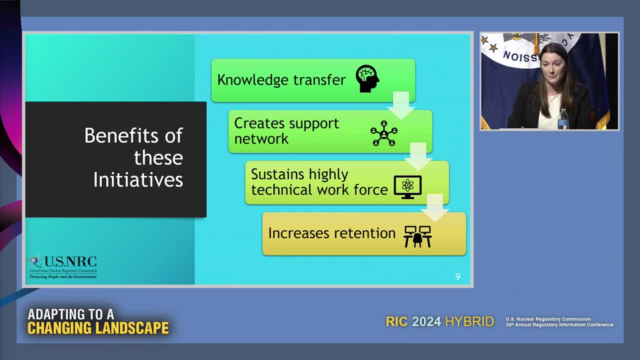 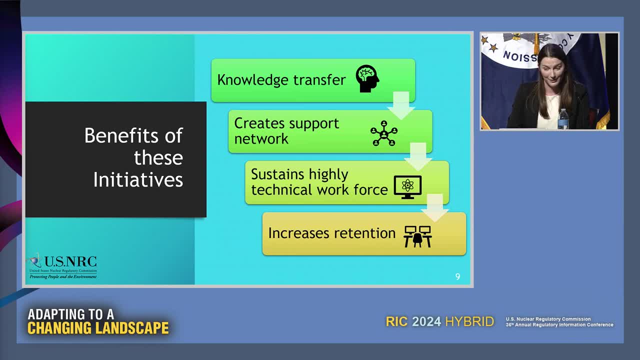 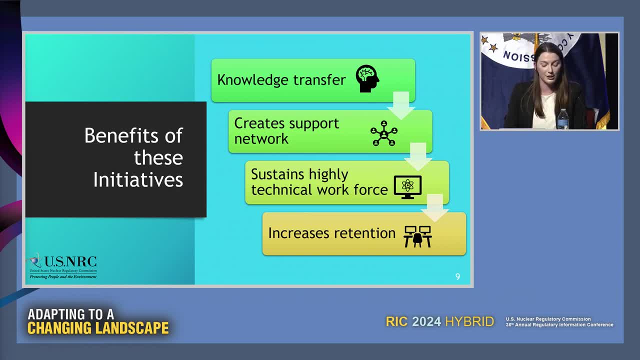 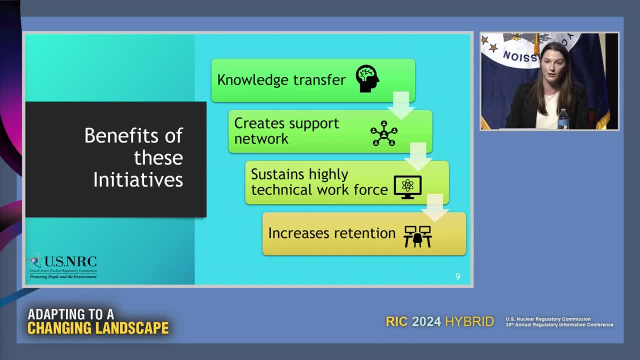 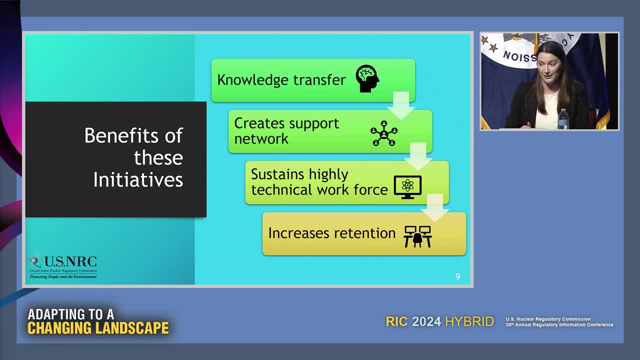 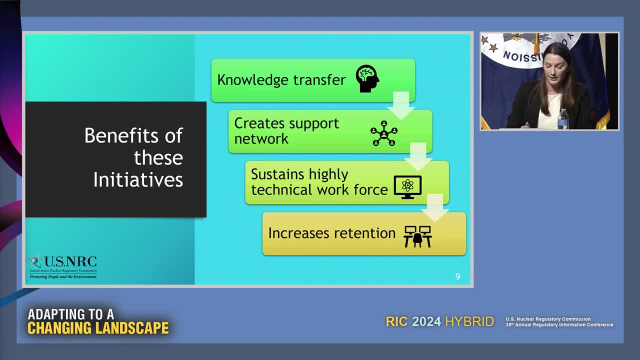 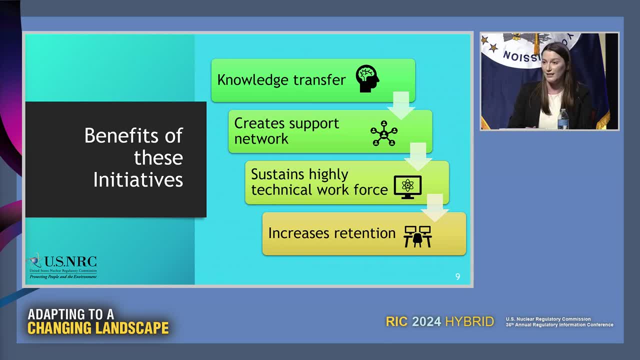 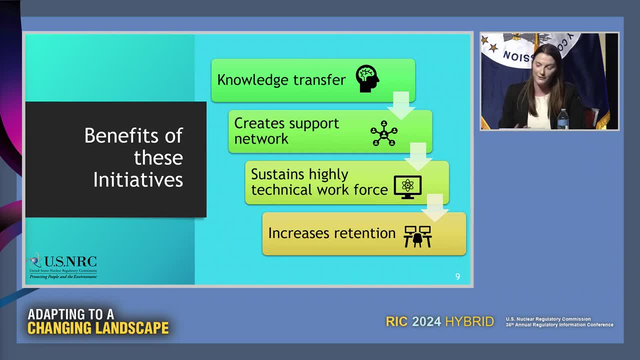 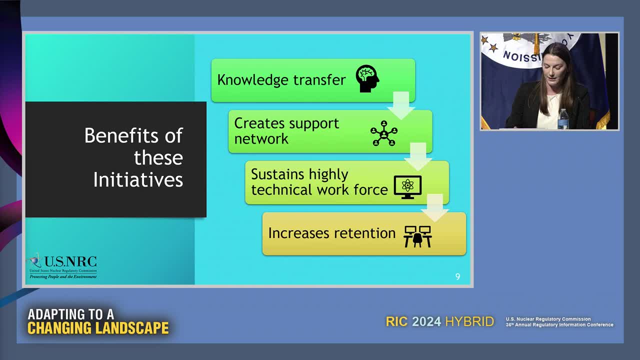 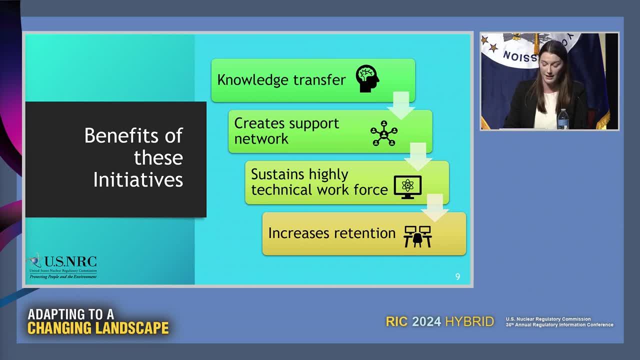 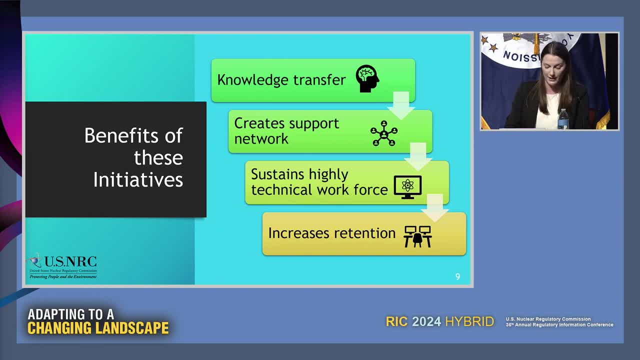 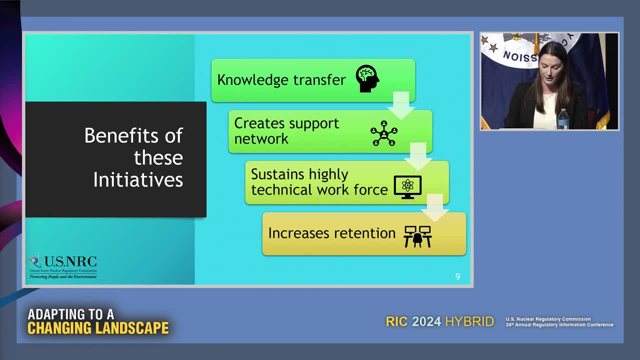 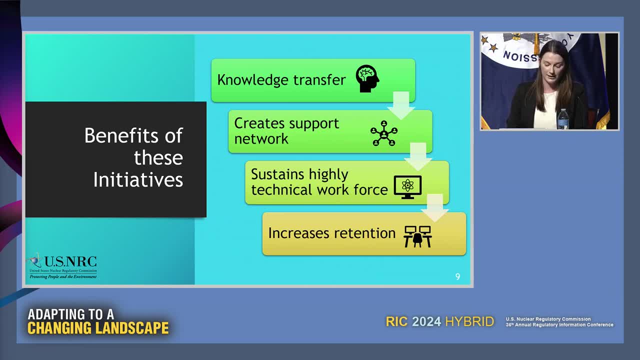 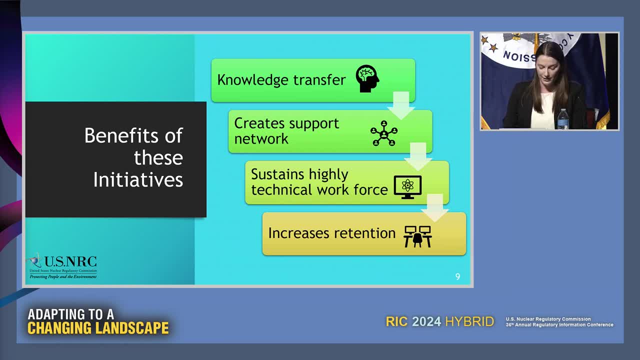 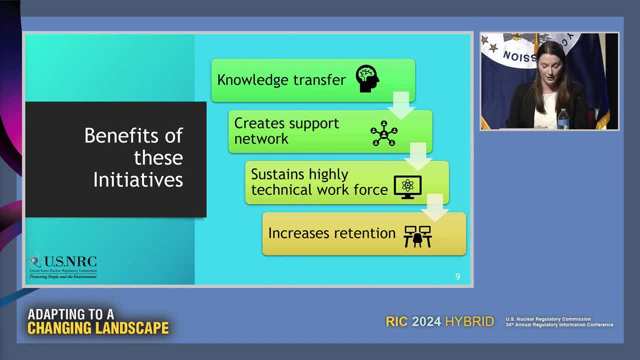 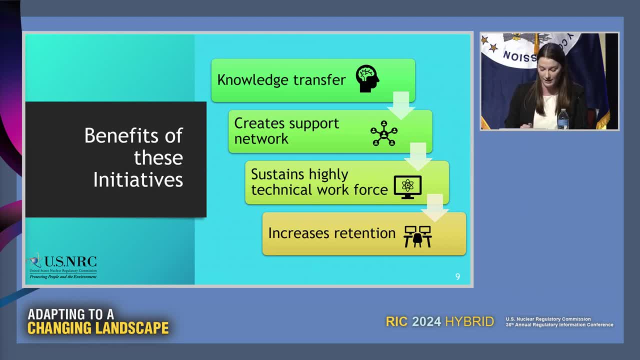 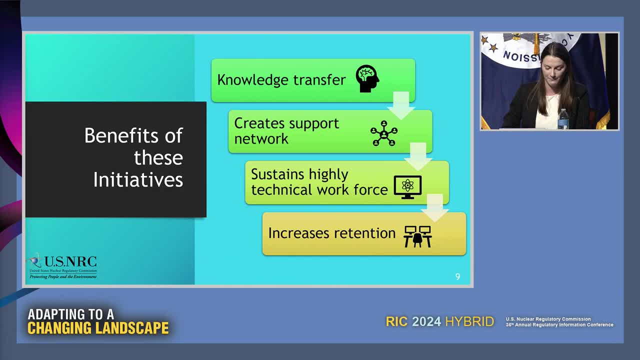 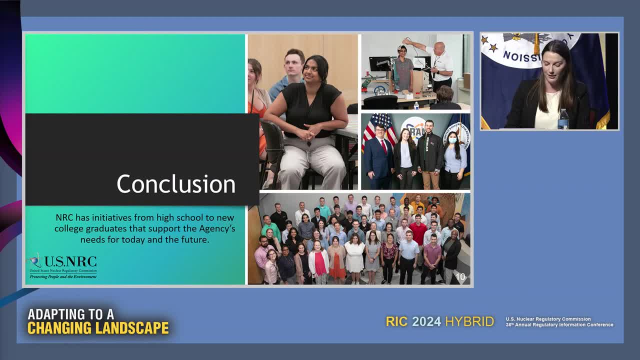 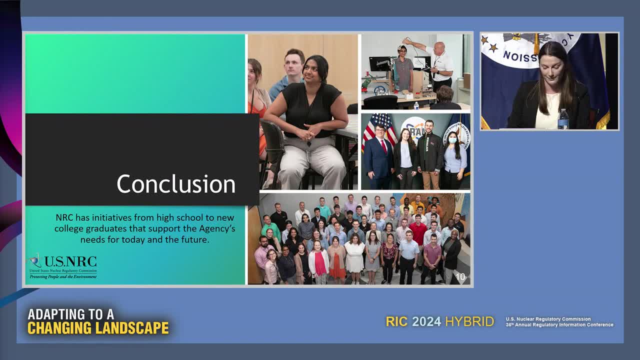 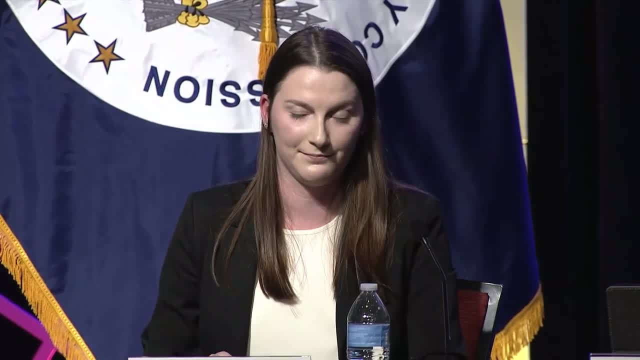 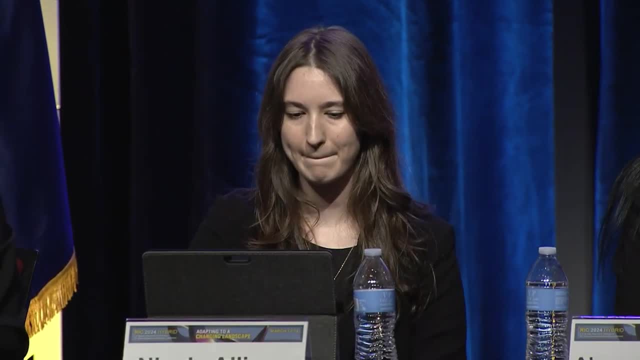 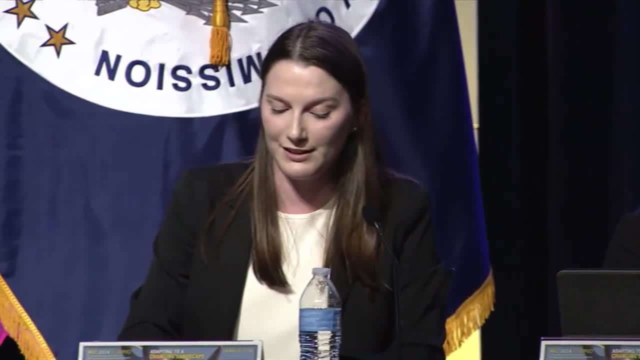 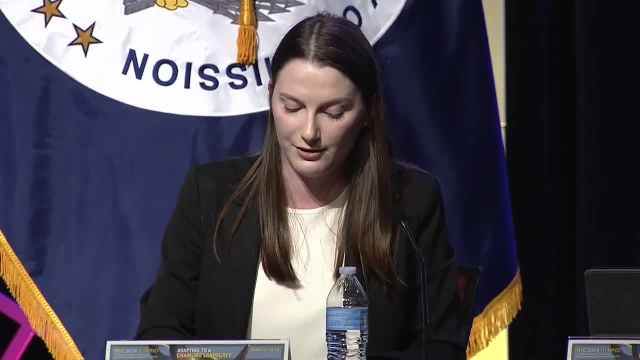 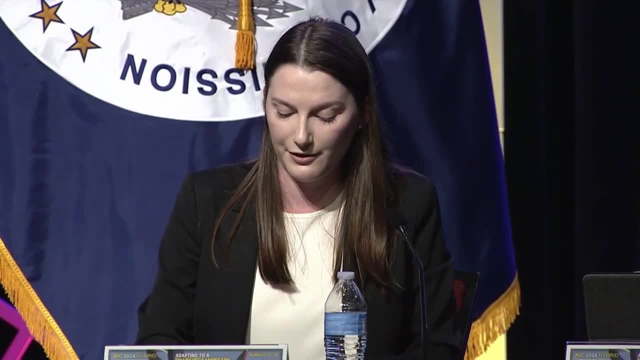 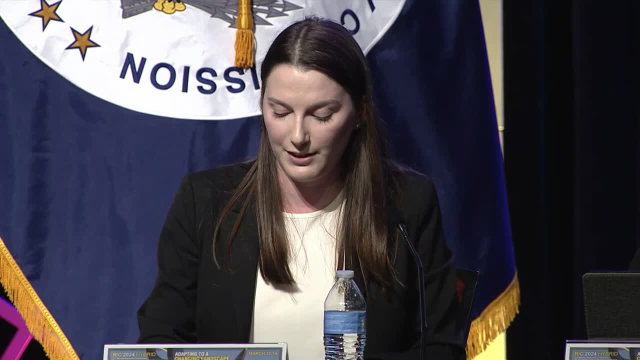 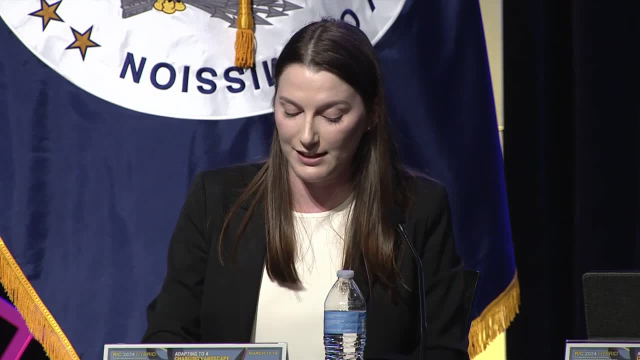 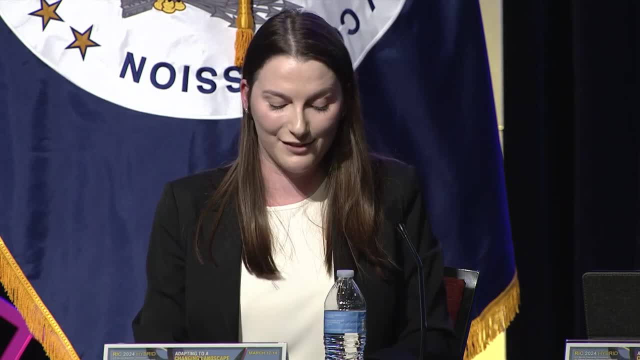 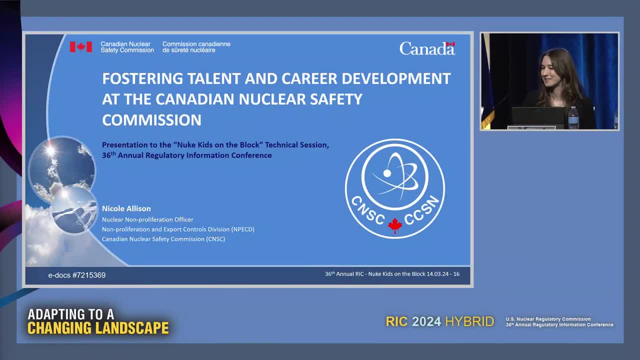 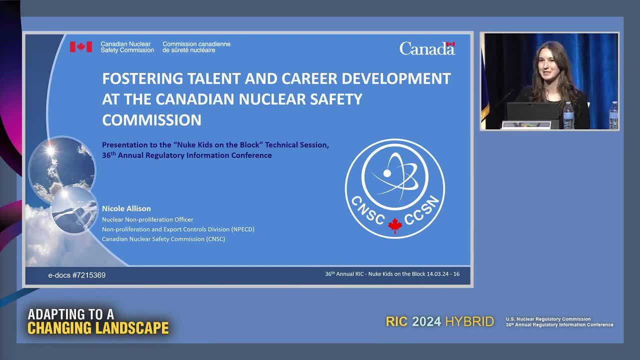 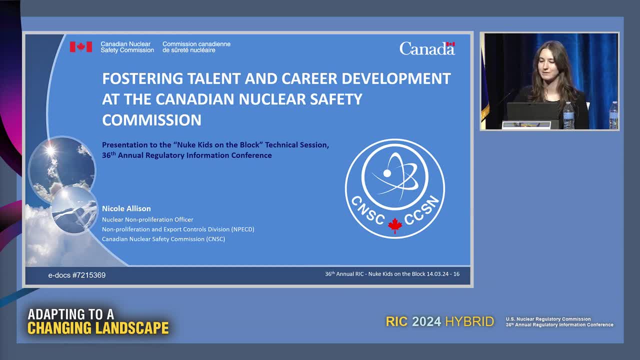 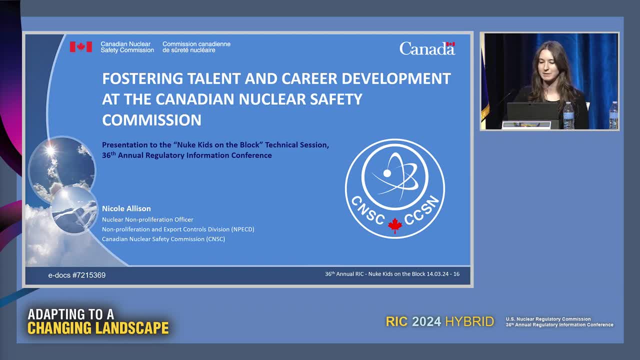 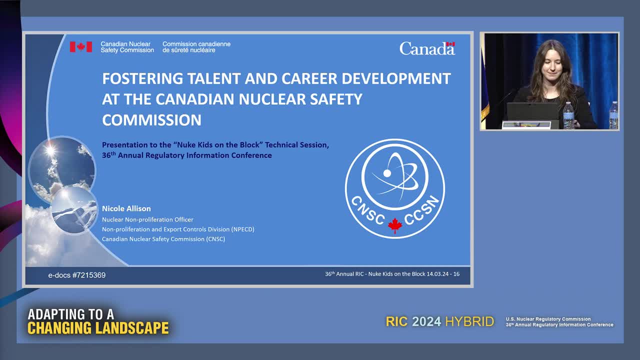 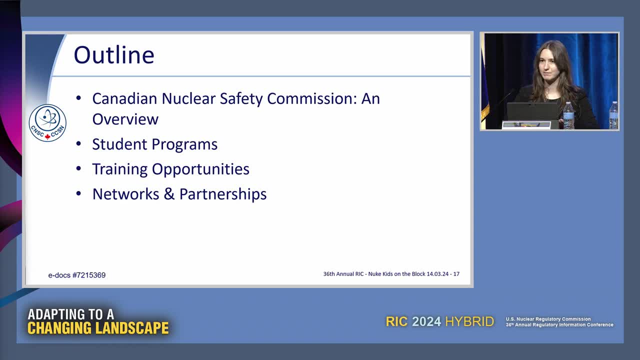 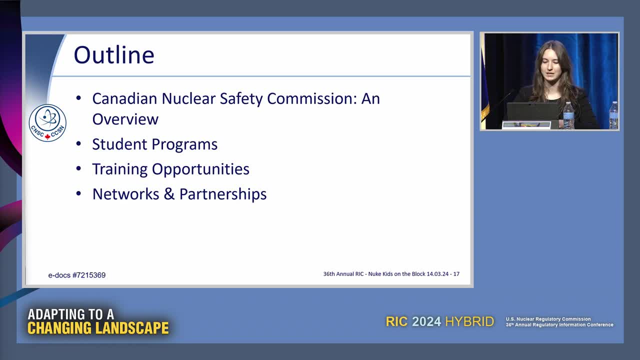 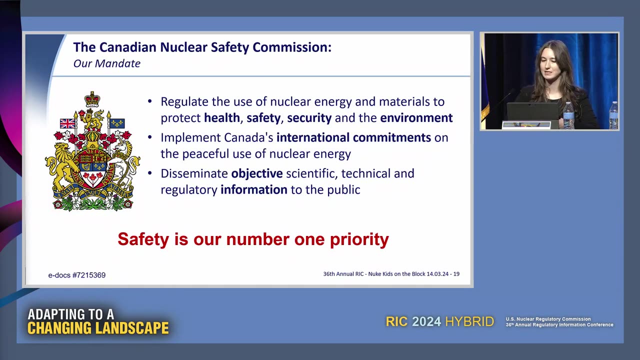 Engineering: Souratos Tontadiravit, Director, National Stakeholder for Nuclear Safety and Nuclear Engineering. harsha jitorad prophet 것. First here, I'll start with just very brief overview. The Canadian Nuclear Safety Commission, or CNSE, as many of you likely know, is the federal agency responsible for regulating. 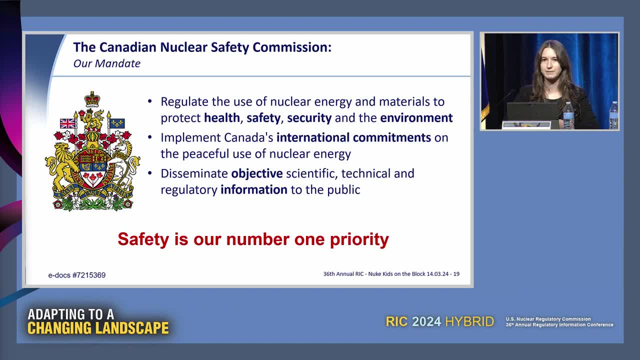 the use of nuclear energy and materials throughout Canada. Our mandate is three-fold: First, to protect health, safety, security and security, control security and the environment by regulating the use of nuclear energy materials. Second, to implement Canada's international commitments on the peaceful uses of nuclear. 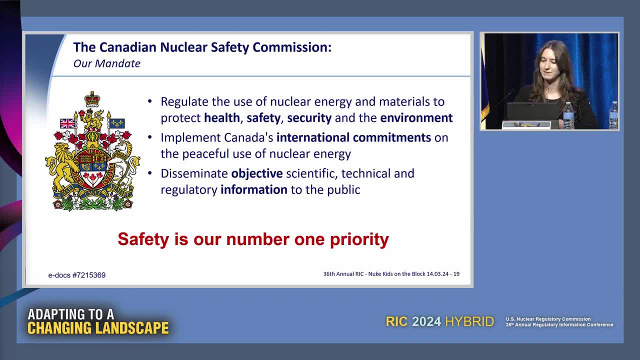 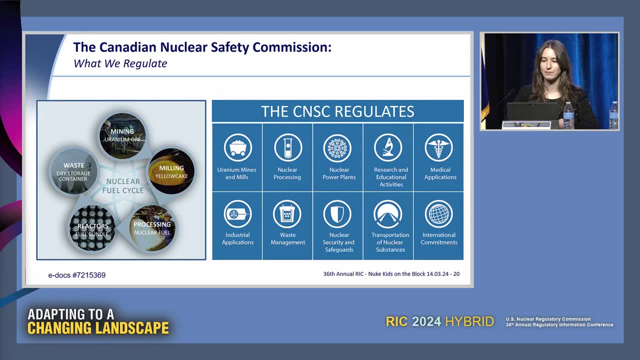 energy And, lastly, to disseminate objective scientific, technical and regulatory information to the public. In terms of the scope of our regulatory program, we're responsible for overseeing all nuclear activities in Canada throughout all stages of the nuclear fuel cycle. 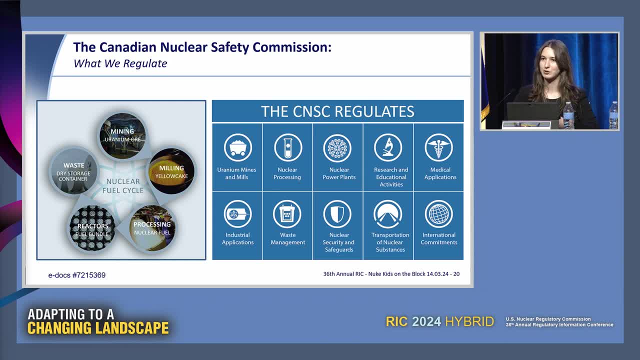 And in terms of my current role, as Miranda mentioned, I'm focused on import and export controls, but in my time as a technical co-op student, I've also had the opportunity to work in a number of different areas of the organization, which I'll touch on more in. 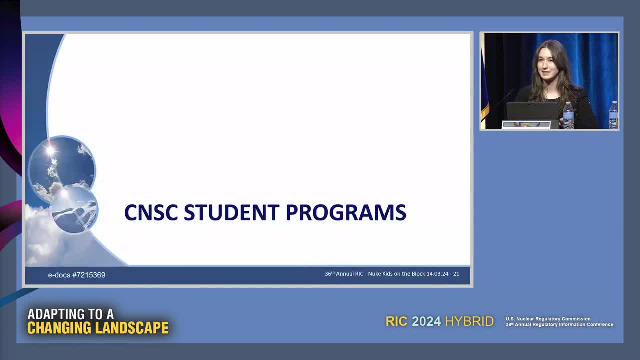 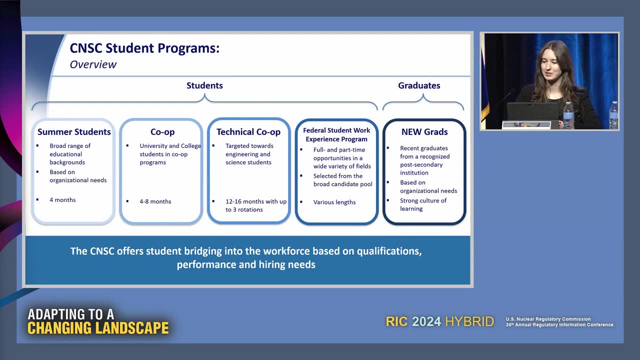 a couple slides. Next I'll take a few minutes to speak to some of our student programs at the CNSC. So starting at a high level first, we have five main categories of student opportunities. This includes four programs which are targeted more towards current college and university. 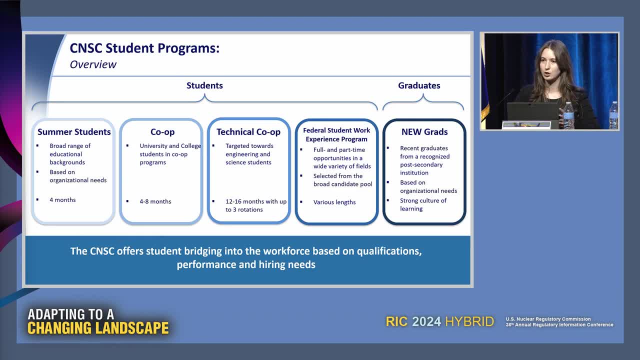 level students, which are our summer student program, our co-op and technical co-op program, and then also a federal student work experience program. But in addition to those four, we also have a new grad program which is targeted towards individuals who have recently graduated from a post-secondary institution. 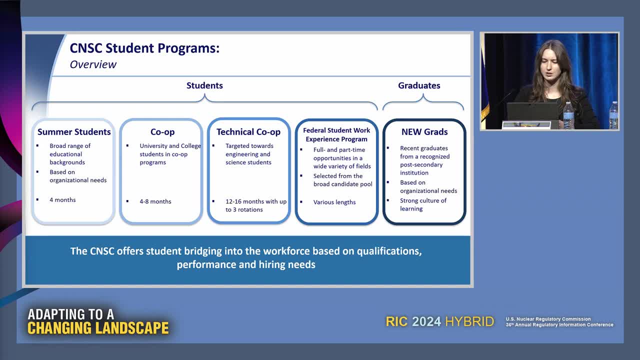 And overall, these programs cater to a variety of educational backgrounds. They draw from those different areas of education based on organizational needs, whether it's STEM or otherwise, And the duration of those programs can range from both short-term part-time opportunities, such as the summer student program, to longer-term work placements, such as the tactical co-op. 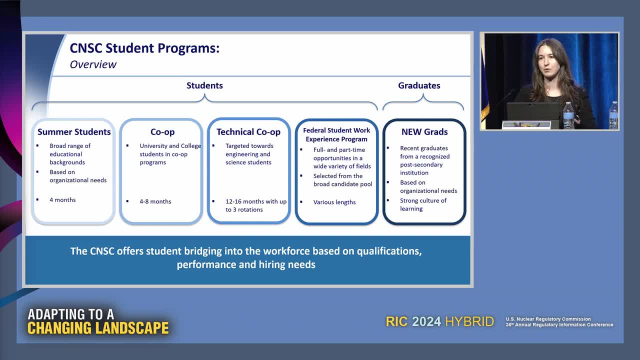 program. Personally, I joined the CNSC in 2010.. I joined the CNSC through the technical co-op program, which again I'm going to speak to in a moment. But I think one of the great strengths of having a variety of programs such as this: 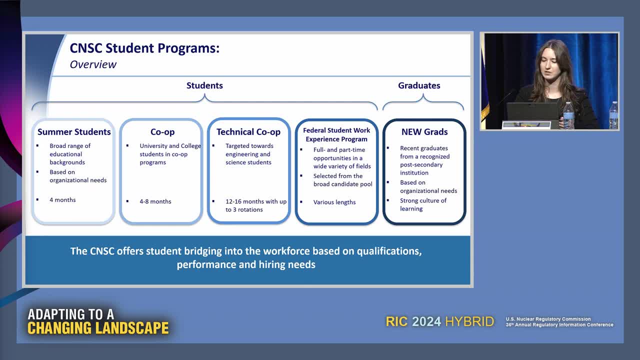 is that these student placements are made so much more accessible to a greater diversity of candidates and audiences. This, of course, has the benefit to those students, as they have greater career development opportunities for both post-secondary and new grad students, But it's also greatly beneficial to the CNSC as an organization, as it helps us to supplement. 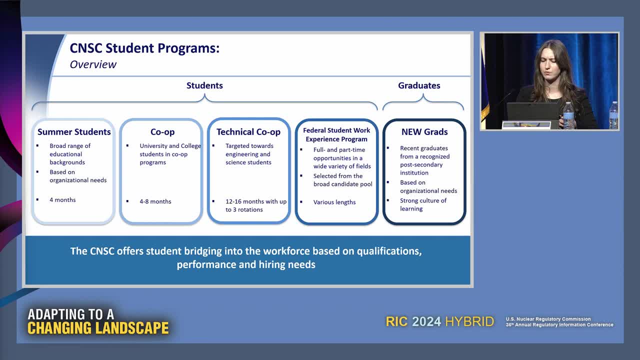 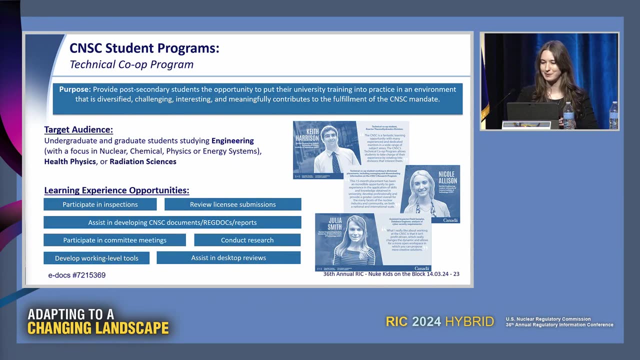 different areas of our workforce, And it also plays a really important role in investing in the education and the careers of those young regulators and public servants who may then be returning to us, as I did, through the student programs. So, as I mentioned, the technical co-op program is near and dear to my heart, as it's how 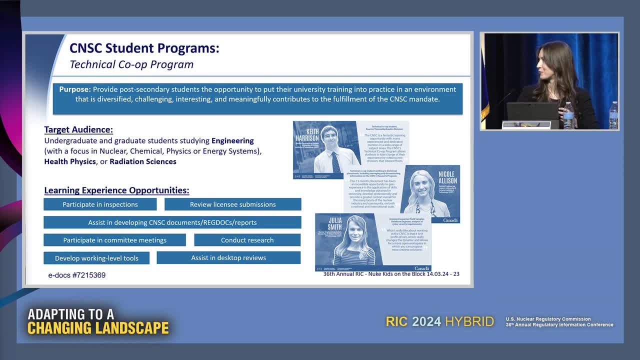 I first joined the CNSC And I like to see that there's this theme of those student programs being so special and crucial in the path that our career takes. The program here, the technical co-op program, is targeted more towards university students studying engineering. 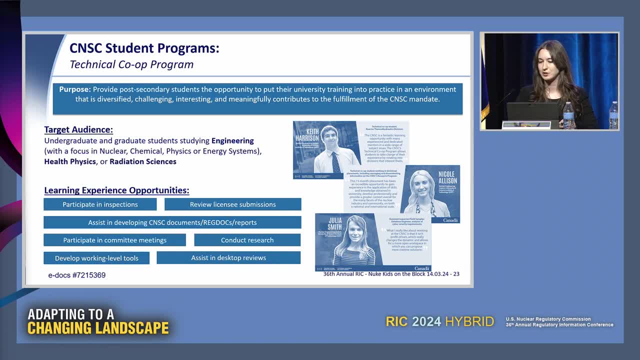 It's also one of the longer-term placements, so it takes place over 12 to 16 months, And during that time, students can rotate through three to four different divisions within the CNSC. While I was a student in this program, I had the chance to work with teams in the area. 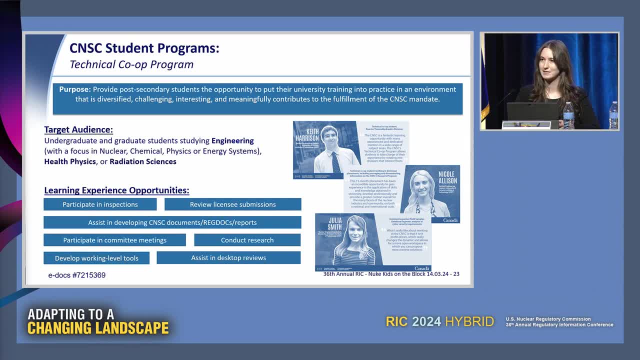 of regulatory research and evaluation, international safeguards, licensing of new major facilities, as well as probabilistic safety assessment reliability. So I got a good flavor of a lot of the work across the organization. It gave me the chance to get involved in activities. 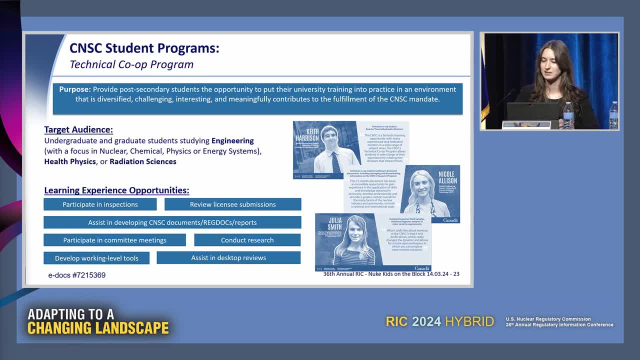 From reviewing regulatory documents to research submissions supporting Canadian safeguards and nuclear material accountancy, to authoring a research paper on the regulatory basis for exclusion zone sizing in Canada, And on that research paper the CNSC also supported and funded my travel to present. 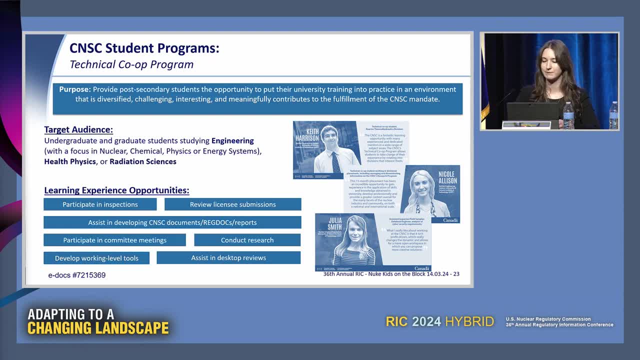 that work at a Canadian Nuclear Association student conference, which was one of my very first opportunities to present research work I had conducted in a conference setting such as that. What I personally found to be really excellent about this program is the fact that it's a 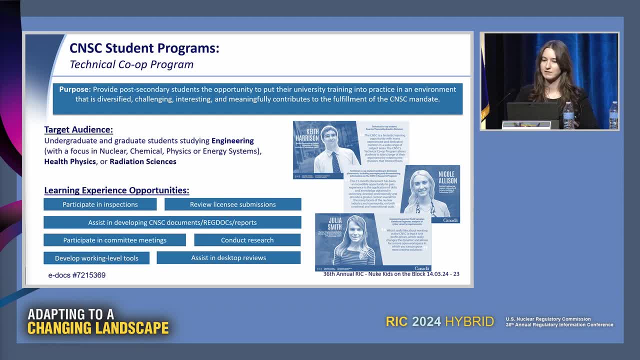 very diverse group of people And I think that's what I really like about this program is that those placements within different teams give first enough time to learn about the work those groups conduct, but also enough time to get meaningfully engaged in those core day-to-day work activities. and 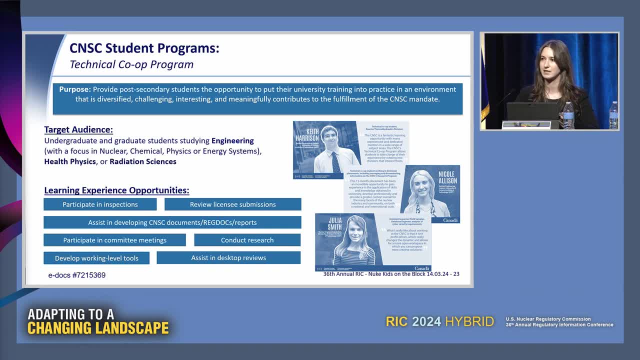 understand for yourself what it's going to be like working in a professional setting such as that. But at the same time, I found that rotating through the different divisions within the CNSC also gave me a much bigger picture. look at how the different areas of the organization 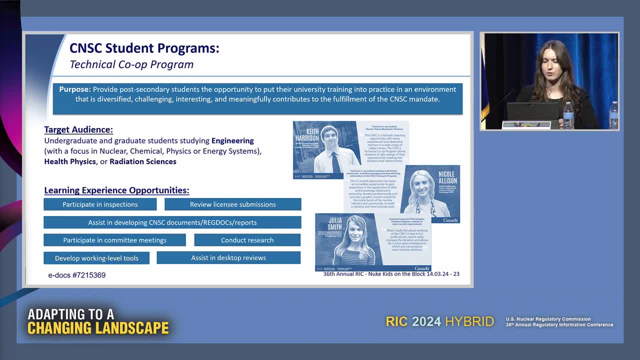 work together, what type of work they perform and, even more broadly, what type of work is encompassed by the nuclear industry at large. I think it's such a great experience. Thank you, I think it's such a great experience to have, especially as a student that's soon to be. 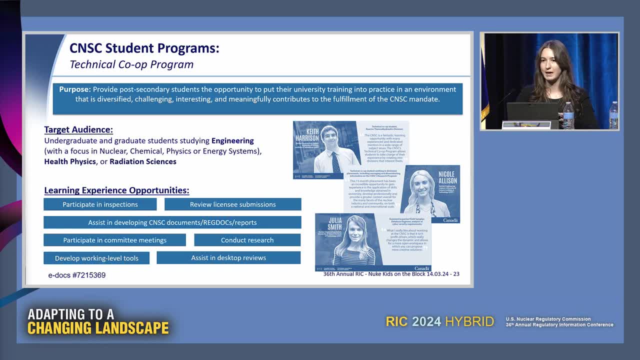 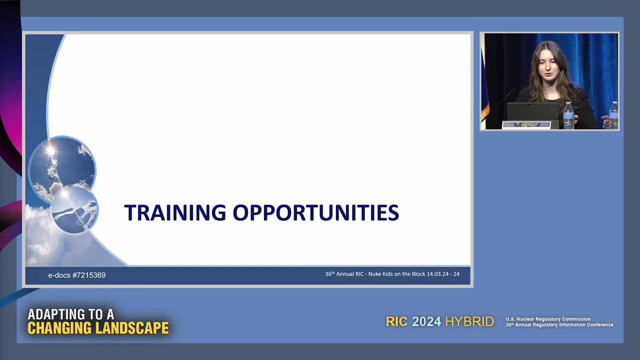 leaving university, because it helped open my eyes to how many different paths and options there were for my career to progress, And it also gave me some firsthand experience as to what it was going to be like working in those different environments. All right, Next I'll speak on some of the training opportunities and programs that we have at the CNSC. 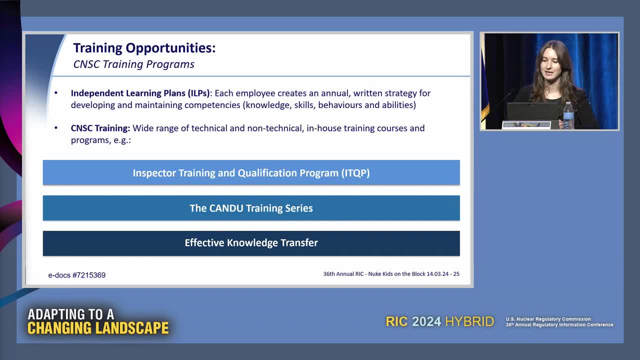 One of the things I really appreciate about the CNSC as an organization is that continuous learning is identified as one of the most important things that we do. This is one of the key areas of our organizational culture, which is needed to ensure that the CNSC is building a competent and flexible workforce. 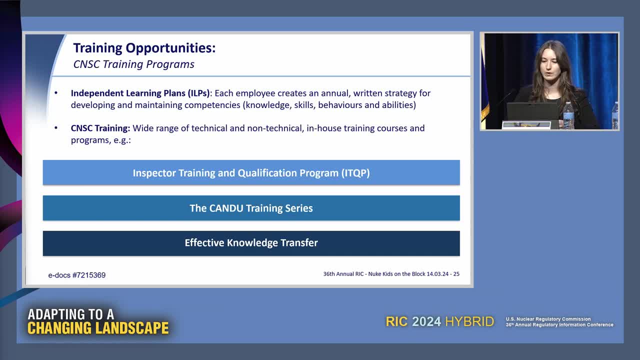 One of the ways this culture of learning is supported is through an independent learning plan program, and this is a program whereby all CNSC employees create personalized written training plans for how they aim to develop and maintain their technical knowledge and behavioral competencies. These learning plans are updated on an annual basis and they're also endorsed by two levels. 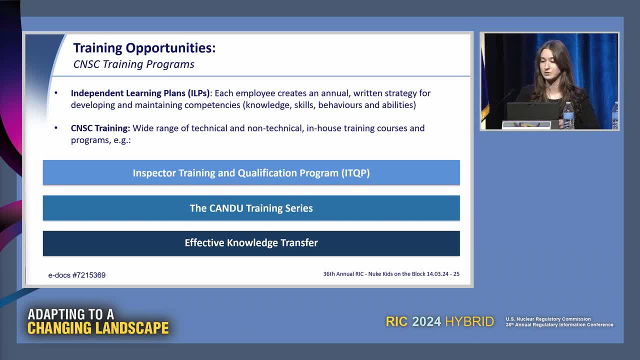 of management to ensure that employees are supported in reaching their career goals and learning objectives. Thank you. The training plans themselves are used both to support building competencies related to your current area of work, but they can also be used to identify areas of training you're. 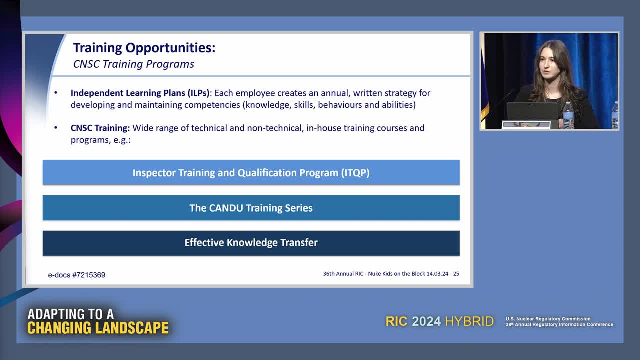 interested in to progress your long-term career development goals in other areas as well. In terms of actual training, there's also a wide variety of programs and courses that are delivered internally to the CNSC, Just to highlight a few notable ones here that I've had the opportunity to experience. 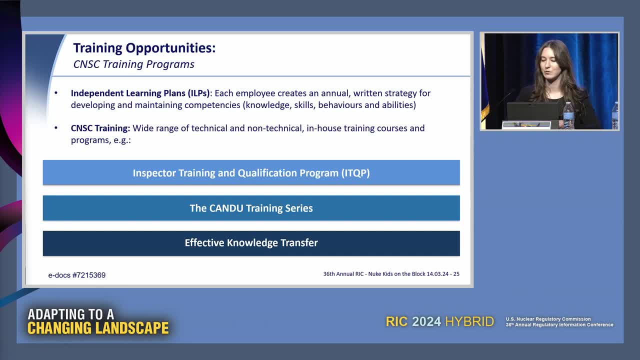 myself. First, I have the CNSC Inspector Training Qualification Program, which is a combination of both general and service line-specific in-class Combined with an on-the-job training period that's supported by a mentor designated to each inspector in training. Another program I'd highlight is the Can Do Training Series, which is a technical course. 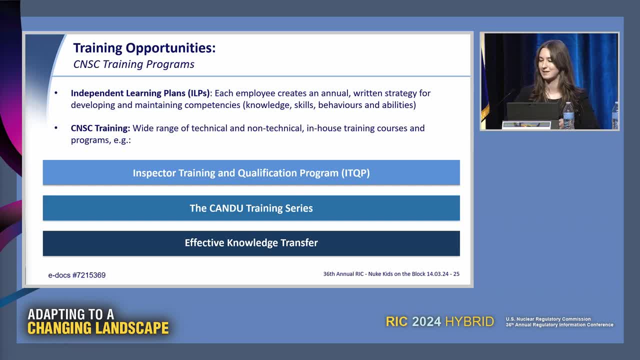 we have on the systems, structures and principles of can-do reactor design. One really great aspect to this series is that it's offered at different levels of complexity: technical complexity, which helps to make it more accessible to all staff who are interested in developing their technical knowledge in that area, regardless of what their educational 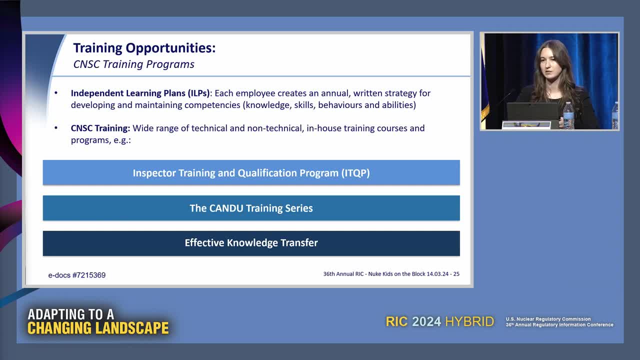 background might be, Whether they came to us from STEM or political science or otherwise. One last course I'll mention here is the Effective Knowledge Transfer in-class training course that we have, which discusses strategies and practices for sharing both tacit and explicit. 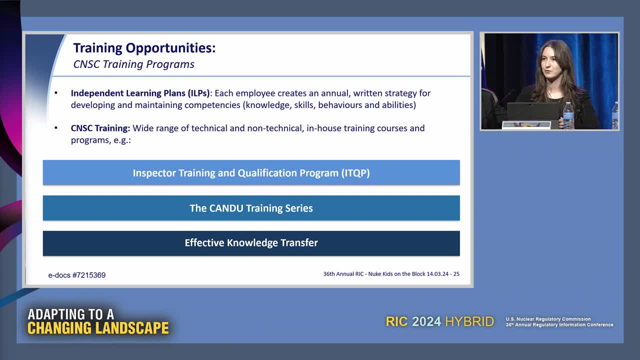 knowledge in various settings. I had the opportunity to take this course recently and I found it to be really beneficial, both from the perspective of someone who has now recently begun training new staff who are joining onto our team- to understand how I can do a better job of sharing my knowledge. 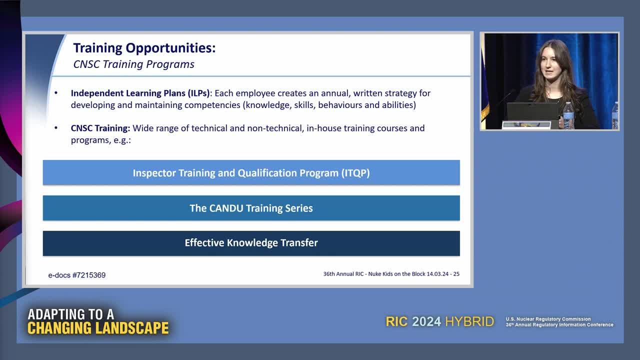 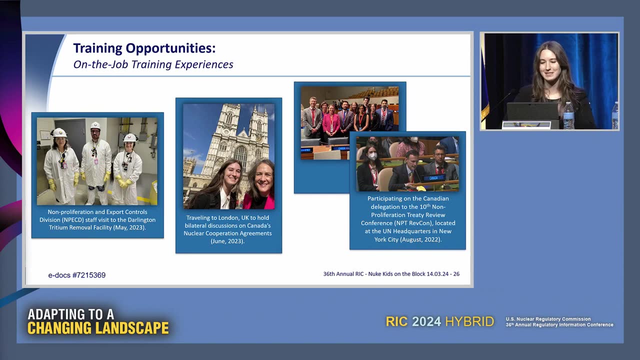 with them. I think it's really important to take the time and reflect for myself on the ways that I learned and how I can be mindful in how I receive knowledge from more experienced staff in a way that's effective for me. Continuing here on that same theme of knowledge transfer and on-the-job experiences, I think 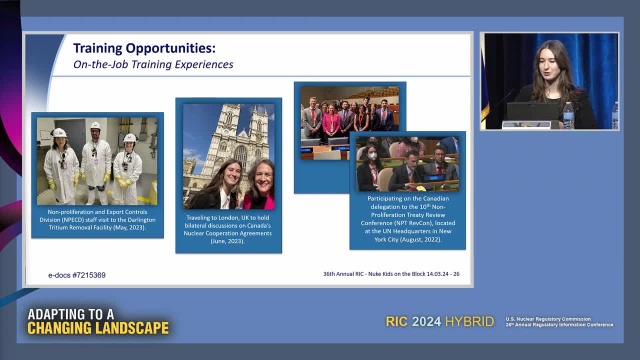 some of the most valuable training and knowledge transfer experiences I've had in my career so far have been those instances where I've been working alongside and learning directly from more experienced colleagues from the CNSC or even other government departments or other areas of the public service. 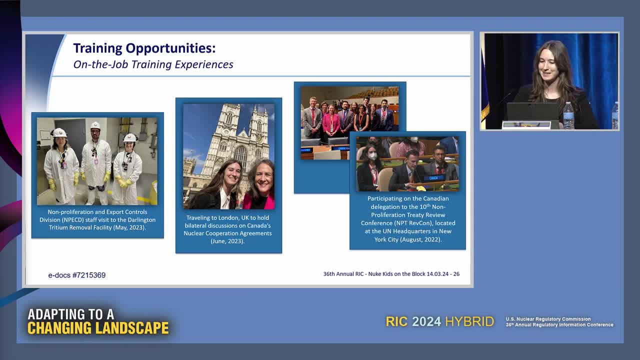 Just to share a few of my experiences here, because pictures are fun. On the left, myself and two co-workers took an on-site visit to the tritium removal facility at the Darlington Nuclear Generating Station, where we had the opportunity to learn about. 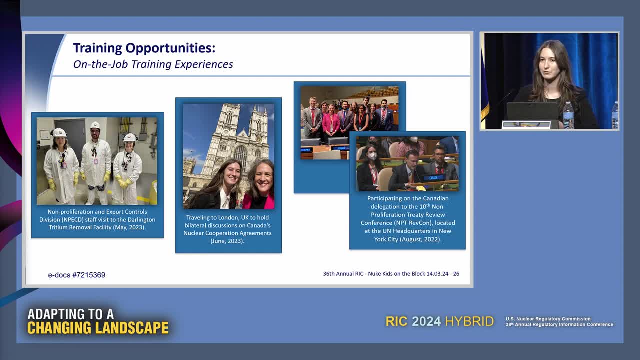 some of the nuclear-related equipment we license as part of our CNSC important export licensing program. The center picture is myself and my director traveling to London, England, to hold bilateral discussions with some of our regulatory counterparts. They did not take place at Westminster Abbey, but we had a very nice time visiting it as. 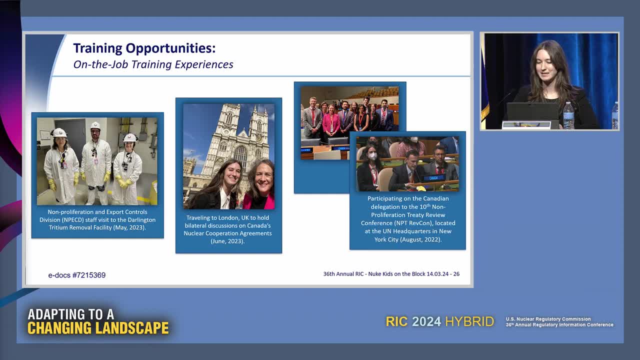 well, And then in the right-most picture is myself, as part of the Canadian delegation to the Non-Proliferation Treaty Review Conference, which took place at the UN headquarters in New York, where I had the opportunity to learn how someone like myself, with a more technical 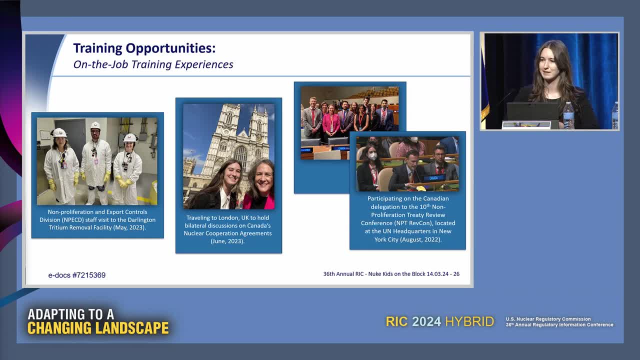 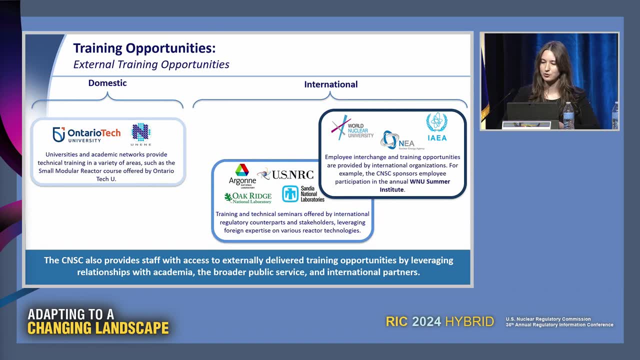 background can support colleagues who are working in more of a diplomatic setting. One last side, on trading. I also wanted to highlight that there's such a wide variety of external trading opportunities that can be leveraged both domestically and internationally. On the domestic front in Canada, 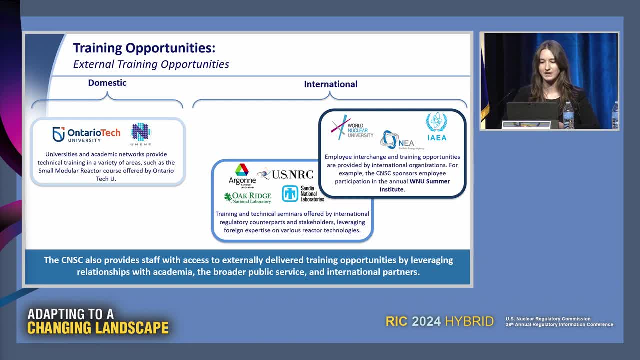 The CNSC leverages relationships with academia to provide staff with technical training opportunities. One example that I've taken is a technical training course on SMR technologies that's offered by the University of Ontario Institute of Technology, which is also where I studied for my bachelor's of engineering. 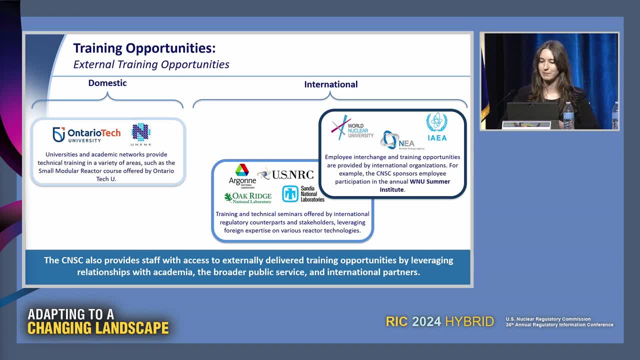 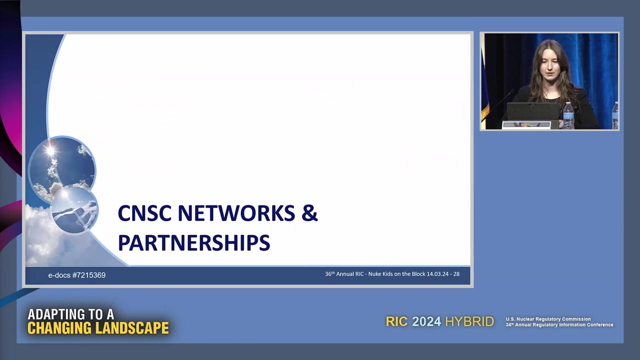 And then looking internationally, technical training offered by regulatory counterparts, international organizations, are also ways that the CNSC leverages those different sources of technical experience and expertise through sponsoring employee participation in those courses or even interchange opportunities at some of those agencies. All right, finally, here I want to touch on a couple of networks and partnerships that 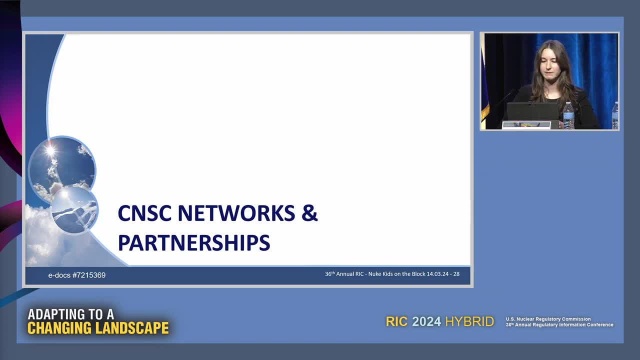 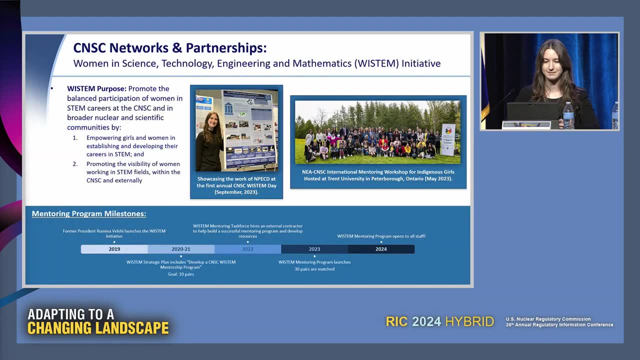 the CNSC leads or engages with, and there are a variety of employee networks and partnerships that the CNSC has. but these are just a couple of examples I've chosen to highlight here that are meaningful for me. So the first example I have here is the CNSC: women in science, technology, engineering. 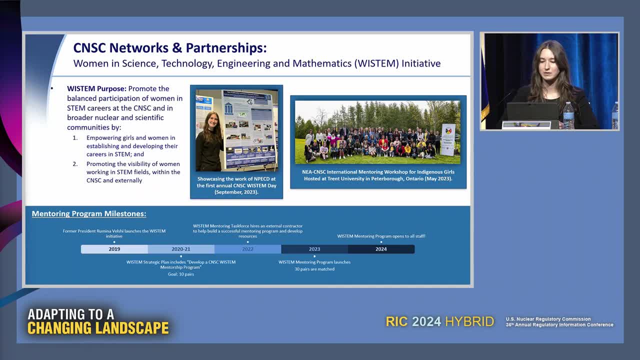 and mathematics, or WISSTEM initiative. This one is a relatively new initiative, which was launched in 2019 under our previous president, Ms Romina Velshi. Overall, the purpose of this WISSTEM initiative is to promote greater diversity, innovation. 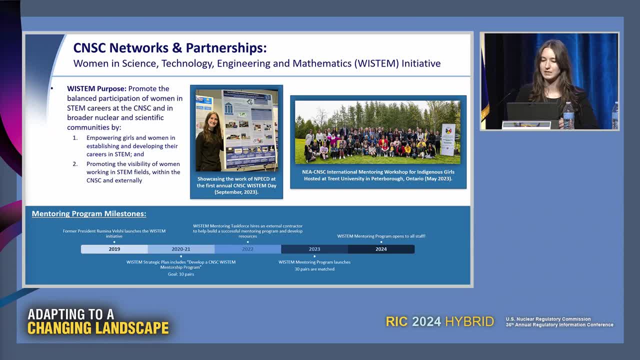 and equity in the STEM workforce by contributing to the empowerment, development and visibility of women in STEM careers. A couple of pictures I have on the slide here just to highlight some recent activities. On the left is a picture of myself at the CNSC's first annual WISSTEM day in September of last. 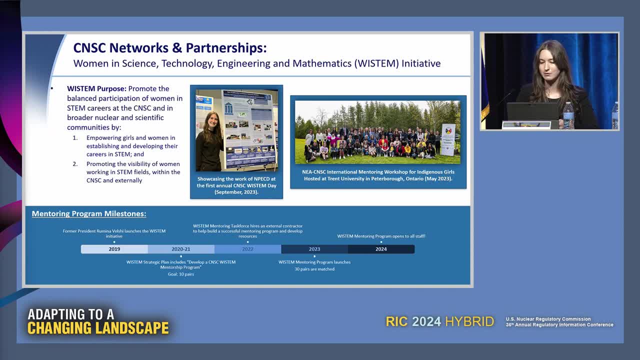 year where I had the opportunity to present on my work and the work that others conduct as well in the non-proliferation and export controls division, and it was also an opportunity for me to connect with and share with other women working in STEM fields across the organization. 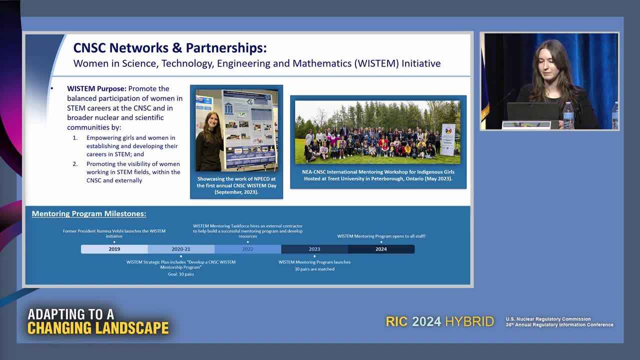 as well as external to the CNSC. And then on the right I have a picture from the International Mentoring Workshop for Indigenous Girls, which was an event jointly hosted by the Nuclear Energy Agency and the CNSC in May of last year. It was an event that the WISSTEM team at the CNSC helped organize and it brought together. 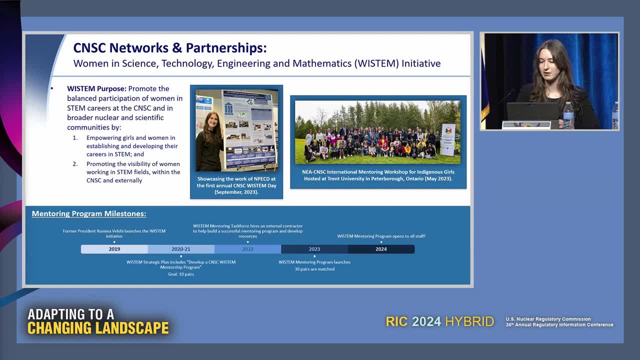 women in STEM fields from around the globe to help mentor and inspire young Indigenous girls to explore career opportunities and the application of knowledge in STEM fields. Then one last point I'll highlight here, which I find very exciting, is the very recent launch of the WISSTEM mentoring program, which is now aimed at connecting women within the organization. 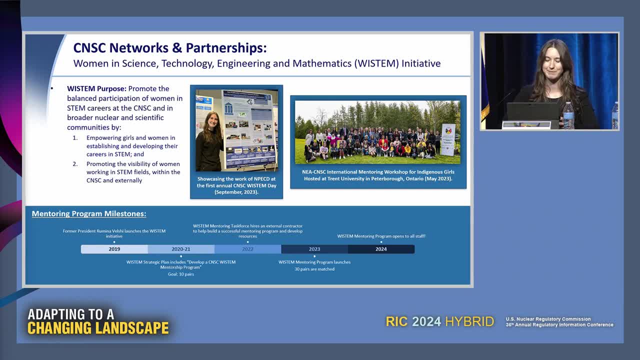 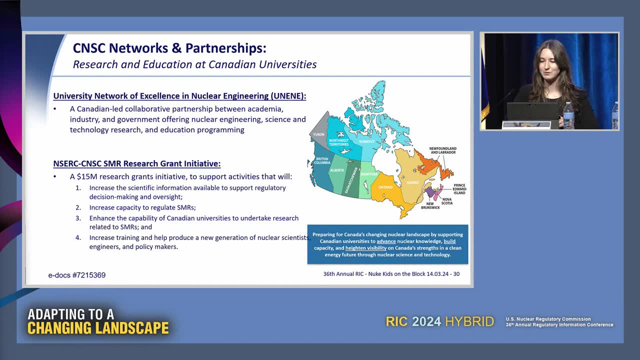 to set up mentor and mentee relationships for them. Finally, I want to highlight some of the work the CNSC is doing to support research and education. The CNSC is working with Canadian universities through networks and partnerships. One example I have here is through the University Network of Excellence in Nuclear Engineering. 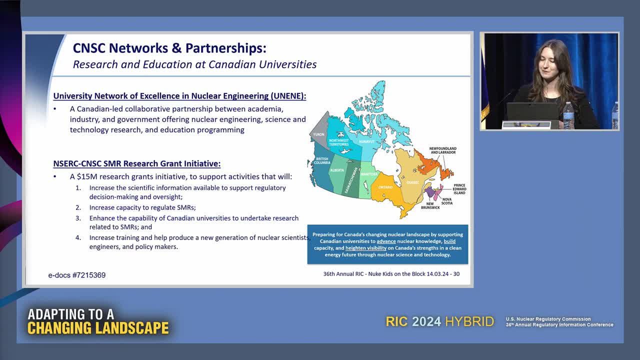 or UNINI, which is a network of Canadian and international universities, industry and federal government working together to develop and support the next generation of highly qualified professionals in the nuclear field. Within this partnership, the CNSC provides support in a number of ways in terms of participating. 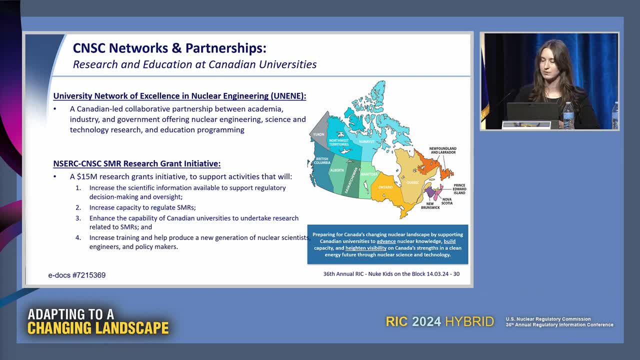 on various committees, giving input on strategic direction, as well as providing funding and grants. And then, in terms of grants, the CNSC has also recently partnered with the Natural Sciences and Engineering Research Council of Canada to launch an SMR Research Grants Initiative. 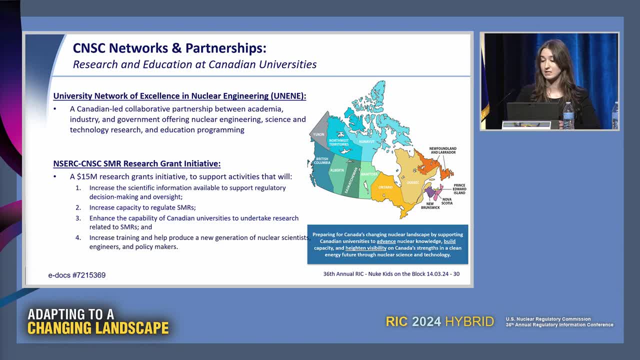 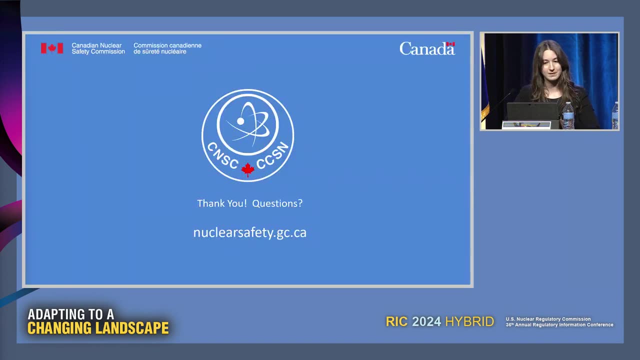 which will fund academic research related to SMRs. The current phase of this initiative taking place right now has currently contributed $9.4 million towards 29 research projects taking place over the next three years, and a second call for proposals is expected to be launched in the next coming fiscal year. 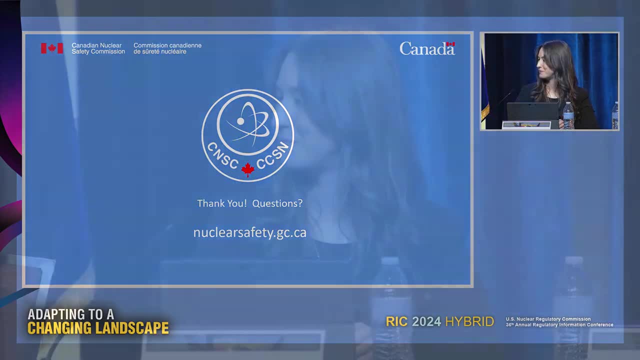 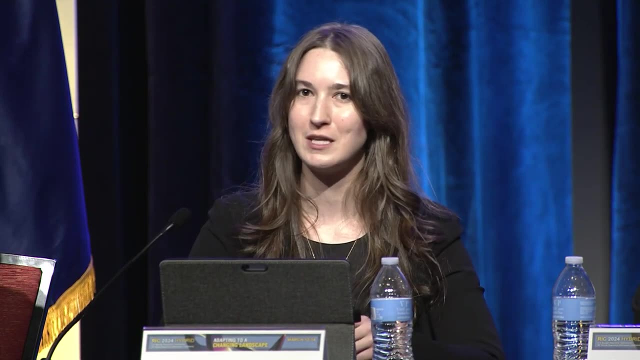 So just to wrap up here, I want to say thank you again to the NRC colleagues For the opportunity to come speak here on this panel. I'm very much looking forward to hearing from my other panelists. I hope this gave you some interesting insights into the various ways that the CNSC is reaching. 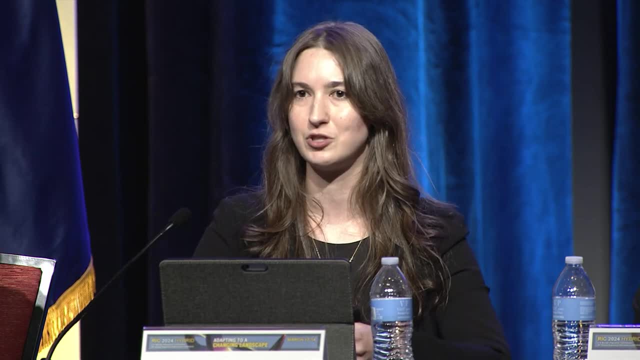 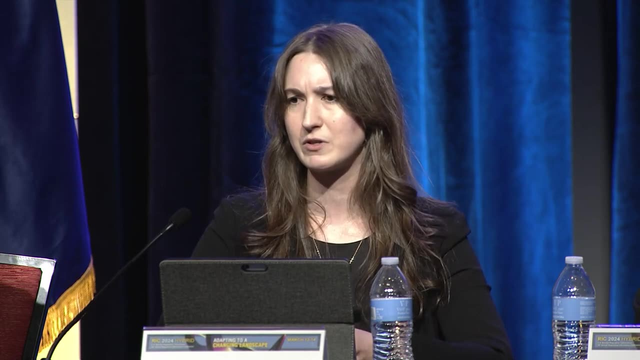 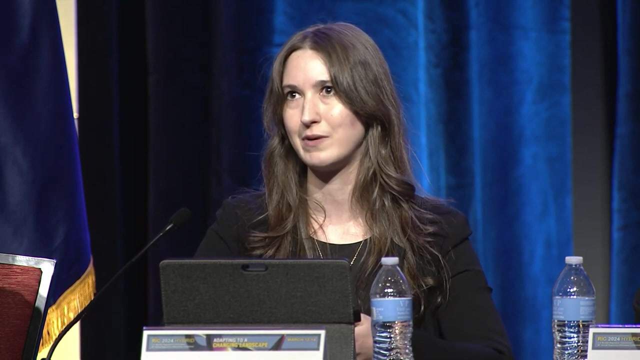 out to students, whether they're in post-secondary institutions, universities and colleges, or younger girls, for example, through workshops hosted by the CNSC, as well as some of the training opportunities and knowledge transfer practices that are incorporated for those young professionals who are now entering their or beginning their career. 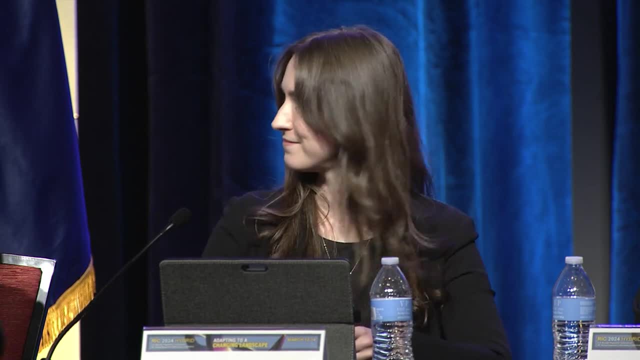 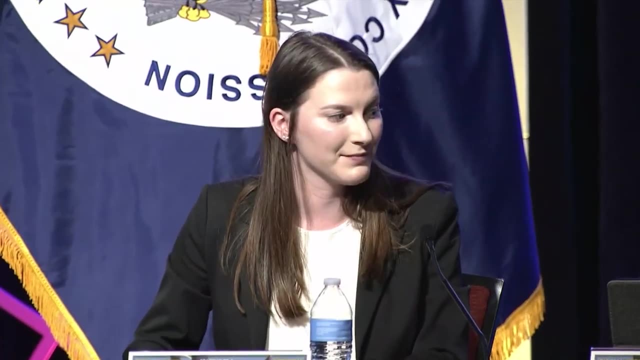 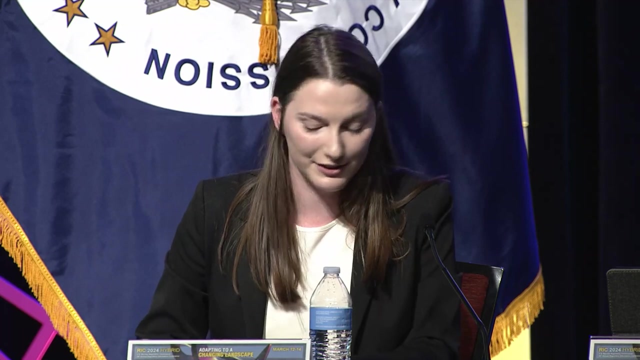 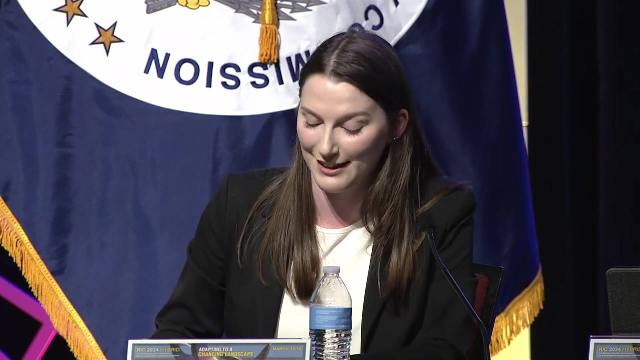 Thank you. I hope our next presenter is Alexandra. Alexandra chose a career in the nuclear field primarily because when she was little, she often heard family discussions about nuclear power in the field. Her curiosity led her to think about what it would be like to work in this field. 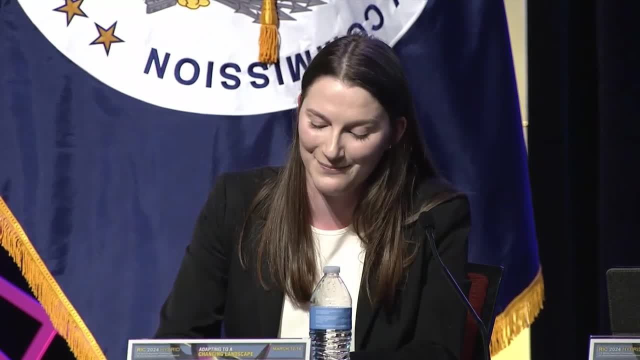 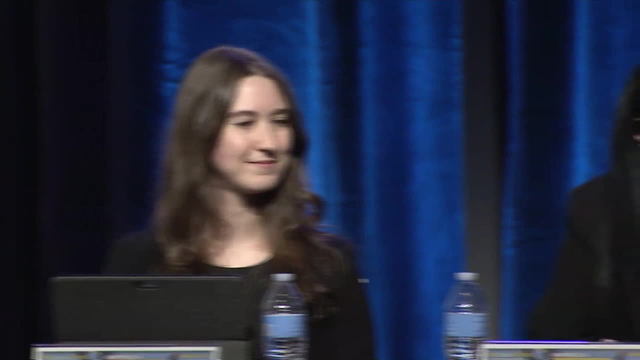 She also wanted to be a part of a dynamic and ever-changing society, an ever-changing industry that promotes the use of clean and sustainable energy sources, And I will now hand it over to Alexandra to present. Thank you so much, Hello everyone. 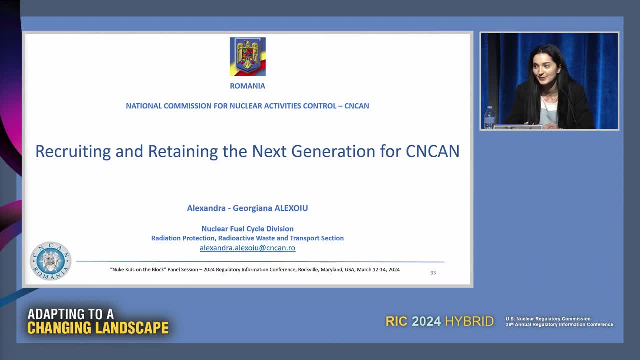 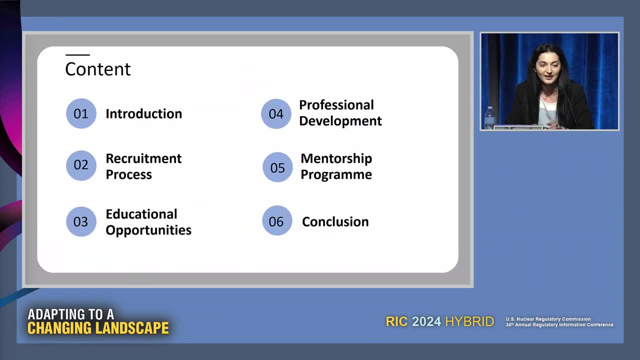 I'm very grateful to be part of this panel session, So my presentation today will be about the process of recruiting and retaining the next generation for Cheney Khan. So this is my outline. I will speak a little bit in the introduction about general things about Cheney Khan, just. 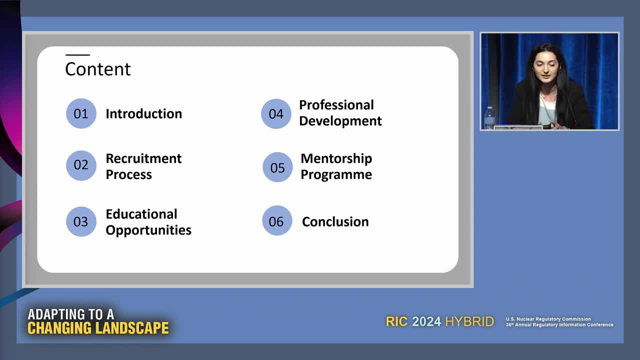 to give you an overview about our mission and the need to maintain and attract the new generation within the institution. Then I will go over to the recruitment process within the institution, educational opportunities, professional development, mentorship program and some conclusion, Okay. 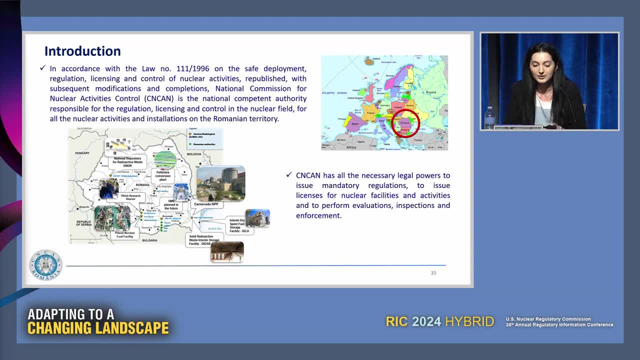 So, in accordance with our nuclear law, Cheney Khan is the national competent authority responsible for the regulation, licensing and control in the nuclear field for all the nuclear activities and installation on the Romanian territory. I put it here: our nuclear country profile. 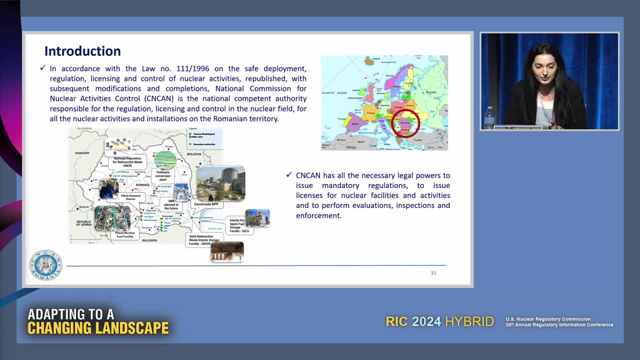 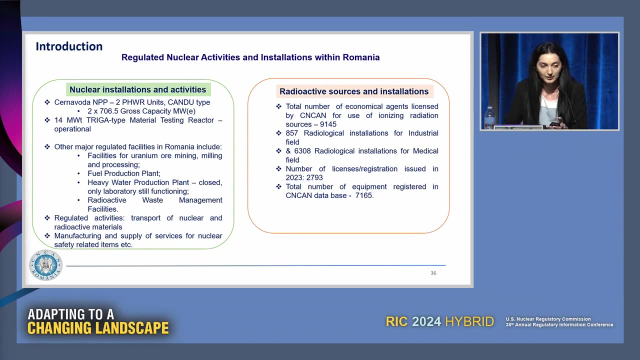 So, as you can see, we have many nuclear and radiological facilities, So we need to attract and keep the next generation of young talent within the institution. As you can see on the map before we have a nuclear power plant with two units in operation. 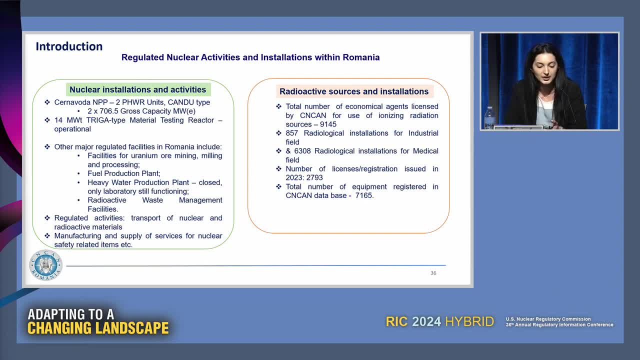 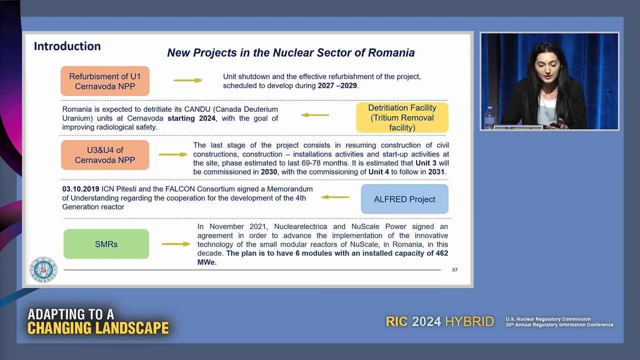 Also, we have a research reactor and other major facilities, like facilities for uranium ore mining, milling and processing, fuel production plant, radioactive waste management facilities and so on. I put it here, on this slide, our future project, Not especially for the technical part of them. 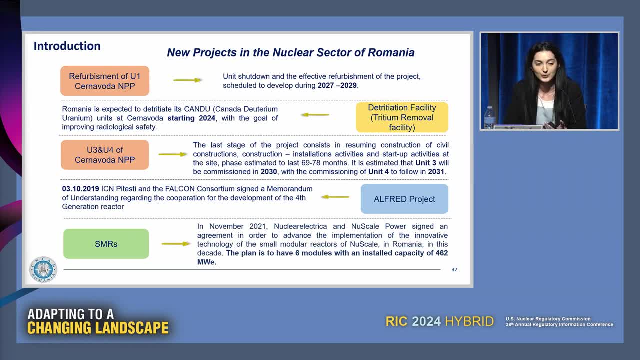 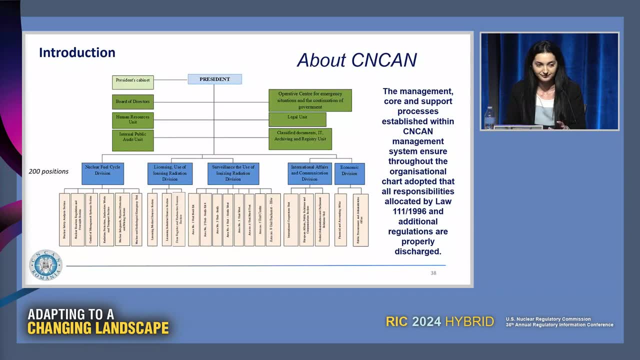 Just to highlight the need and the fact that it is very important to us to recruit and maintain the next generation for both current and future projects. This is our organizational chart. I will go quickly through them. So we have five divisions. Three of them are technical divisions. 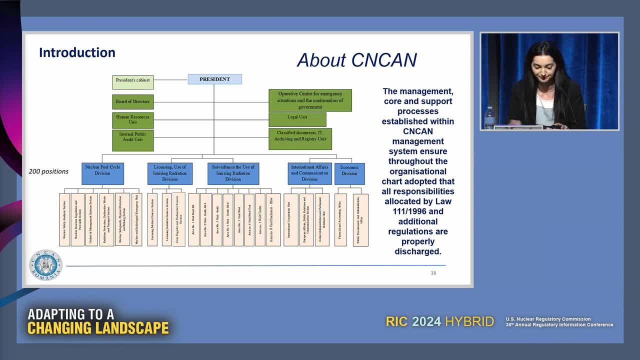 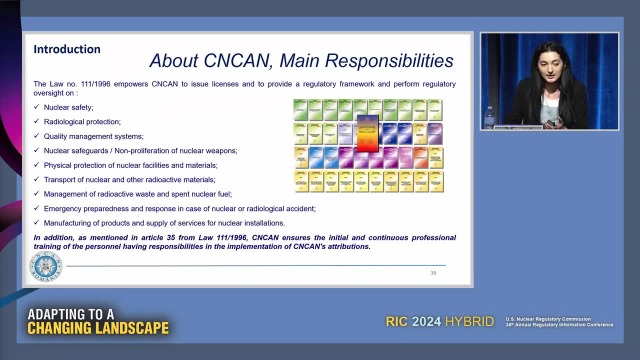 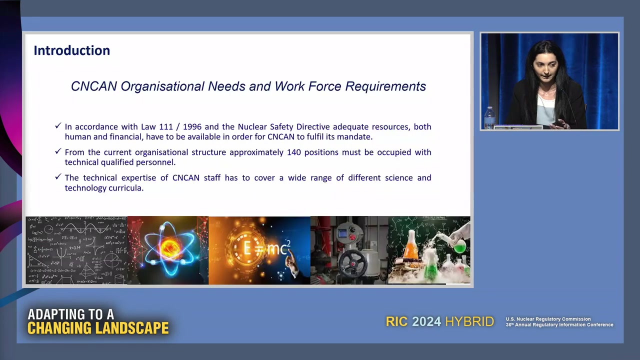 I'm working under the nuclear fuel cycle division And the last slide about CENECAN. So our main responsibilities is issuing licensing, provide the regulatory framework and perform regulatory oversight on nuclear safety, radiological protection, quality management system and so on. 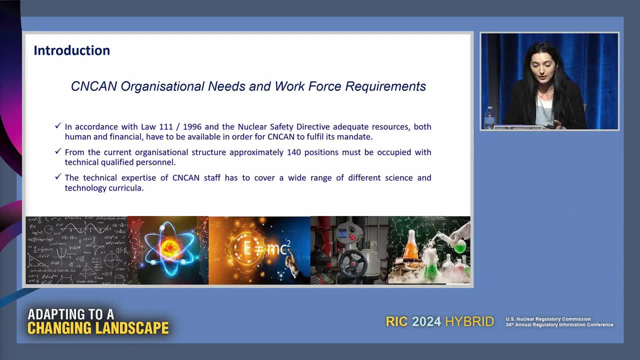 Regarding our organizational needs and workforce requirements in accordance with our nuclear law. Under the nuclear safety directive, adequate resources, both human and financial, have to be available in order for CENECAN to fulfill its mandate. From the current organizational structure, approximately 140 positions must be occupied. 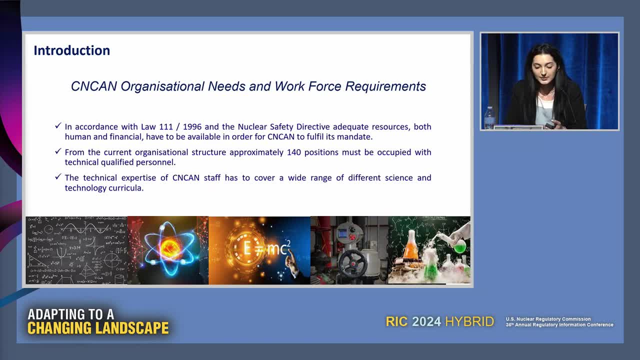 with technical qualified personnel. The technical expertise of CENECAN staff has to cover a wide range of different science and technology curricula. So I will give you some examples in the following slides: Slide 5.. Slide 6. Slide 7.. 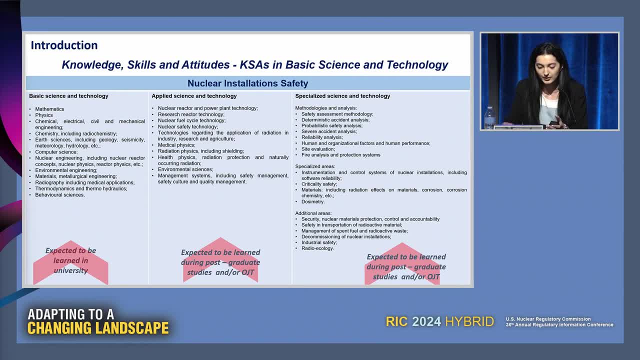 Slide 8.. Slide 9.. the slide presents an overview of knowledge, skills and attitude, For example for nuclear installation safety. So we expect young graduates to have the basic science and technology knowledge from the university and, regarding the applied science and specialized science and technology, to 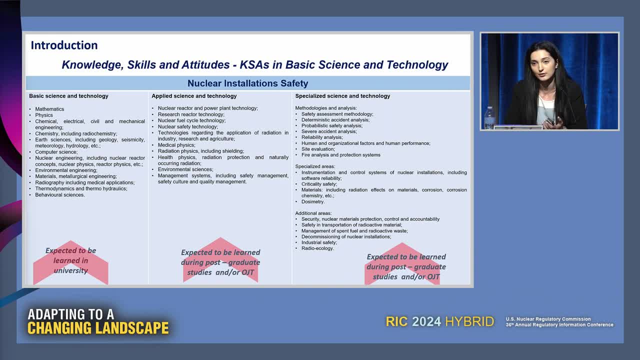 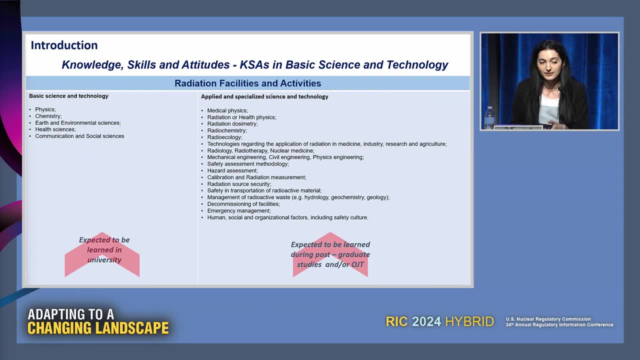 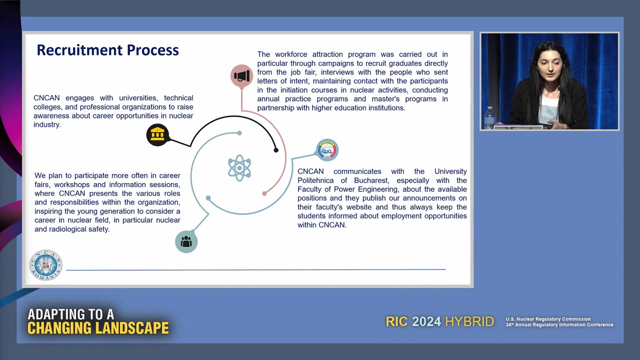 be learned during post graduate studies and or on-job training, Slide 10.. This is the same approach example for the radiation facilities and activities we have. we expect some basic science and technology knowledge and the other one to be learned during postgraduate and on job study training. so now I will speak about the 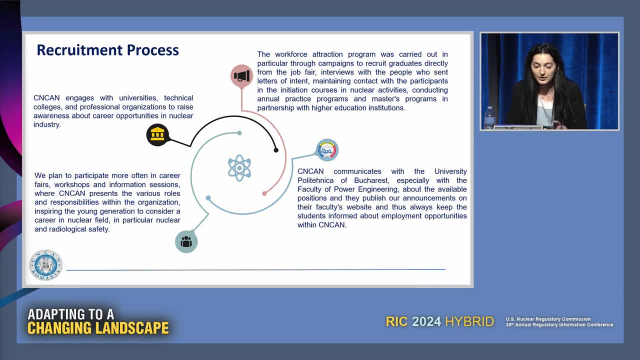 requirement process. so the work-based attraction program was carried out in particular through campaign to recruit graduates directly from the job, fair interviews with people who send letter of intent to us, maintaining contact with the participant in the initiation courses in nuclear activities. and conducting annual practice program and master's program in partnership with 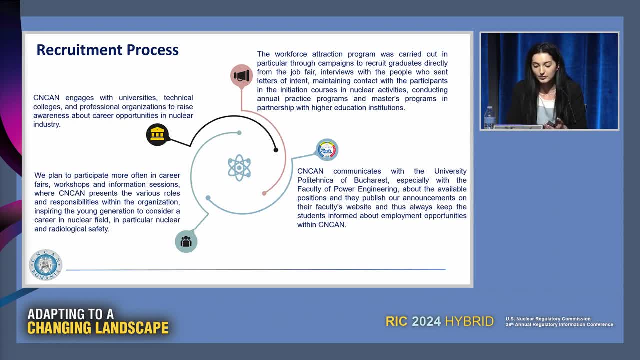 higher education institution. we communicate with the University Polytechnica in Bucharest, which is a technical University, especially with the Faculty of Power Engineering, about the available position within the institution and they publish a our announcement on their faculties website and those always keep the students informed about employment opportunities within Chenecan. so as I 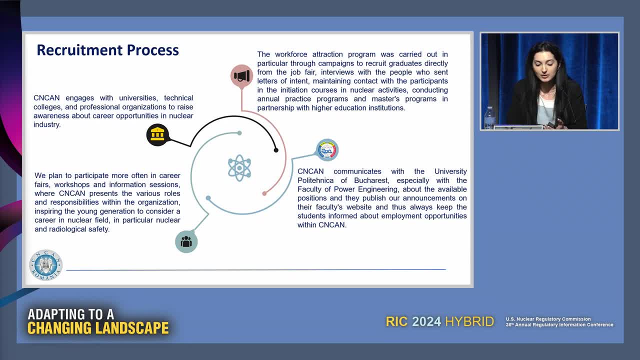 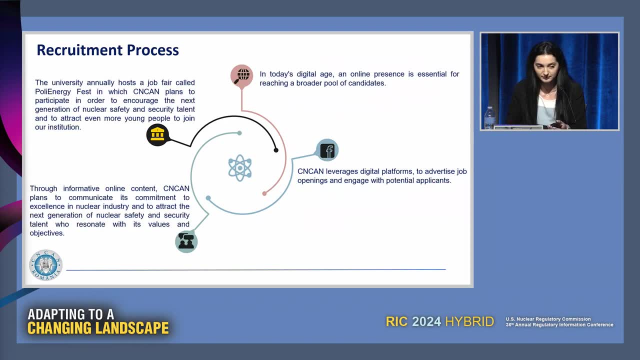 said Chenecan, engage with universities, technical colleagues and professional organization to raise awareness about career opportunities in nuclear industry. as we all know, in today digital age, an online present is essential for reaching a broader pool of candidate. So, if I can leave a read: digital platforms to advertise. 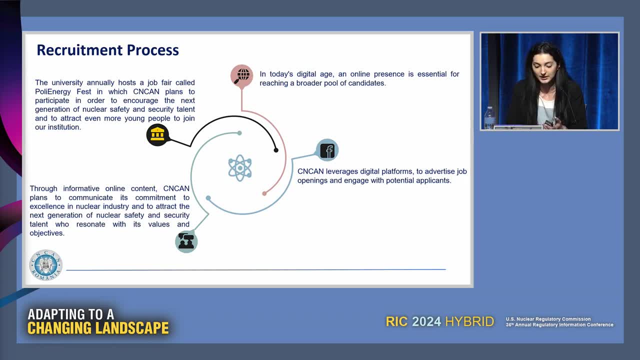 the opening engagements with potential applicants. also the University, I know we host a job fair called fully energy fest in the you can Ήan Pan to participate in order to encourage the next generation of nuclear safety and security talent enter truck even more young people to join our institution. regarding the anyways we are engaged on global. addressed the helped probably anting original. you know the commission has a number of members now. WAR NOW in the community at our institution and by academics. stands in our community in the veins, as well as clinical intelligence and advanced in two organizations inы. 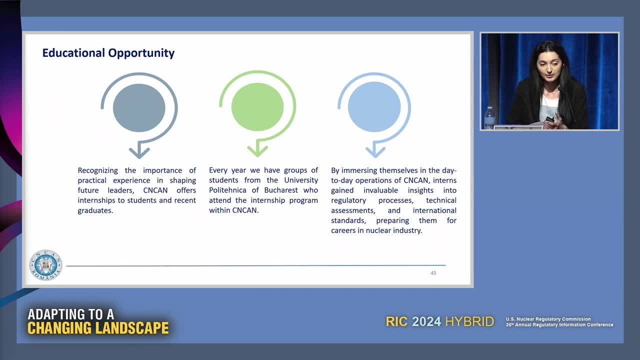 that are located here. all love to them. niin people are reaching out for numerous Regarding the educational opportunities. so recognizing the importance of practical experience in shaping future leaders. CENECAN offers internship to students and recent graduates. So every year we have groups of students from the University Politecnica of Bucharest who 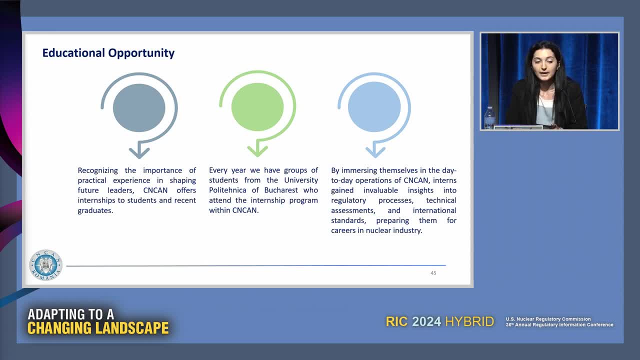 attend the internship program within CENECAN And, by immersing themselves in the day-to-day operation of CENECAN, interns gained invaluable insight into regulatory process, technical assessment and international standard, preparing them for careers in nuclear industry. 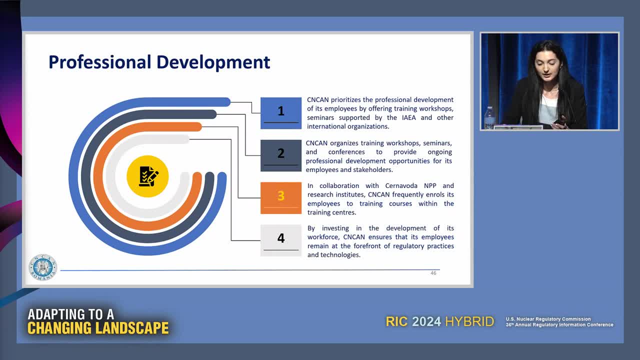 Regarding the professional development. so CENECAN prioritized the professional development of its employees by offering training workshops, seminars supported by IAEA and other international organizations also organized training workshops, seminars and conferences to provide ongoing professional development Opportunities for its employees and stakeholders. 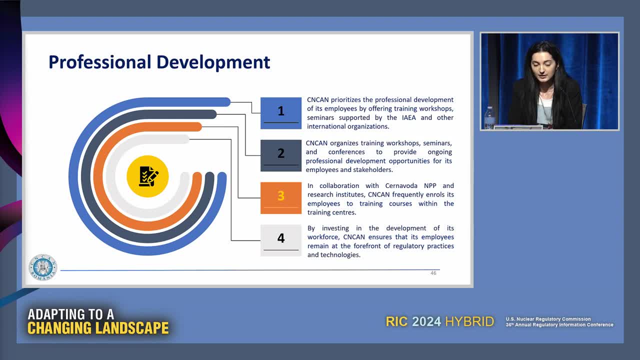 Also in collaboration with Cernavoda, NPP and the research institutes. CENECAN frequently enrolls its employees to training courses within the training center And by investing in the development of its workforce, CENECAN ensured that its employees remain at the forefront of regulatory practices and technologies. 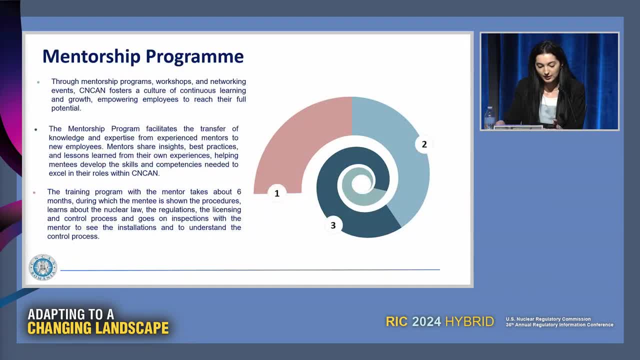 And so we have a lot of opportunities for CENECAN. And so we have a lot of opportunities for CENECAN. And some words about the mentorship program. So through mentorship program workshops and networking events, CENECAN foster a culture. 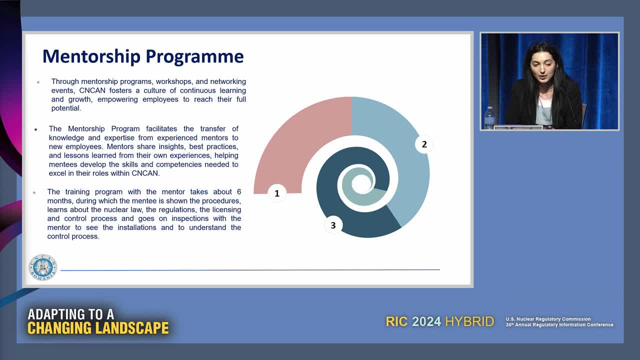 of continuous learning and growth, empowering employees to reach their full potential. The training program with the mentor takes about six months, during which the mentee shows the procedures, learns about our nuclear law, the regulations, the licensing and control process, and also goes on inspection with the mentor to see the installation and the 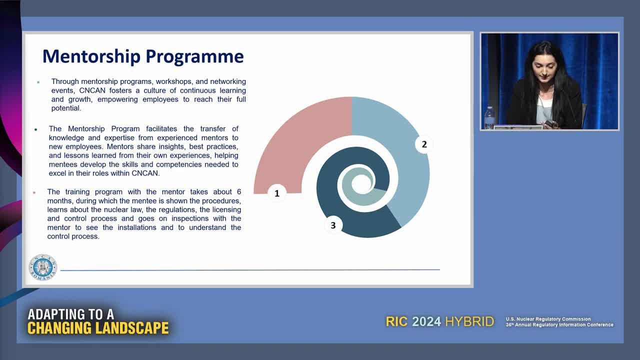 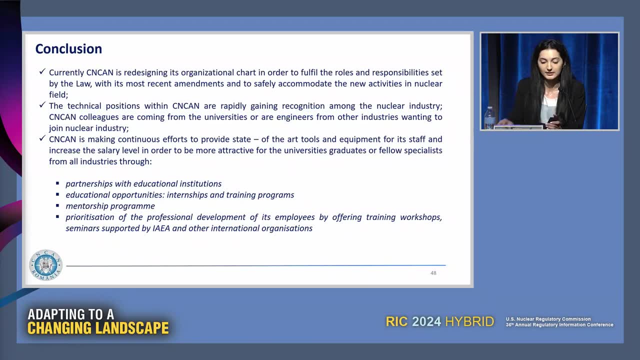 organization and understand better the control process. And, in conclusion, currently CENECAN is redesignating its organizational chart in order to fulfill the roles and responsibilities set by the law with its most recent amendments and, to safety, accommodate the new activities in nuclear field. 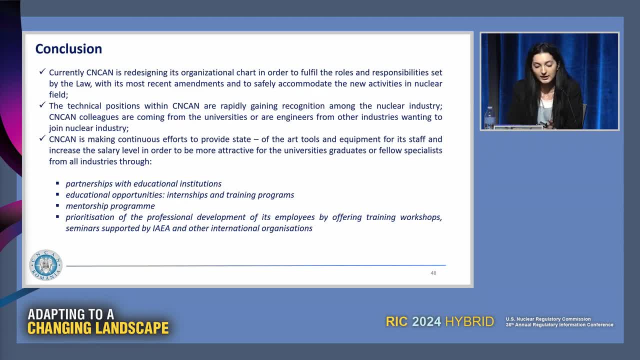 The technical position within CENECAN are rapidly gaining recognition among the nuclear industry. So CENECAN colleagues Are coming from the universities or are engineers from other industries waiting to join nuclear industry. Also, CENECAN is making continuous effort to provide the state of art tools and equipment. 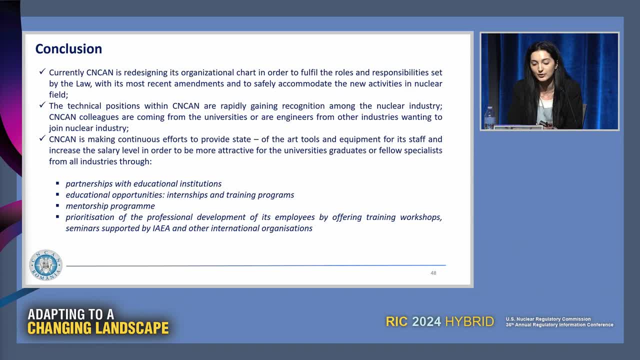 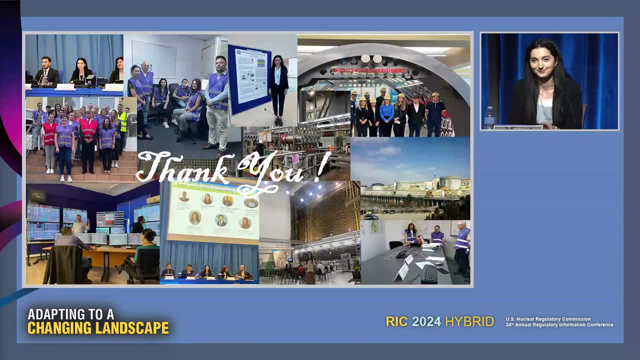 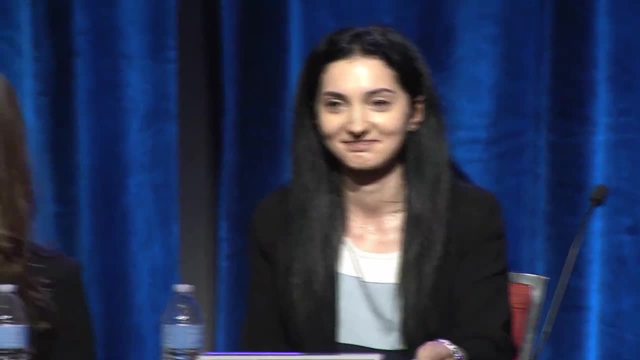 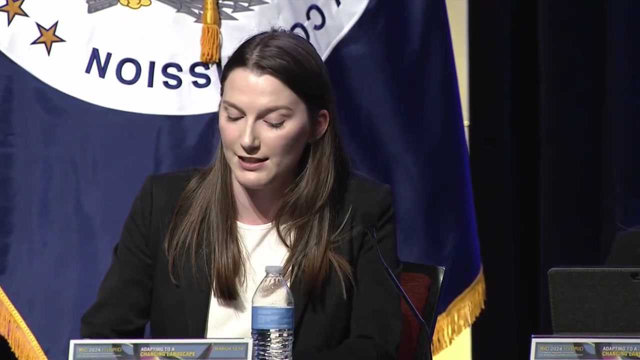 for its staff and increase the salary level in order to be more attractive for the university graduates or fellow specialized. Thank you, Thank you for your presentation, Alexandra. Our next presenter is Mira. Mira chose to work as an inspector in Fanner because she wanted to satisfy her technical 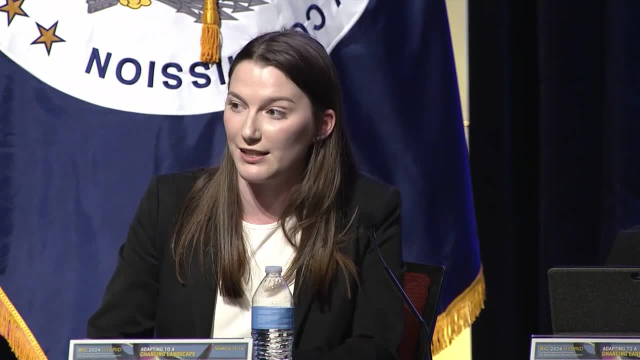 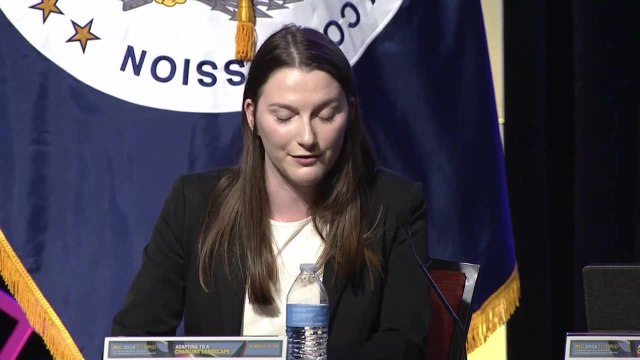 passion, while making sure that passion would serve her country and the people of the UAE. She felt that the inspector position was dynamic and inspiring. Years later, she is thankful for the choice that she has made, because it would be boring to work in any other position. 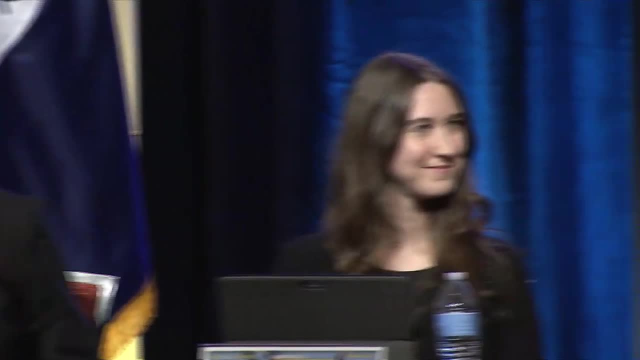 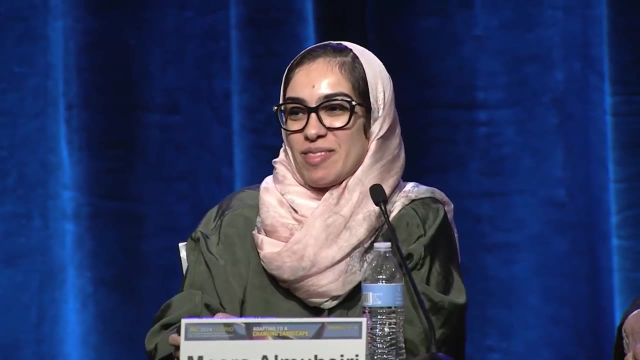 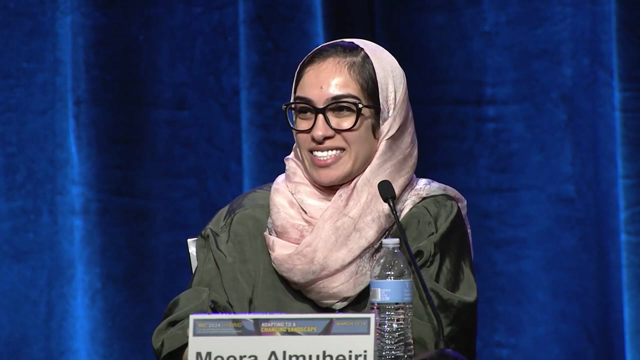 I will now hand it over to Mira to present. Thank you, Miranda, Thank you, Hello everyone. Thank you so much for everyone, all the mentors, all the great friends who have made time to come and be present while we discuss our journey. 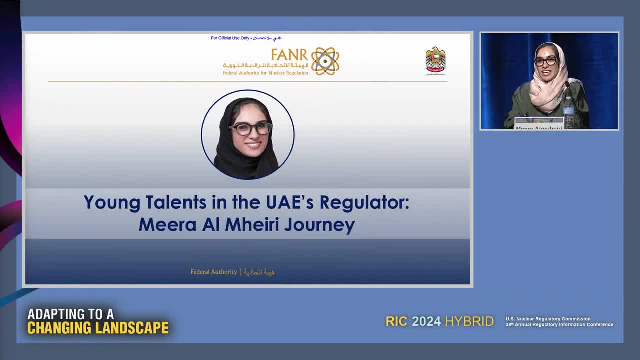 My name is Mira And today I'm going to shed the light on my journey. how did I transfer from a kid in the 90s to the first Emirati female nuclear safety inspector, and how FANR and the UAE? 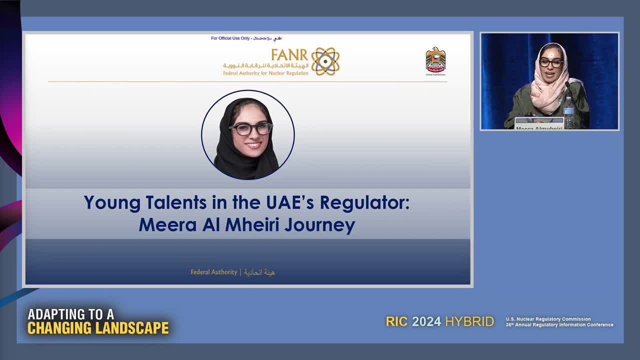 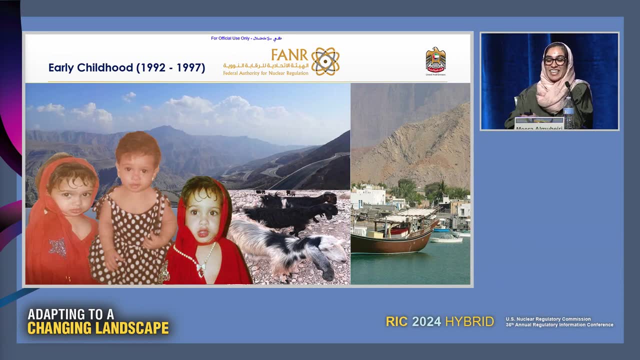 as a whole had helped me to become the person I am today. So it all started in 1992.. Two things that I clearly remember from my childhood was that I loved goats. My first pet was a goat and I used to spend every day in the afternoon going to the farm. 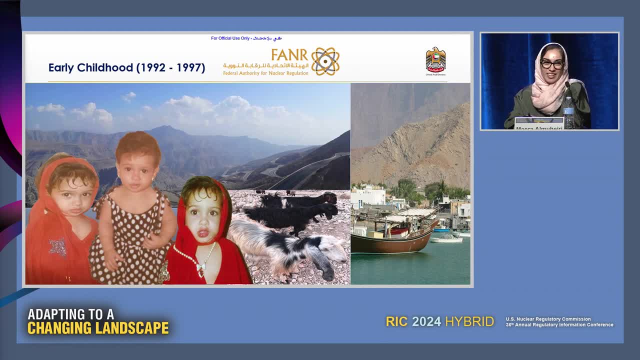 and playing with the goats. And the second memorable thing about my childhood was my sense of fashion. I learned from my mother and my aunties how to dress very colorfully and I think I still have that sense of fashion And I always admire. I remember when I saw Andrea the first. 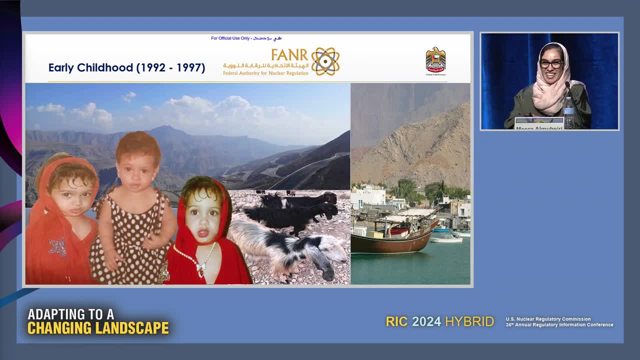 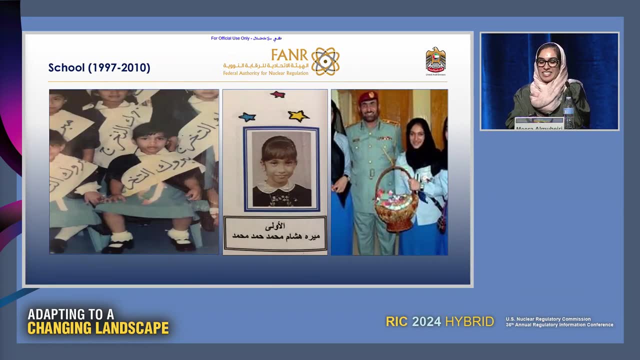 First day, second day and today. I was like girl, you have the colors, I love them. And then I moved to the school and what I remember about school days were two things: My growing passion to volunteering, giving back, working in different community activities. 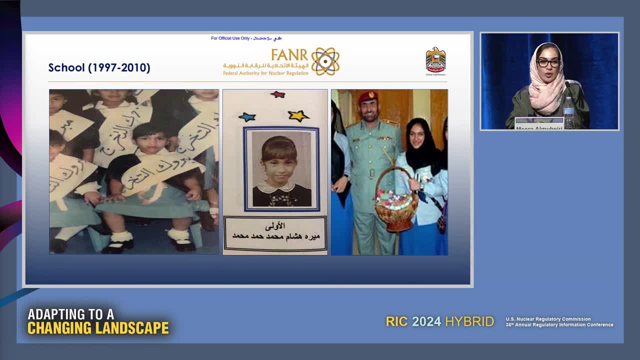 and then the second thing was doing well in school, Trying, Trying to learn, trying to commit, to grow every day. And I remember when I was in school I wanted to be so many things. I wanted to be a politician at one point, then a diplomat, then a teacher, then a psychologist. 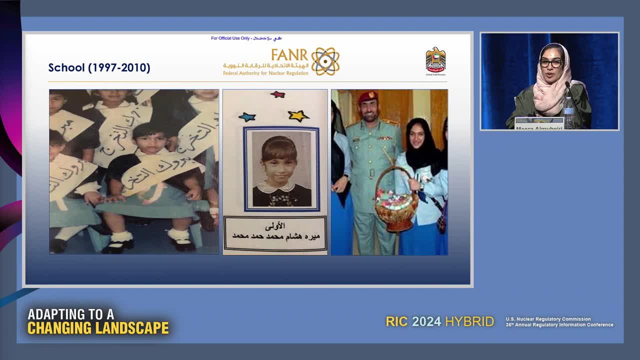 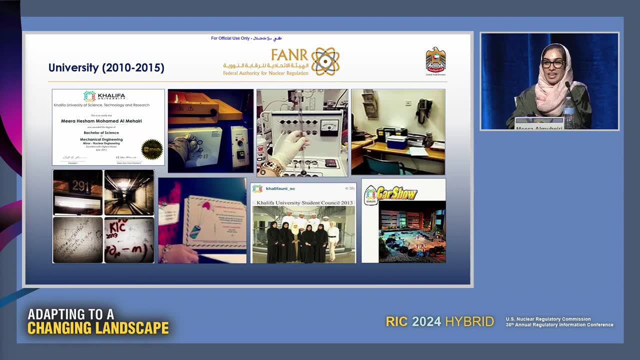 And the list kept growing. and it was only then, when I reached the high school, I figured that I actually want to be an engineer. I felt that I have- I have so many, so much passion towards science, towards mathematics, and the only profession 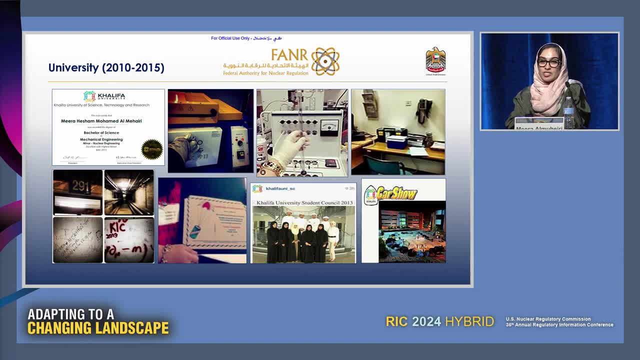 that would help me grow. that passion was engineering. So I decided to pursue a bachelor degree in mechanical and nuclear engineering And I remember that that choice, as Miranda said, was mainly to fulfill my passion towards STEM And, in the same time, In the same time, be part of this revolution in a new sector in the UAE and help to serve 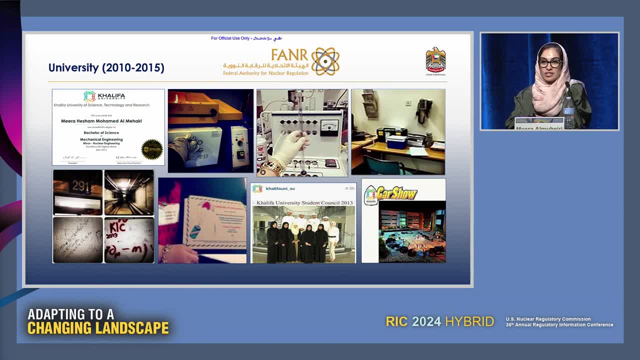 my country in that field, And in the university as well, I wanted to do so many things, So I wasn't only doing my bachelor degree, but I was doing research in the biomedical field. I did a lot of material, having fun in the material lab, creating stuff and products. 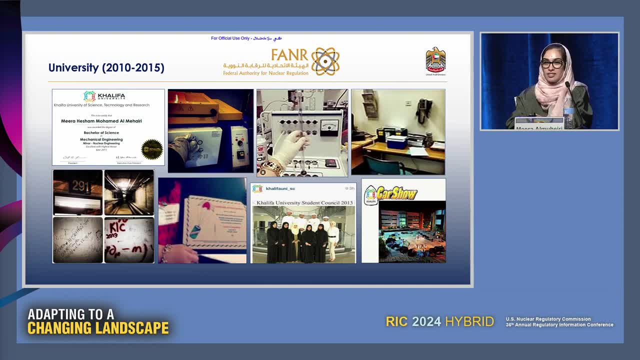 And then I decided that we want a club for cars and adventures And let's do volunteering here and then. So it was a very engaging life full of different activities, and I wanted to get to know to the different personalities that I have within that actually love to try so many new things. 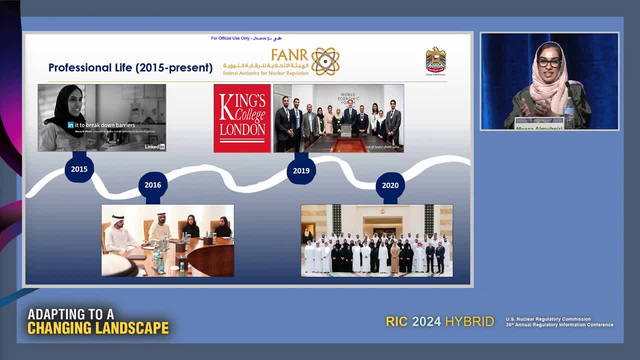 and the same curiosity, the same desire of learning and getting to know things in different fields continued during my professional life. In 2015, I started my job in FANR, the UAE regulator, and become the first Emirati female to serve as a nuclear safety inspector. 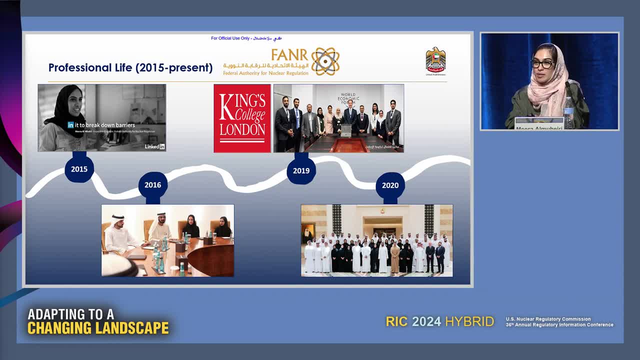 It was an amazing journey because it really suited my personality. I didn't want something boring, I wanted something challenging, something that I aspire to grow in, something I need to learn every day and something that is dynamic, And I felt like, as Miranda mentioned, that being an inspector is really the right fit for me. 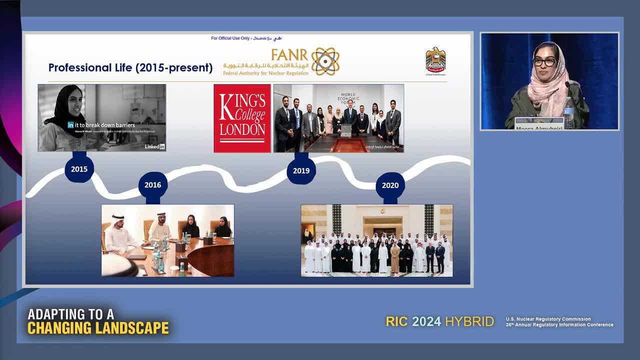 And in 2015, I started, And now in FANR, we have more than 38% of our workforce who work in these technical fields. Ladies who are inspiring, ladies who I work with every day, ladies who teach me, and we always have engaging conversation. 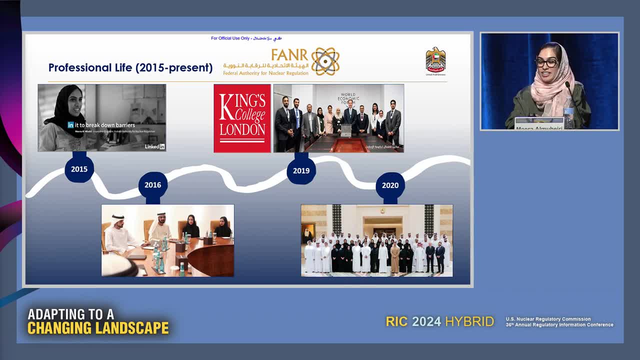 not only on the local level, but also in the international arena, A year after I was selected by the government To work as an advisor to the UAE government with regards to youth policies and strategies, As you know, and as DJ Krister mentioned previously, that we are a very young nation. 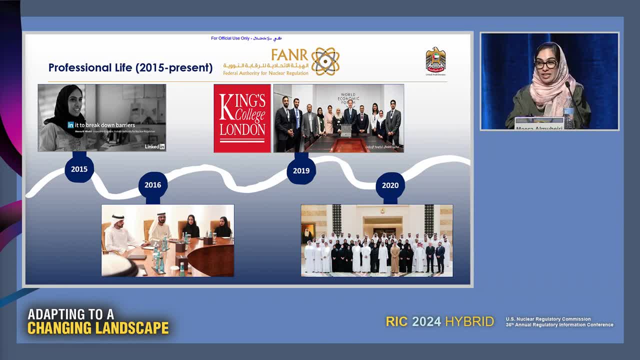 The youth population is around 60% of the UAE And such a young nation needs to be listened to. We need to understand continuously what are the desires, what are the desires of our youth, what do they need? what do they aspire to? 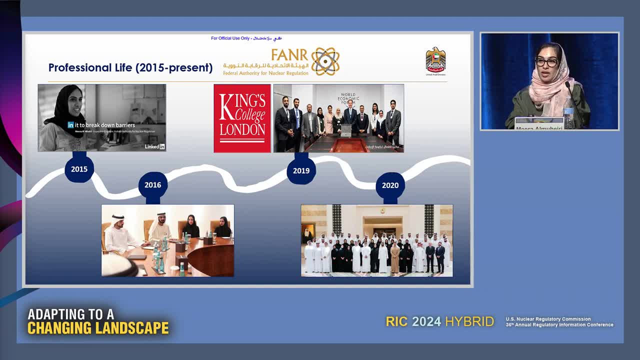 what are the challenges that they're facing, so that they grow beautifully and contribute to the peacefulness and prosperity of our country. So it started over there, and then, years later, I reflected on myself And I thought: what else can I do? 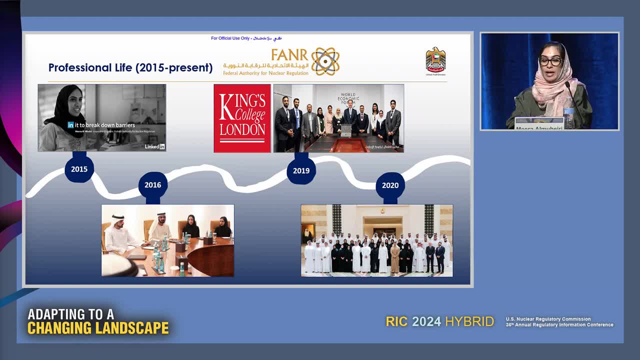 Is my engineering background enough to help me do my work in FANR And, as well, my advisory roles within the government? The answer was no. it's not enough. So I decided to pursue a degree in King's College London. 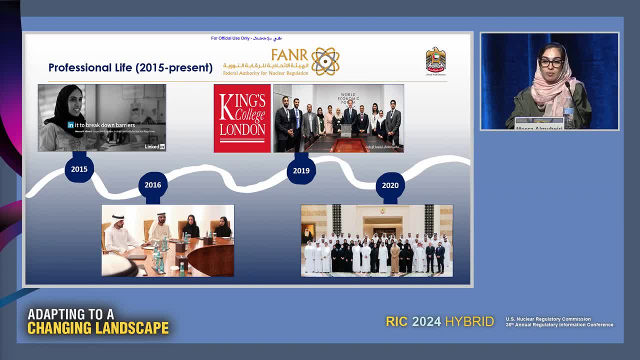 And I was mainly studying international affairs. but remaining loyal to the nuclear field, I specialized in nuclear intelligence and security And that opened a lot of doors, I would say, to my career, And I think that's what I'm going to do for the rest of my life. 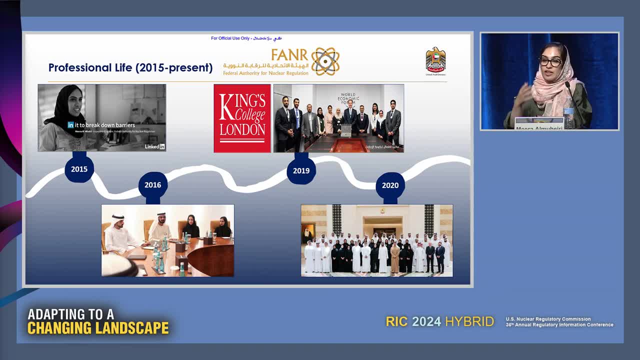 And I think that's what I'm going to do for the rest of my life. I think that's what I'm going to do for the rest of my life Because it gave me a different perspective on how the three S's integrate the safety, security and safeguard within the nuclear sector. 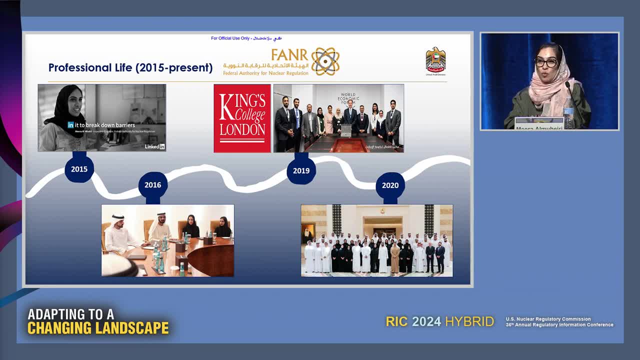 but also gave me a broader understanding of how and why international affairs are very important, especially in the nuclear field. Within that year as well, I received the government again recognition and support And I was selected to be part of the Delegation to the World Economic Forum. 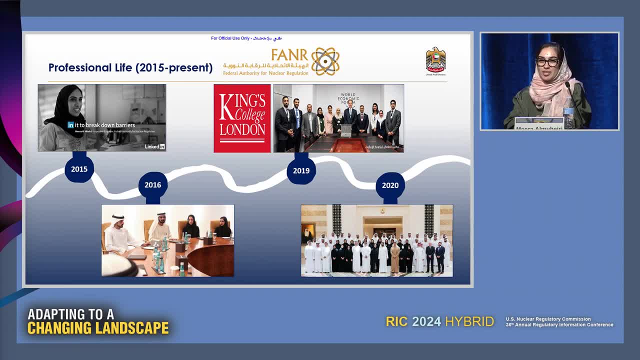 Just being there and representing youth. All the ministers were having back-to-back meetings and doing a lot of hard work And I was just there enjoying my time and learning from our ministers, And it felt extremely good to know that our leaders really support youth and support women. 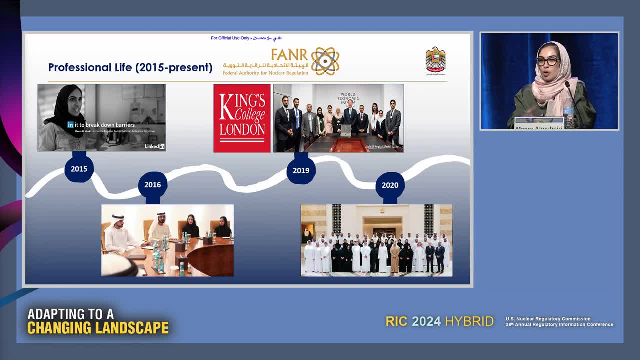 And they actioned that. It's not just propaganda or just words. They're actually really actioning that from a higher level, a strategic level, up to the working level. A year later, another resemblance of such support. I was selected as one of the very young board members in the UAE government. 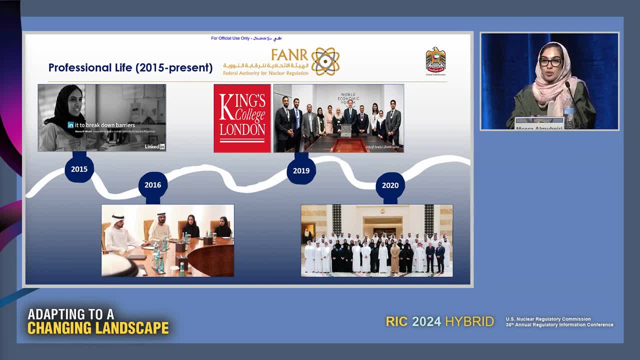 serving in one of the government entities, which is the Supreme Council for Motherhood and Childhood. It was a very nice opportunity And I got questioned: you're a nuclear engineer and you're not even a mother. How could you serve on that board? 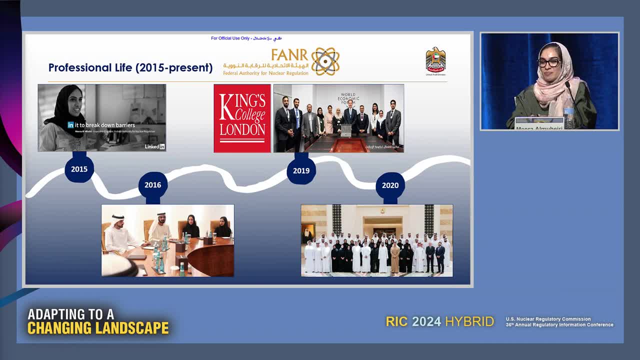 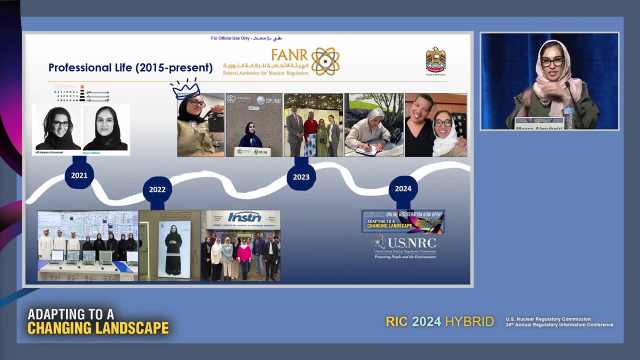 But again, I think the diversity of different knowledge and different skills that are brought and that are appreciated by our government from the nuclear sector is what made me sit on that board. Thank you In 2021, another resemblance of our leaders' appreciation and support. 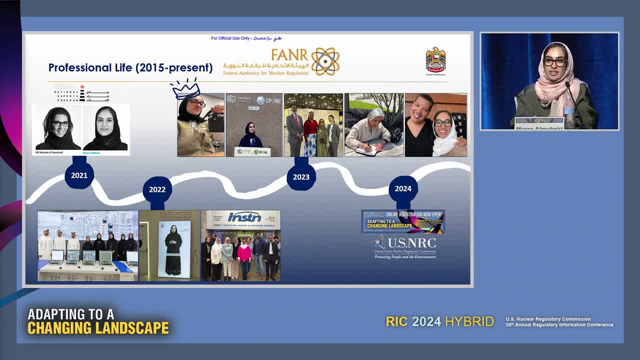 and also FANR's engagement in my personal journey. So I was selected to be part of the UAE expert program, serving on the policymaking field, And in that it was my opportunity to inform the policymaking sector with regards to how we do it in the nuclear. 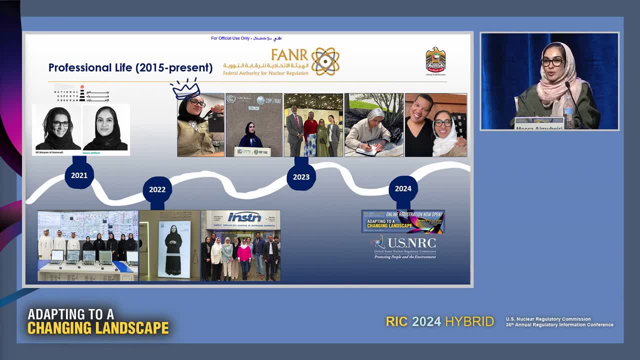 And years after, I saw multiple solutions that were created and were inspired actually from the nuclear sector. In 2022,, I had the privilege to graduate from the Senior Reactor Operator Management Certificate, then have been seconded for a training in France. 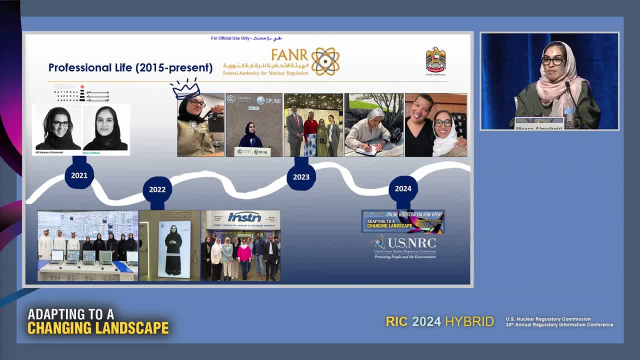 learning about material and fuel, and then met a lot of great people from around the globe who are my mentors, my friends and a great network of what I call sisters. And today, in the USNRC RIC- it's my first RIC- 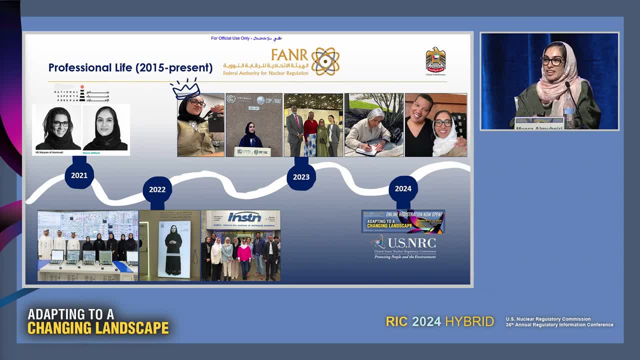 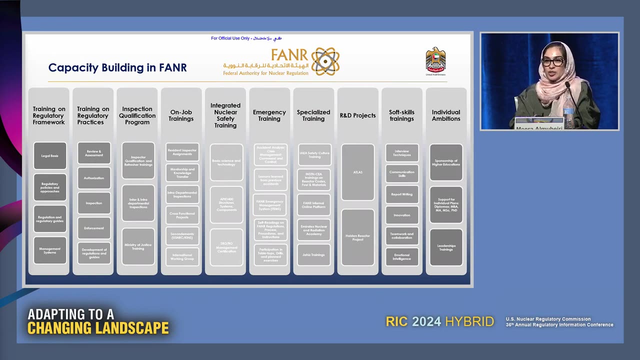 Very memorable, beautifully done, beautifully executed, and it's the best place to network And get to meet old friends. All of what I did, I couldn't do it by myself. It started from the UAE strategic direction of engaging youth, empowering youth across all sectors. 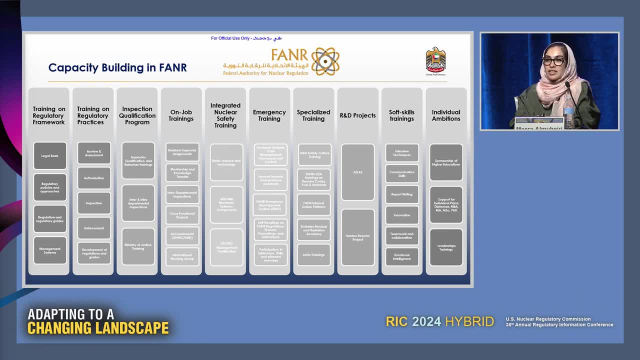 and then it was effectively implemented by FANR through systematic training and capacity building programs. So in FANR- me and my young colleagues- we have different options to learn and grow. every day We get or we start our journey by training. 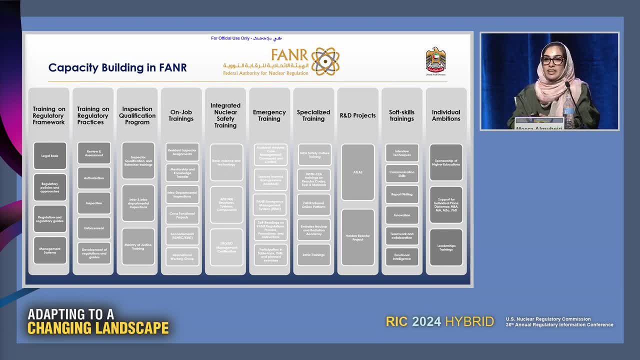 being trained on regulatory framework, understanding the regulatory philosophy, the legal basis. Then we get to understand what is our job as a regulator, What are the processes that govern our work. Then we get qualified as inspectors. Then we do a lot of on-job trainings. 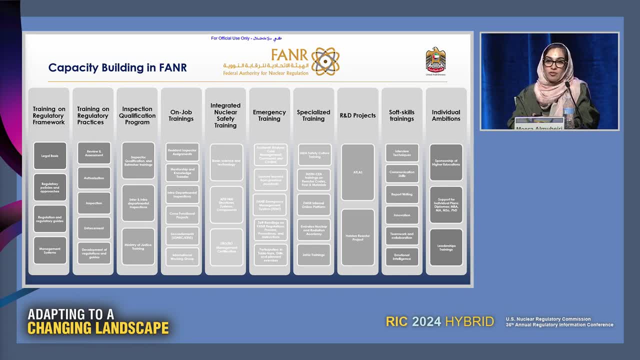 Whether we are situated in the site in Baraka for a couple of months and become resident inspectors, Whether we go and shadow our expertise, who come from all over the world. And then we have multiple other modules where we have extensive training on the systems, the structures and components. 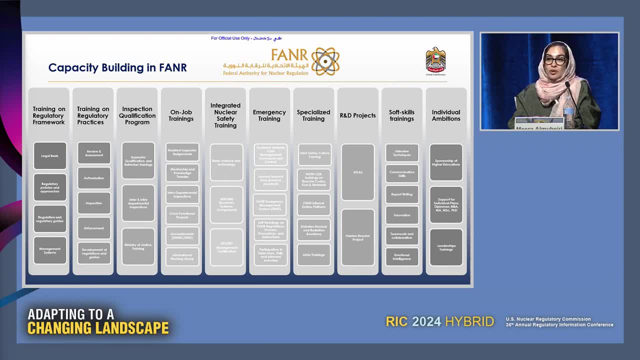 We get to learn about emergency research, and I had the privilege to work with Halden and developed that mindset of research and how it actually gets integrated in the nuclear sector. Then a lot of soft skills. It's not only how you conduct your job as a regulator. 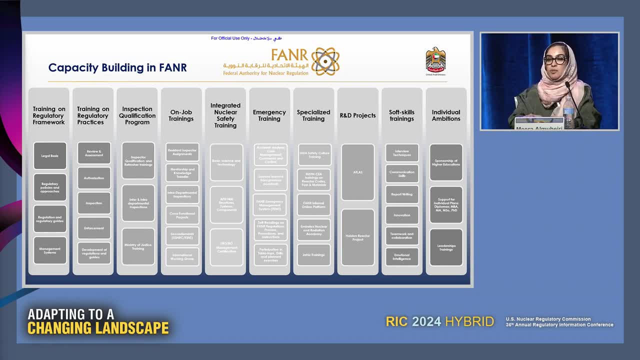 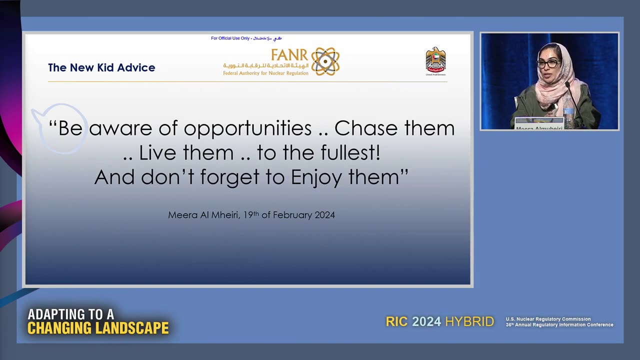 but how also you communicate as a public servant with the public and making sure that your job is actually making them safe, and you can communicate that. So I believe that I wouldn't be here without the support from my leaders from the EU government. 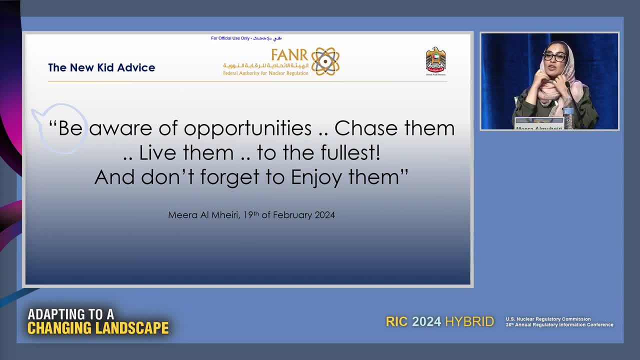 Not only to me but to all the youth of the UAE, And also the systematic approach that FADR has developed and put in place to support the younger generation. And if there would be one advice that I can give as a new kid in the block. 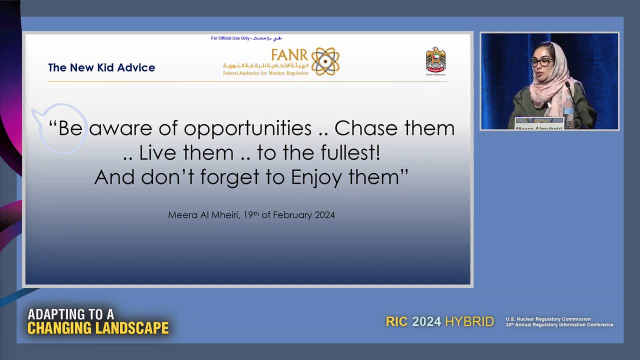 it would be to be aware of opportunities. There will always be opportunities Within your organization, outside your organization, and you might also create those opportunities. So be aware of them And once you kind of feel that these are the opportunities for you. 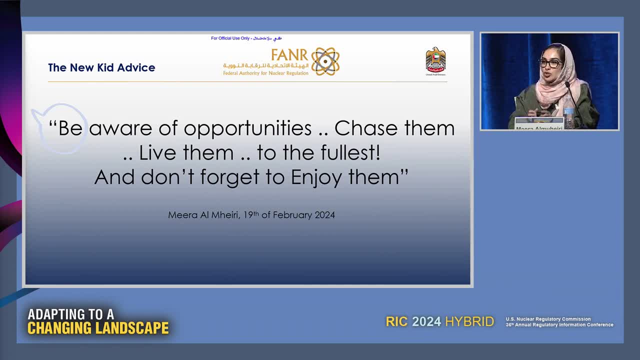 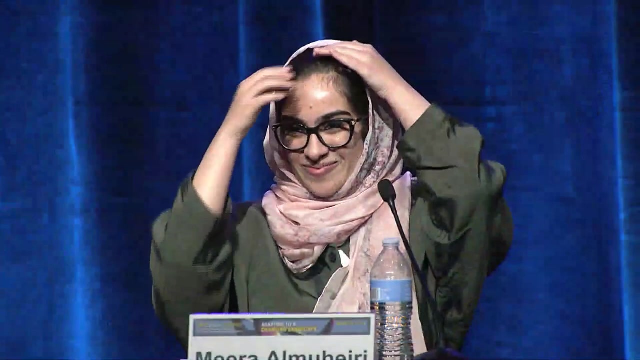 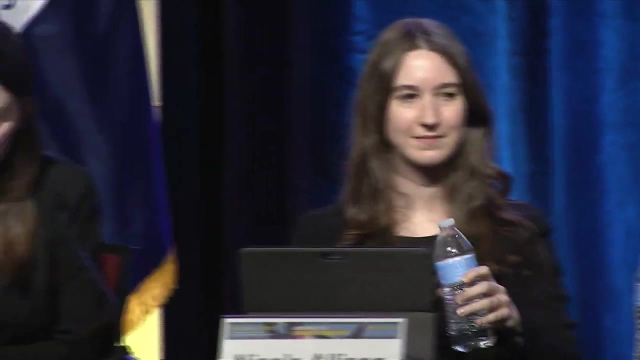 go and snatch them, Utilize them, Use them, Enjoy them And then, later, you would realize how important these opportunities were in shaping your personality and you becoming the person that you are. Thank you so much. Thank you for the presentation, Mira. 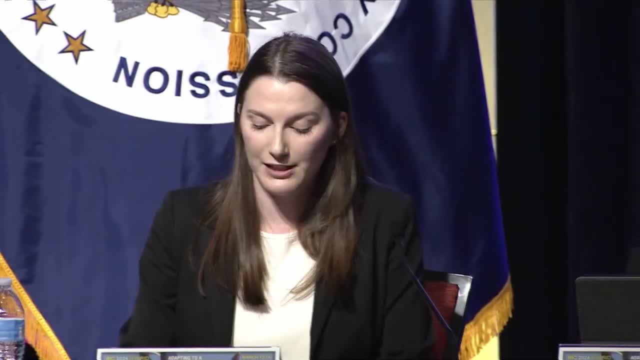 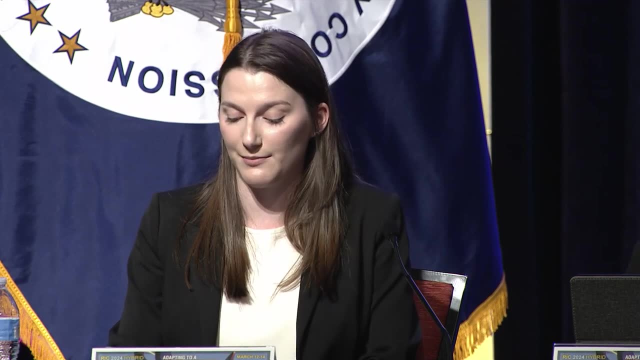 Our final presenter is Soratos. Soratos has always believed that public service is a meaningful job. He wanted to work in engineering since he was young and, upon his graduation from engineering school, the Office of Atoms for Peace had a scholarship program where he completed his PhD. 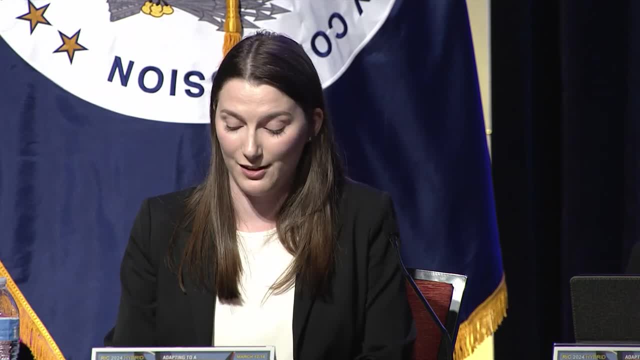 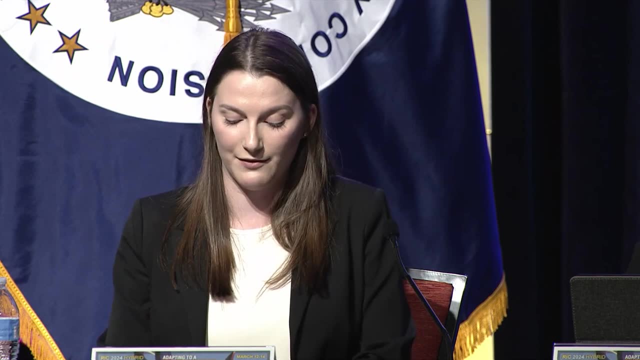 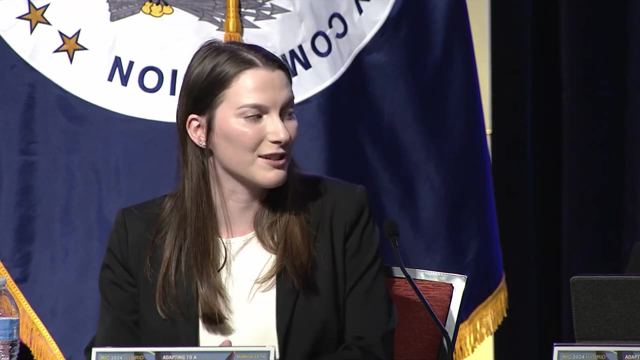 Working as a nuclear regulator is not usually a hands-on operation or research, but involves continuously learning, scrutinizing and inspection, And inspection of the technology and innovations for the nuclear industry, which has always entertained him. I will now hand it over to Soratos to present. 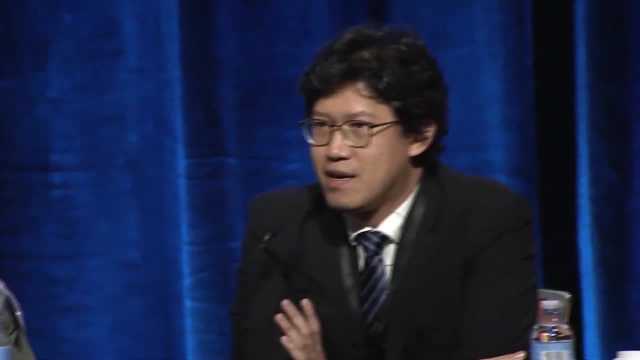 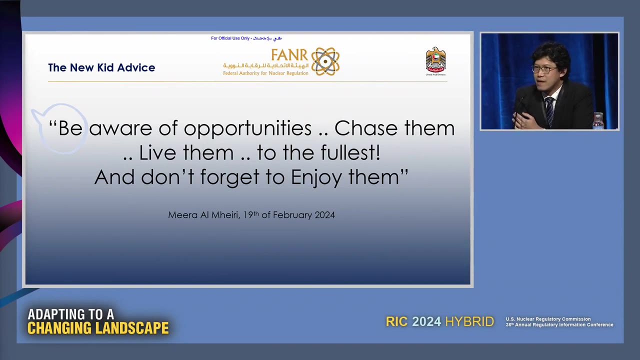 Thank you very much, Miranda. Good morning, It is my honor to be among the panelists and to be the only man on the stage, And thank you very much for the opportunity to present some of the activities in Thailand on building the talents in nuclear safety and security. 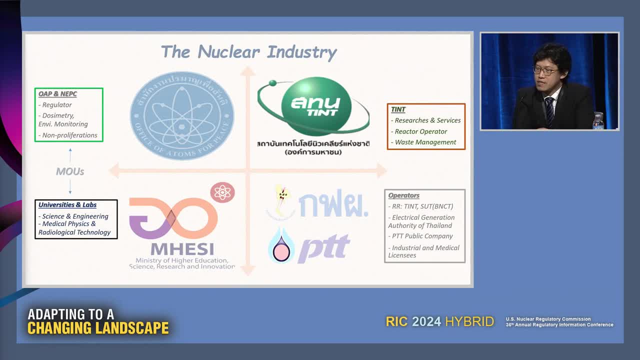 So I would like to just go directly to the introduction of who is who in Thailand in the nuclear industry. So first, on the top left, we have the OAP as the nuclear regulator. We also have some capabilities on dosimetries and environmental monitoring. 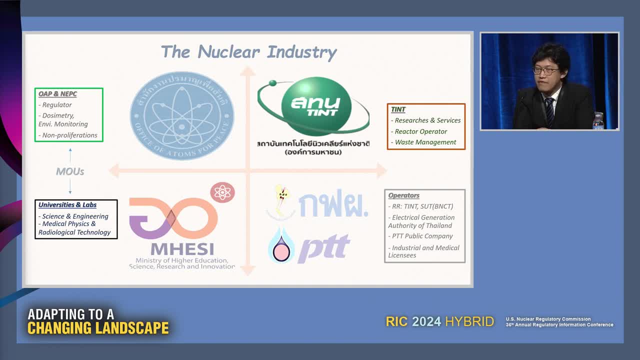 And OAP also supports the non-proliferation regime of Thailand. And then on the right side we have the Thai Institute of Nuclear Technology, who is our research reactor operator, and also the waste management facility, And then both of the organization belongs. 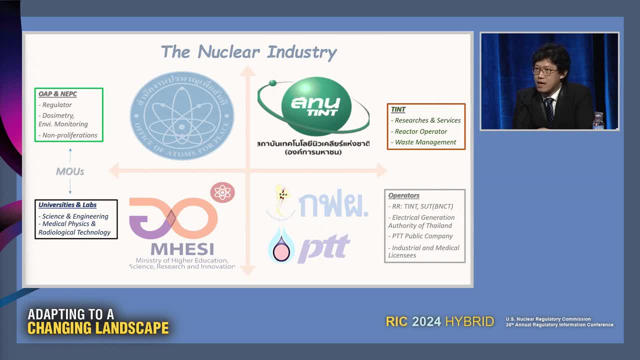 to the Ministry of Higher Education and Science, and then, on the bottom right, we have the utilities. who is the EGAD, the Electrical Generation Authority of Thailand? who is the prospective operator of the nuclear power plant? And we have thousands of radiation isotopes licenses. 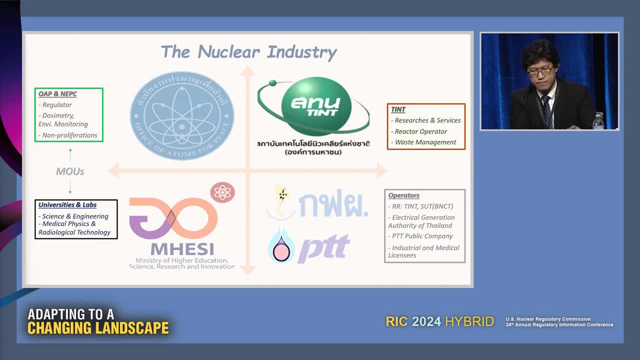 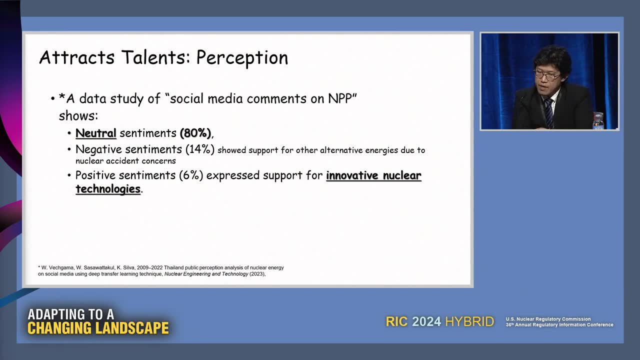 in Thailand. Then, to talk about building talents in the nuclear industry, I thought it might be useful to look at the current perception of Thai people on the nuclear power plant. So there is a big data study of the social media comments: Facebook comments. 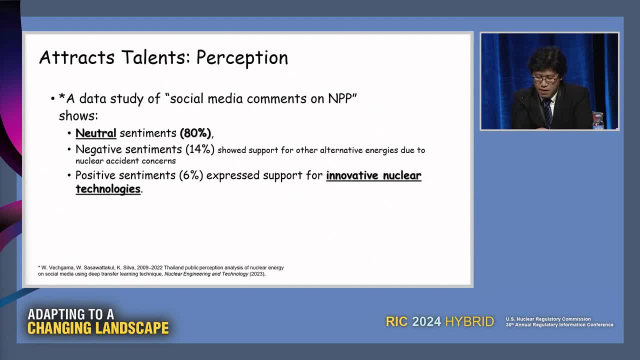 from the year 2009 to 2023 on the subject of perception of Thai people on nuclear power plants, which reveals that the majority of Thai people- about 80%, still believe still have the neutral sentiment on nuclear power plants. So, although there are several incidents, 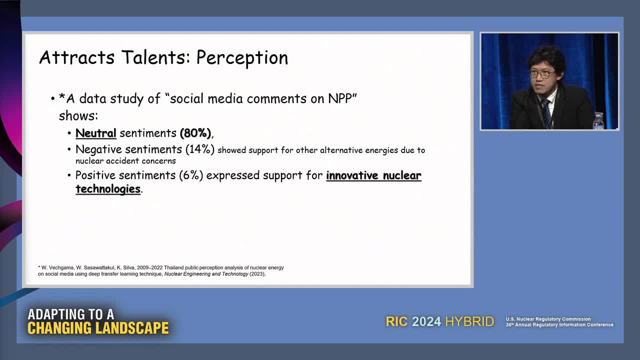 during the past decades. that challenges the public acceptance of nuclear technology. the majority of Thai people still consider nuclear power plants to be one of the potential energy solutions And therefore, at this time, I still believe that we still have the opportunities to convince people. 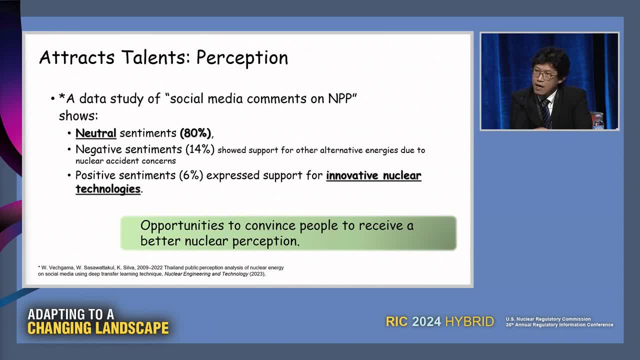 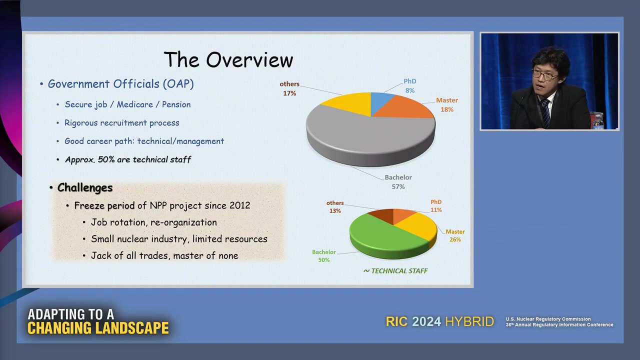 to receive a better nuclear perception and attract them to get involved in the industry. And it is also found that those who support nuclear power plants focus their discussion on innovative nuclear technology. So now looking inside the regulatory body, the OAP, so at the current moment, 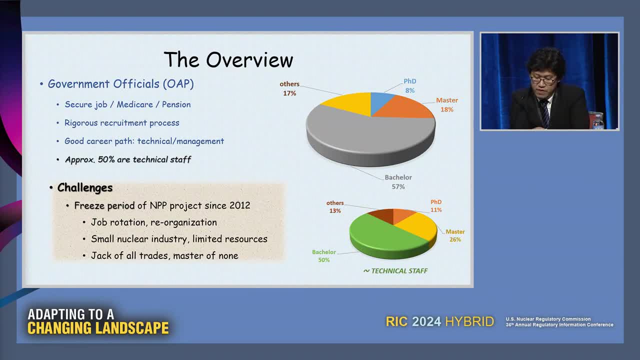 the workforce of the OAP. we are all civil servants and approximately 50% of the staff are technical personnel. However, there is a challenge since the freeze period of nuclear power plant project in 2012.. There were internal job rotations and reorganisation. 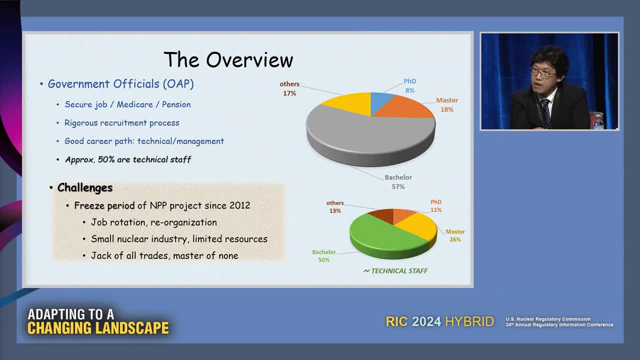 Also, some technical staff moved to other government or governmental units or other provinces And since the industry was not expanding and with limited number of personnel, technical staff might not be able to focus only on one expertise. It is often that one person might be assigned to take on. 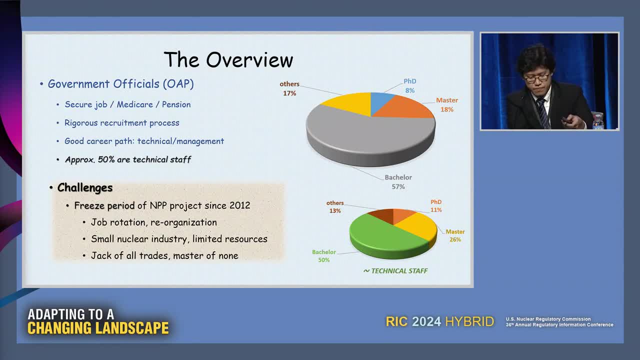 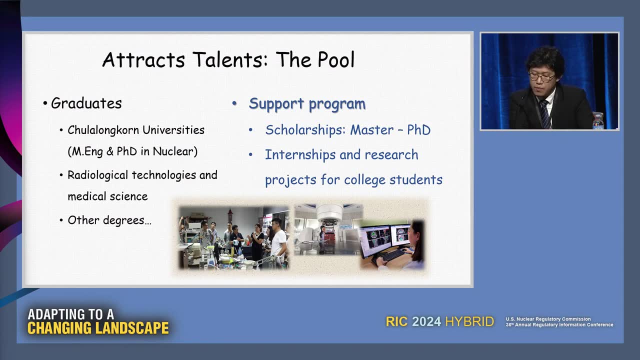 two or three duties And, as I mentioned, that approximately half of the staff are technical personnel, Most of them received their degrees from national university in science, engineering or radiological technology, But also in order for OAP to obtain personnel with specific expertise. 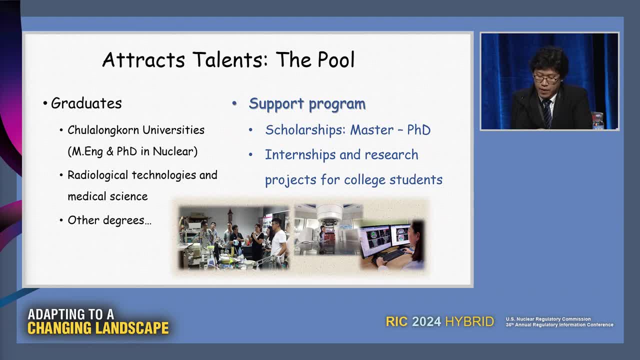 OAP can request the Thai government for a scholarship programme for our staff to further their education in the field of nuclear in the national or international universities and then come back to work at the OAP after obtaining their degrees. Nevertheless, although OAP regularly recruits, 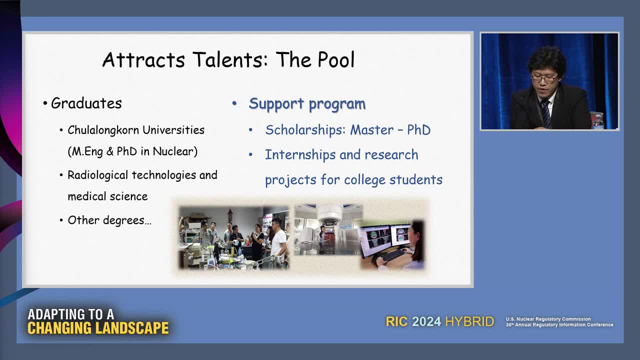 university graduates. there are a few cases where the recruits, especially those who have master or PhD degrees later, prefer to move to work in academics or research instead to pursue their personal interests. So therefore OAP tries to deliver more communication on the roles and functions. 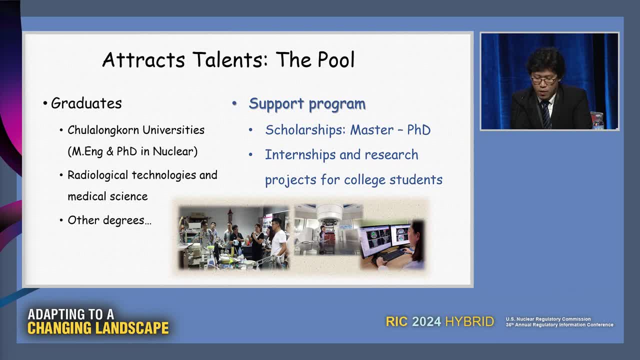 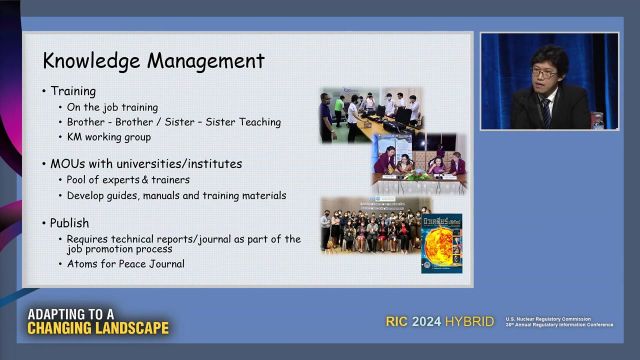 of nuclear regulatory body to the public. to help the graduates to have clearer expectations of the nature of the work Before making their decision to work in the regulatory sector or any technical support organisations Now. to ensure that our staff have the necessary competency to carry out their work. 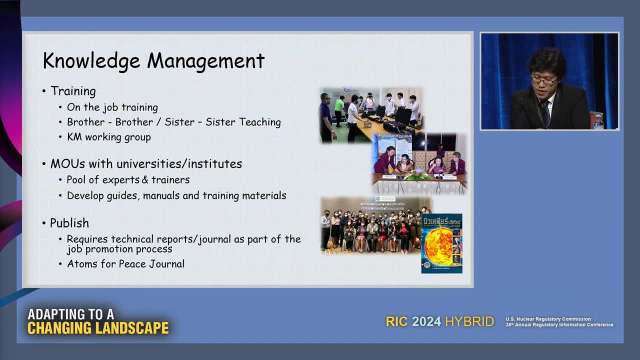 OAP mainly uses on-the-job training within each division, But in addition, OAP has recently set up a knowledge management working group to help analyse the gap in the training and also prioritise the topic of the training And during the past few years, 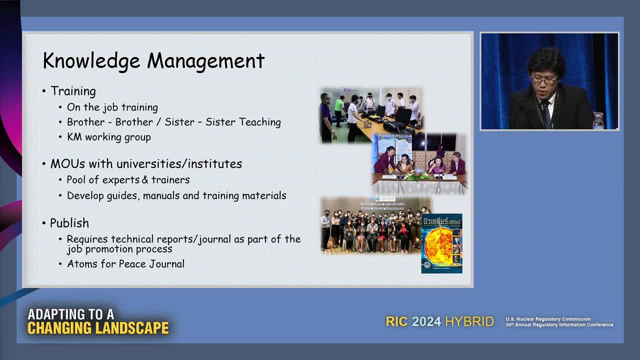 the working group has organised knowledge management programmes in the style of brothers and sisters training, So which aims not only to promote knowledge transfer but also helps promote a more friendly and relaxing working environment. So we also encourage corporations and technical exchanges between OAP and the university. 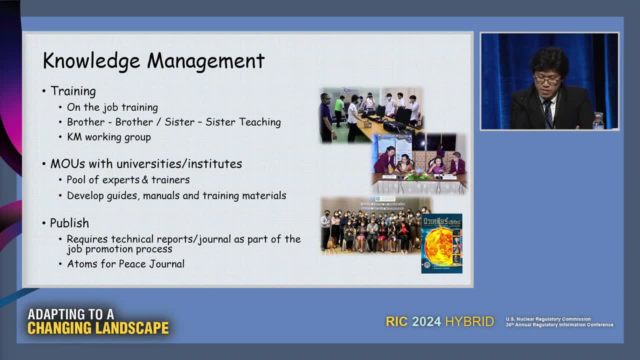 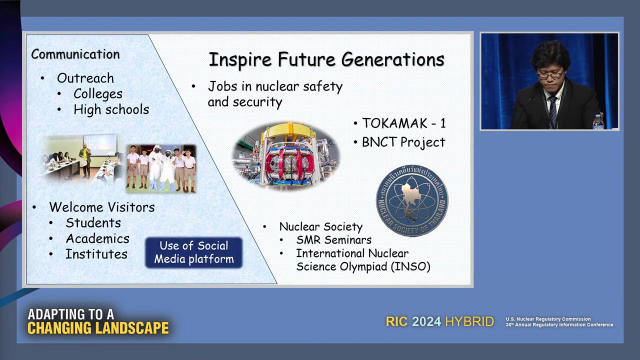 since OAP and all the public universities are already under the same ministry And our technical staff are required to write technical papers as a part of the job promotion and encouraged to publish articles on any nuclear related topics. And there are nuclear activities in Thailand from. 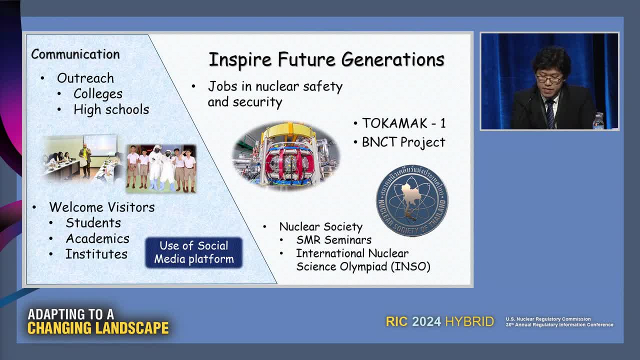 both from the OAP and from the organisation in the industry that help promote public perception towards the use of nuclear technology. OAP regularly organise visits to schools and universities to communicate about nuclear and radiation safety, And we also use social media as one of the public communication methods. 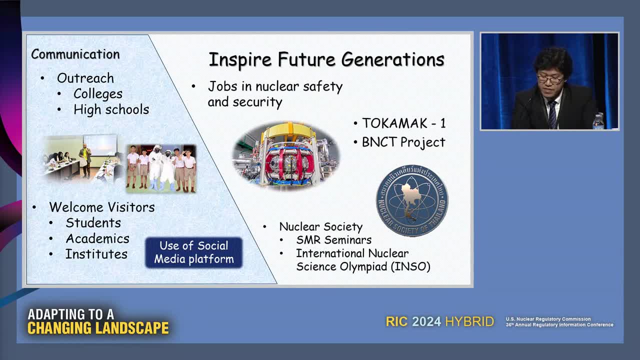 And we welcome visitors from academics and other governmental units to observe some of our laboratories and to learn about our regulatory activities. And on the nuclear application side there is the Tokamak project by the Thai Institute of Nuclear Technology, which received great attention from the public. 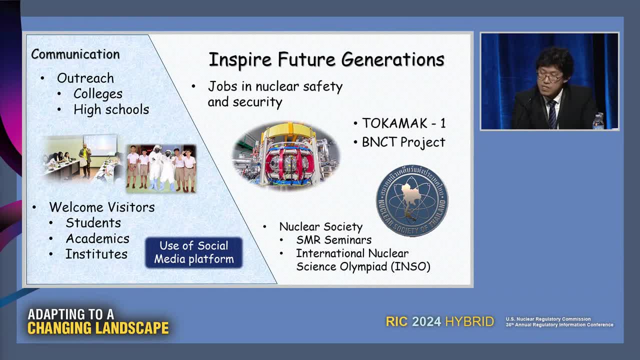 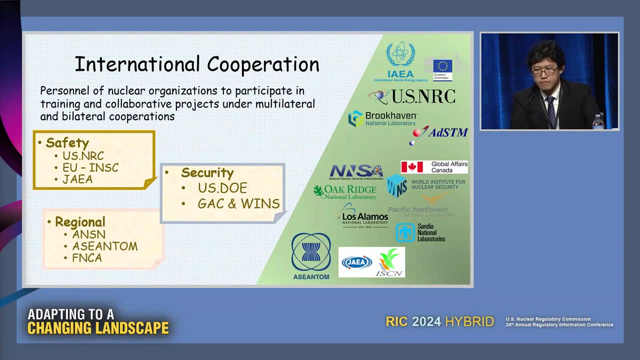 And also there is the Nuclear Society of Thailand, who is currently very active on the topic of SMR technology and on the topic of promoting education in nuclear. So we are very, very proud to be part of this. Thank you very much, Thank you. 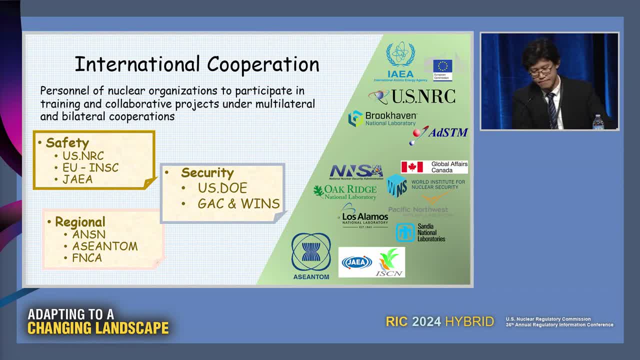 Thank you very much, Thank you. Thank you, Mr Chairman. Thank you, Mr Chairman. I think we will hear from Mr Noonan about the potential and potential for the future of this programme. Mr Noonan, you are the first. 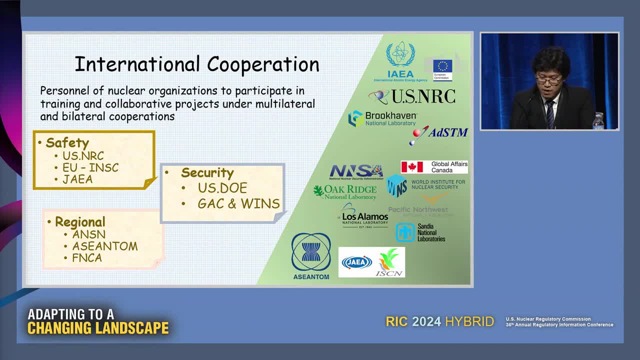 to speak on this topic. I will start with Mr Noonan. Mr Noonan- I think he is the first to speak- to maintain the necessary competence. There are bilateral cooperation on nuclear safety and security between Thai government and the USNRC and the 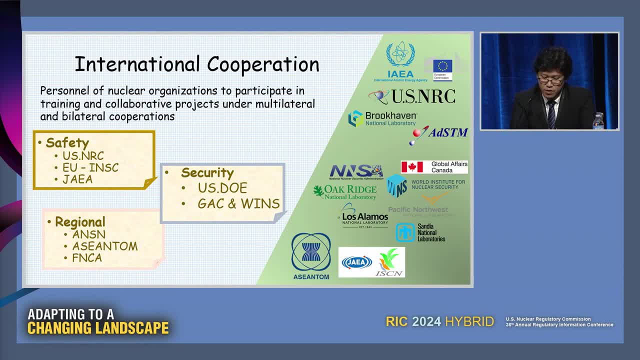 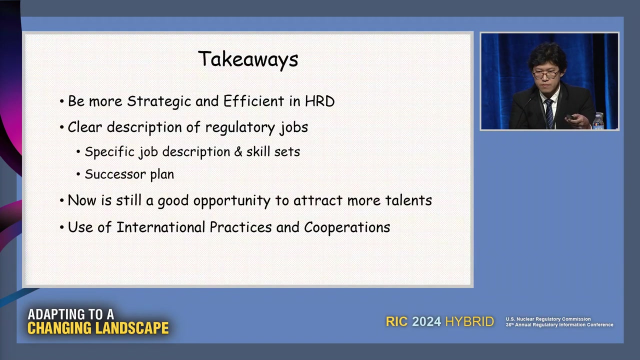 USDOE. Also, there is the cooperation among ASEAN countries, where activities such as the ASEAN-TOM and technical cooperation of research reactor operation between Thailand and the Philippines, and also activities such as the joint border exercise between Malaysia and Thailand. Lastly, the takeaways of some topics that 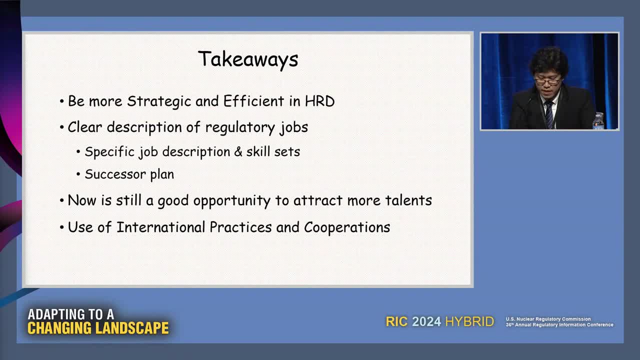 OAP should focus in fostering the current and next generation workforce for nuclear regulation and for nuclear safety and security industry. that is, we need to be efficient at managing expertise and always think ahead about the future program. and then OAP needs to focus on specifying, updating a clear 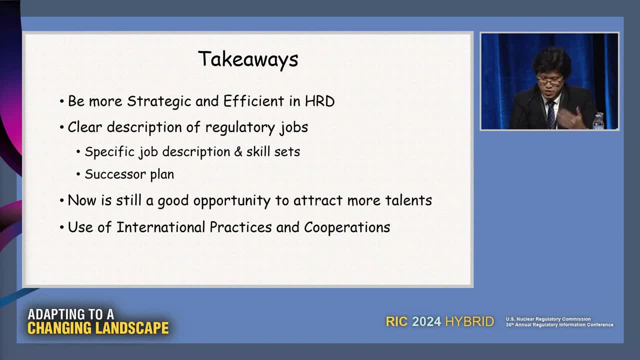 description of each job, each task in our regulatory roles and the skill sets that are necessary. The third one is too many people, especially the younger generation. in Thailand, Nuclear technology is still considered a stimulating subject and it is important for the regulator and industry to communicate and 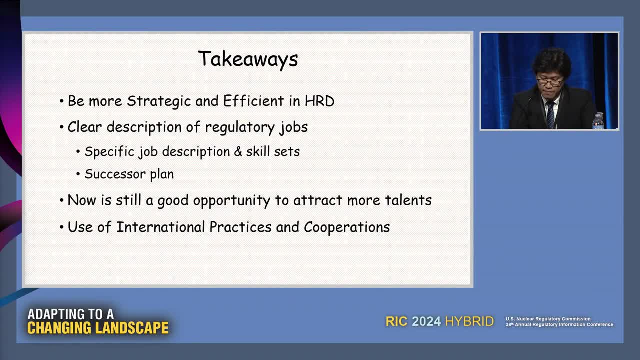 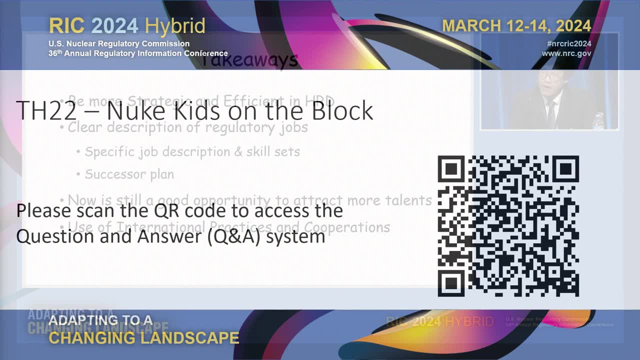 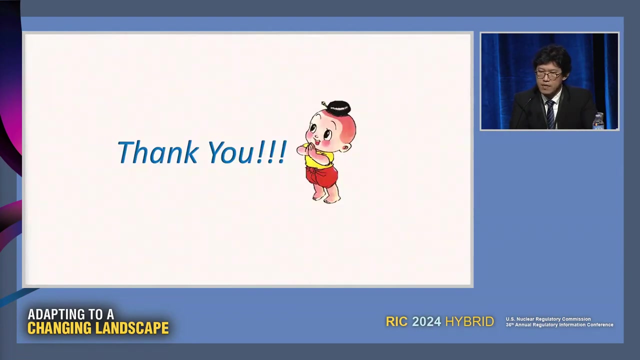 to help ensure the confidence in technology and make nuclear subject open and accessible. And finally, uses of international practice and corporations will help ensure the safety and, at the same time, ensure the sustainable growth of nuclear application in Thailand. Again, thank you very much and it is my great pleasure. 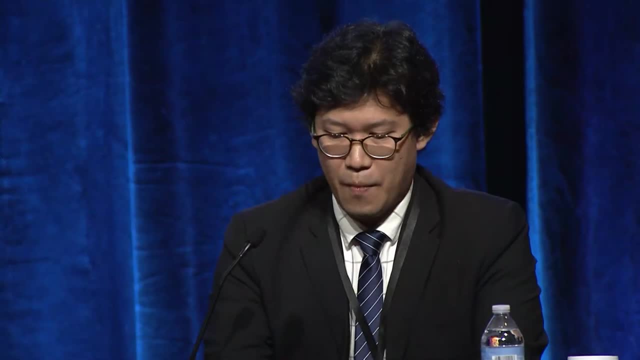 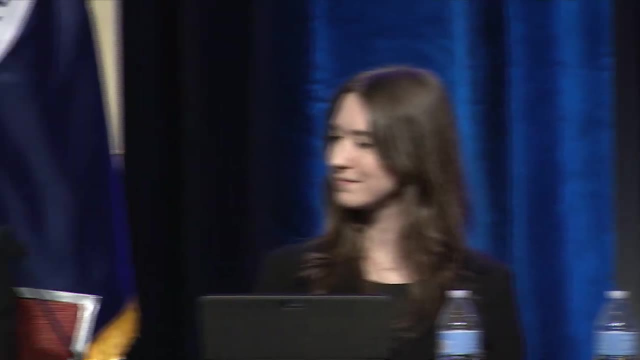 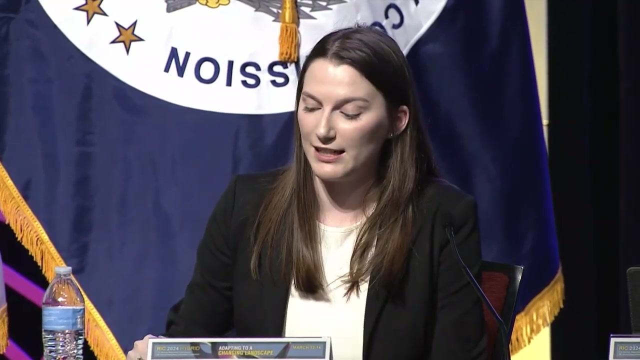 to be here. Thank you, Thank you all the panelists, for those great and informative presentations. It was really great to hear about what your organizations are doing. So at this time we're going to transition to the Q&A portion of the session and we have 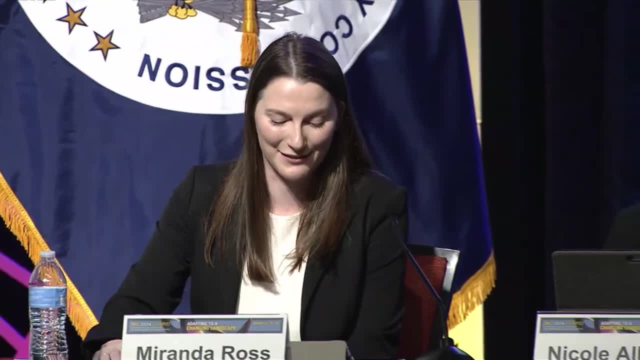 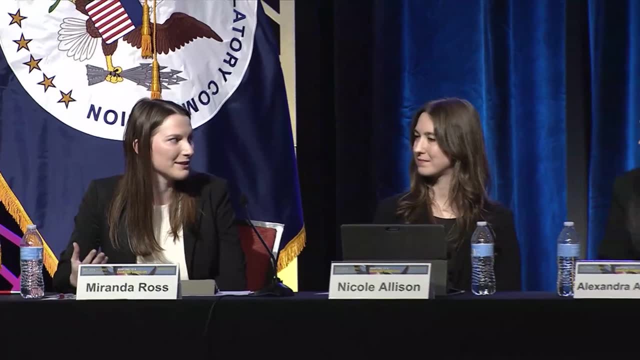 a lot of questions, So thank you to the audience for being so active. It's really great to see. I'm going to start out with a question that I'm going to direct to Mira, but then I'll open it up for anyone else, especially the other women on the. 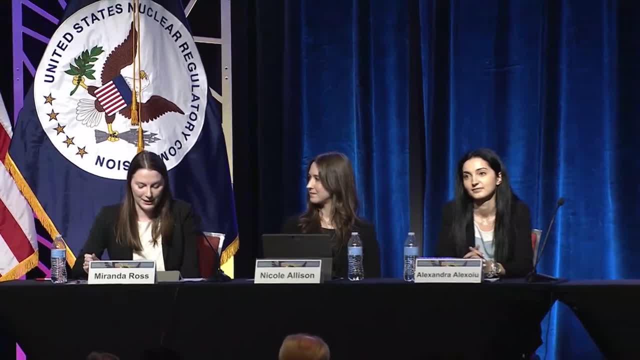 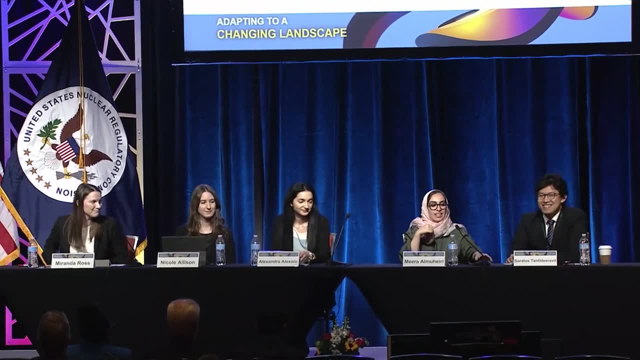 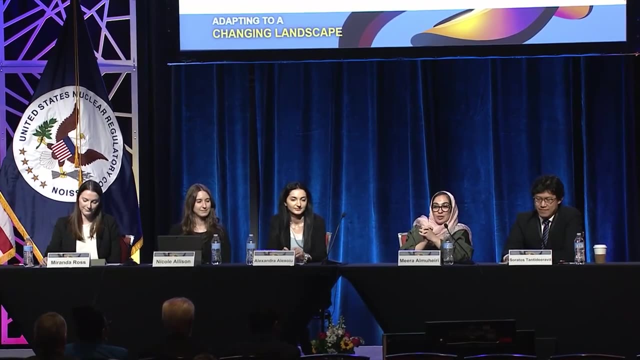 panel. What can I do to excite my daughter to pursue a career in nuclear? and what excited you? I love this question, so I'm really excited to hear what you have to say. Thank you for the question. So I think the first thing to do as a good parent. 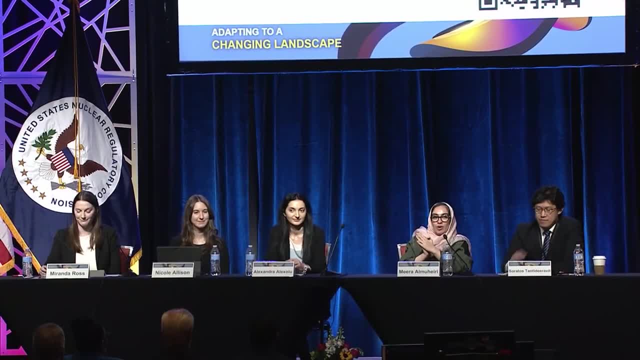 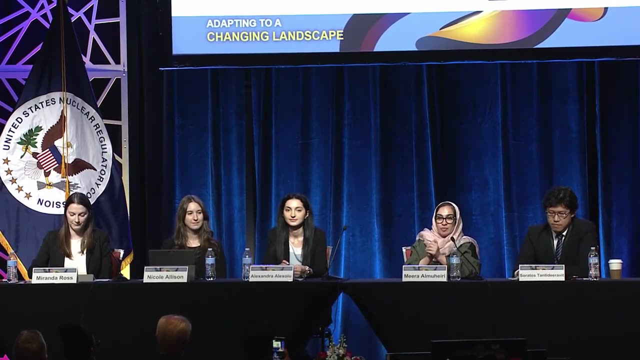 is to always support your kids, Whether they want to pursue a career in the nuclear field or other field. I think that support in itself and that freedom that a parent can encourage their kids is very important. So first of all, support them, regardless of 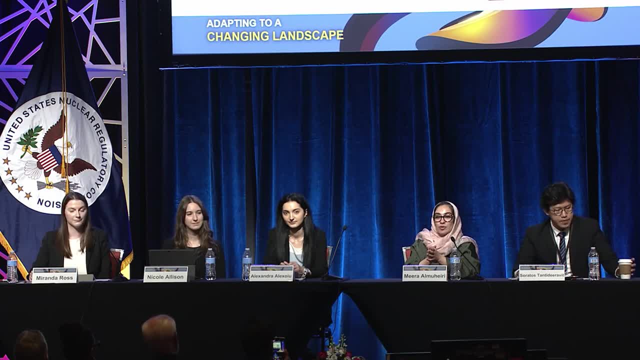 whatever field that they want to pursue And then if you kind of want them really badly to join the nuclear field, it's very important to showcase why. Why nuclear is important. It's contributing towards environmental causes, cleaner energy and all the good. 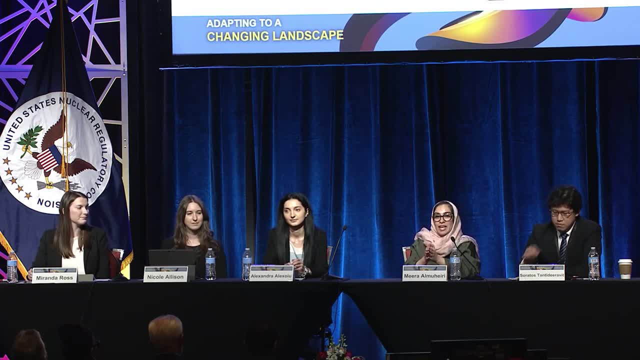 things that the nuclear sector bring, But also focus on the human aspect. If you are in the nuclear field, I'm sure you have so many great stories to share, So try to share these stories, and if they decided to pursue a job in the nuclear, then that's great. If not, then always. 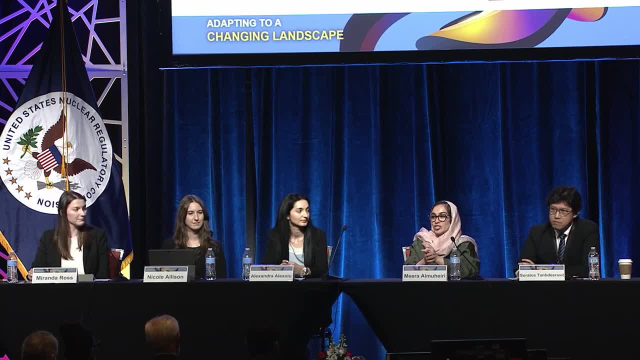 support them. In the nuclear field, not only engineers are needed, but a vast variety of expertise and skills are needed. So encourage them, and I wish them all the best in whatever choice that they make. Does anyone else want to add anything? Great answer, Mira, I think. 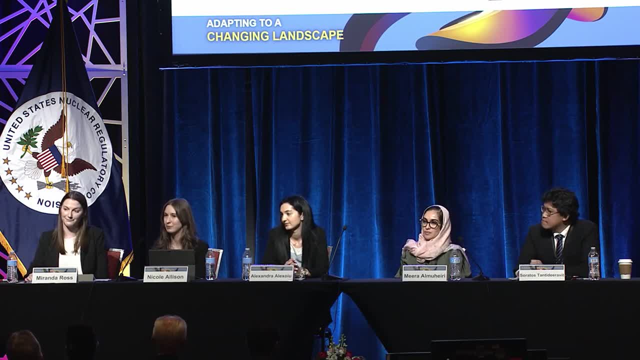 what I would add to that is, and what we've heard previously throughout this conference at the gender equity panel, is the idea of role models and mentorship and having women in STEM fields who you can look up to, And I think that's important. but 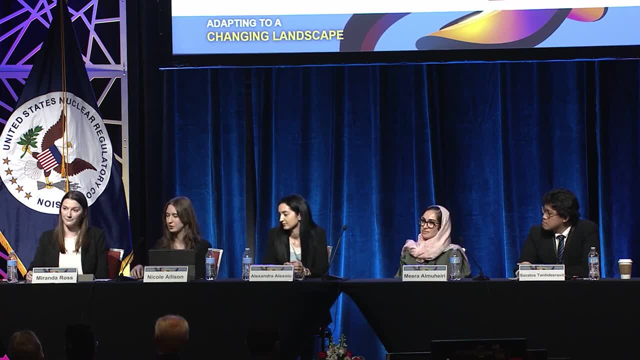 further from that, I think it's also important to have those mentors and those role models that are closer to home, in a way that you have a more direct connection with Older girls who are in, let's say, high school age and are pursuing STEM careers. 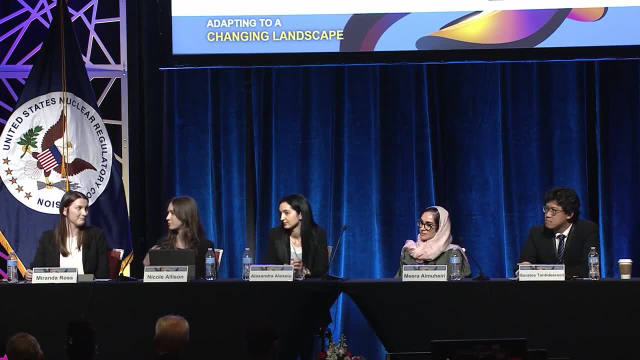 and finding those connections within your community, Spending time with those people who you can connect with on a more personal level and understand and see that, oh, they're doing this type of work. This is something I can do as well, I think even for myself now, although I'm not a. 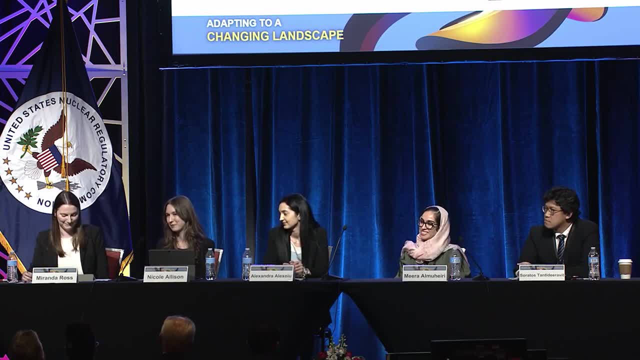 young girl anymore. in my current role within nonproliferation export controls, I'm so fortunate to have a lot of women within this group- my director, senior advisors- who are so competent and passionate and they are role models and they are people that 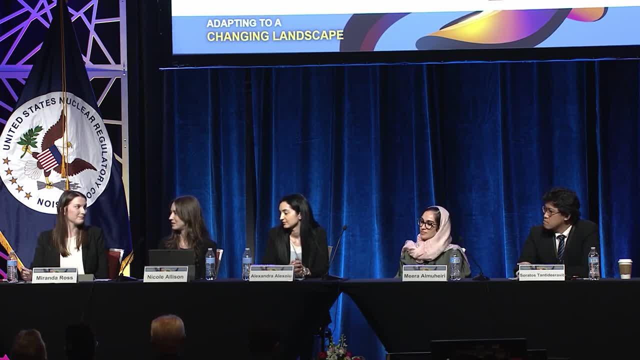 I have direct interaction with and that I have direct connections with, And it's a different type of mentor that I think is really valuable to have. I can also add that I know how easy it because I have in my family a woman working in this nuclear field, so she supports. 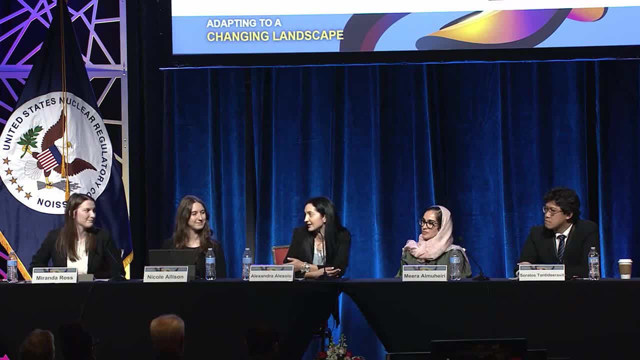 me and she learned me what is the nuclear energy, and she told me that it's a great field and you have to work to see the benefits in this field. Well, that is a great segue into the next question, which is many of you touched on mentoring. 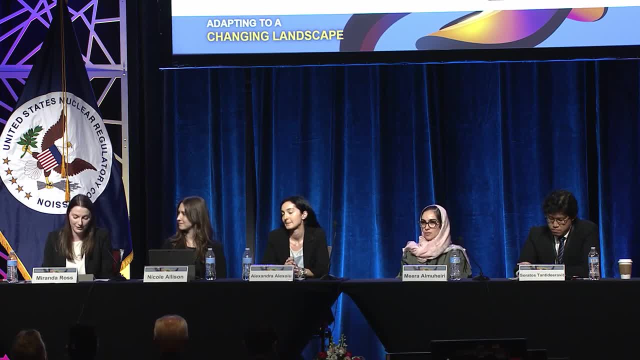 programs at your agencies. Can you share a story of how your mentor has inspired you, or how you have inspired your mentor- And I'll actually start with this one, because one of my mentors is here in the audience, so I'll give her a little shout out- Tammy Bloomer. 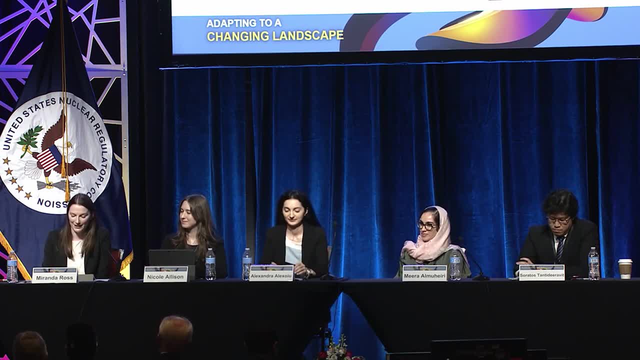 has been a career mentor for me and I can definitely say that she's inspired me by just seeing a woman in a leadership position and seeing her move throughout the agency, so I know that that has been a really great thing for me to see and have those. 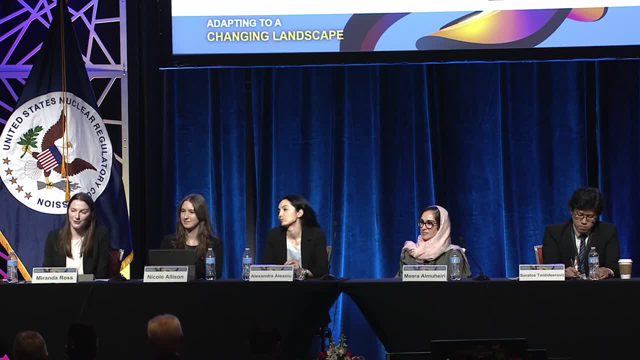 conversations about the challenges that she went through to get to those. So I'll open it up to anyone else. I can also repeat it again. if you want it again, I can add to the mentorship program. I believe that in Sanner we already have. 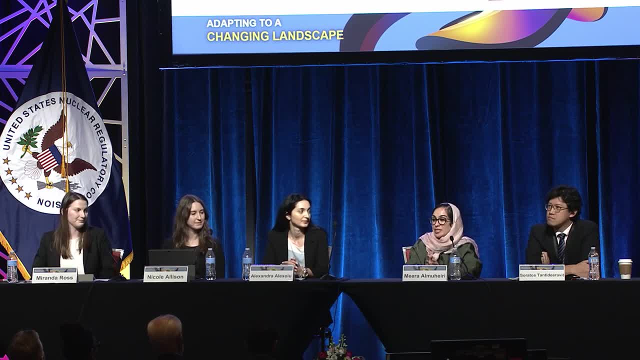 a well established mentorship program where you actually follow the lead of multiple experts. I can just walk in the hall and one of my mentors would stop me and just give me a technical question and I have to answer it, and if I don't, then I have to go back and study. 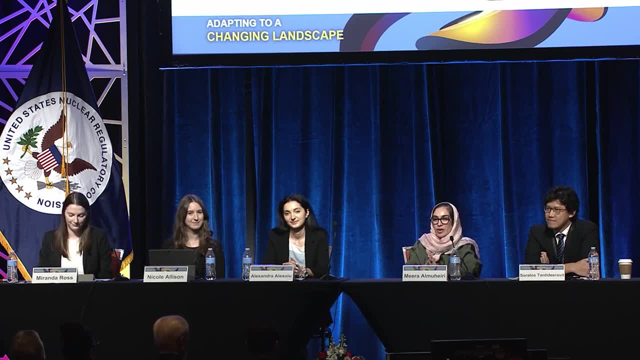 and then give the answer. Then we have you know, when we go to inspection missions or we do on job training, then we are shadowing our expertise, who come from all over the world and they always share with us the stories that they had in the nuclear field. and how can we avoid that? 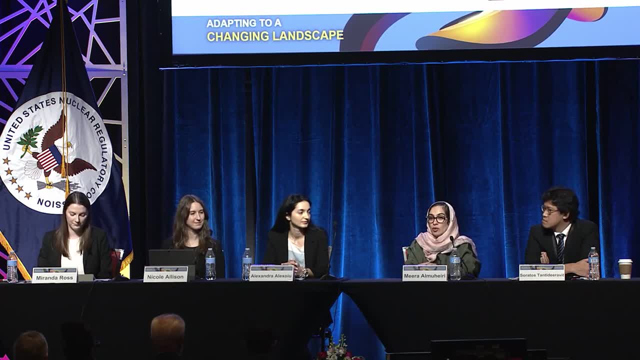 So every time I go to the power plant I make sure I wear my PPE's, because my friend told me that one like a person that was walking next to him he would have lost his eyes if he didn't wear the safety glasses. and I was like 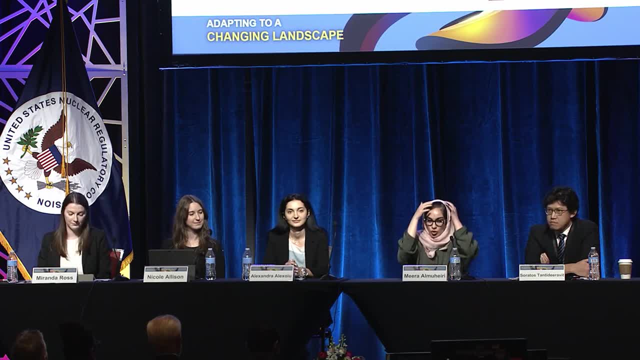 really, or you know, they're always joking around telling yo Mira, we cannot really hear because we used to walk in the plant without earring buds. so that's a kind of mentorship that happens occasionally but also systematically, and then I also have to give credit. 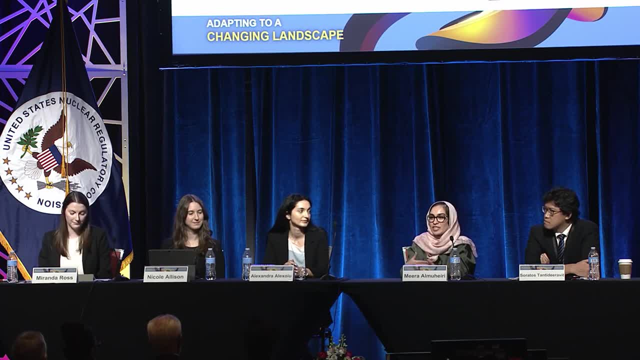 to the inspirational women that I've encountered into my journey, and one of them is Madame Vilchi, who really inspired not only me but a generation, generations of girls to pursue career in the nuclear and also here, as I'm interacting with a lot of leaders, one of who 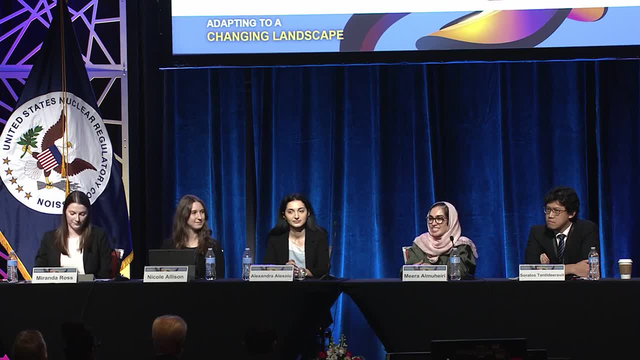 I really admired was Commissioner Wright and his attitudes towards people. so every day, we encounter an opportunity to learn, not only from people in higher positions, but also younger people, people who we work with on a daily manner. so I think we need to be open to see those. 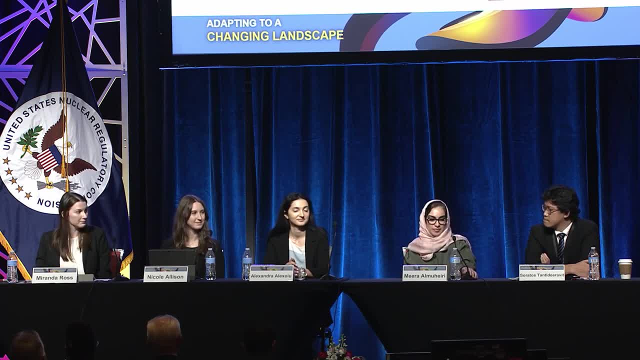 opportunities of learning. okay. so yes, as I mentioned in my slide that we have a training or mentorship in a style of brothers and sisters, and I would like to say that it helps not only the teaching and the transfer of knowledge, but it had kind of building trust between 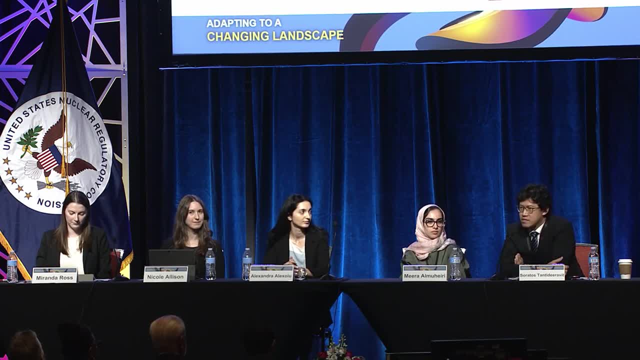 our supervisor and the younger staff, and so it's kind of a relaxing conversation which helps promote the exchange, not only, you know, the top down transfer of knowledge, but also the bottom up, that, the feedback to the higher level as well. I'd just like to add to that: 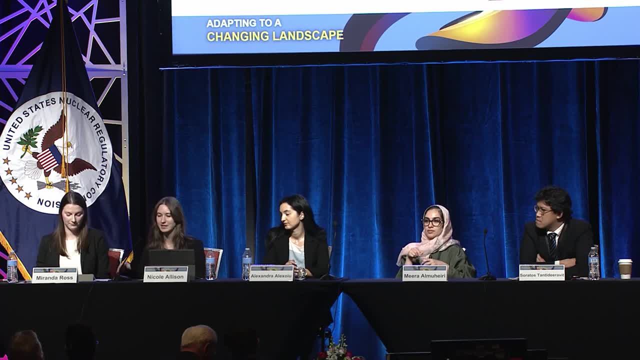 I think that's a really good point, Sortos, on that level of trust that comes from establishing good mentorships, where you are working together with those people who are your role models or are the people that are transferring their knowledge to you or acting as your mentors. 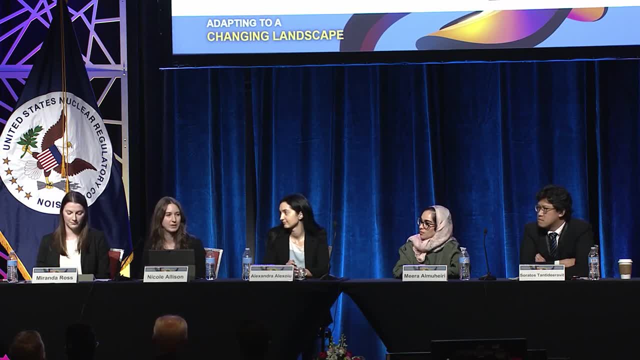 but also breaking down those barriers of formality- sometimes right- and connecting on more of a personal people to people level right. and how having that type of relationship and opportunities to work together where you are receiving knowledge but also right, breaking down those barriers again and connecting on a more personal level are so crucial to having 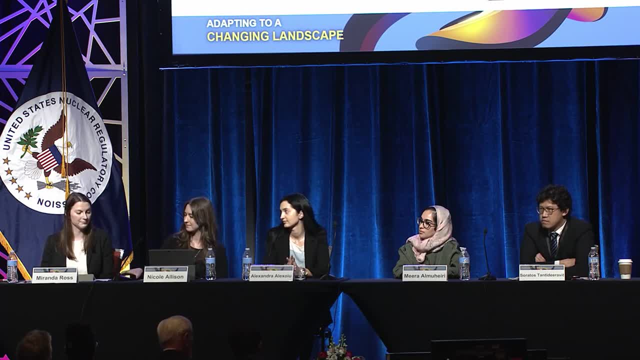 good mentorship experiences. alright, thank you. so I'm going to start this question with Sortos and then we'll open it up for anyone else who wants to add: from your experience, what have you done or what has your agency done to help you feel connected and integrated into the? 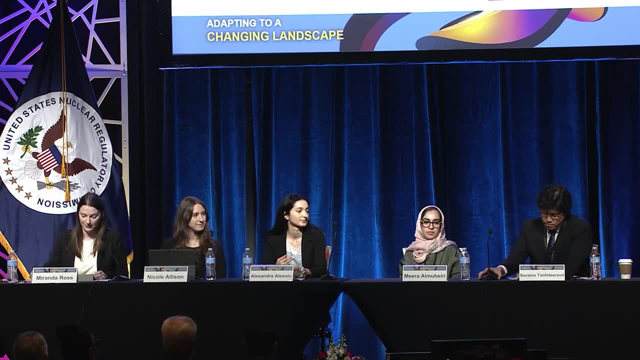 regulatory world. okay, so firstly, when I joined the office, it is a part of the civil servant, the regime, and we have the training program as for every civil servant, which kind of gives some introduction and principles for us to what to do and how the system works and what is the. 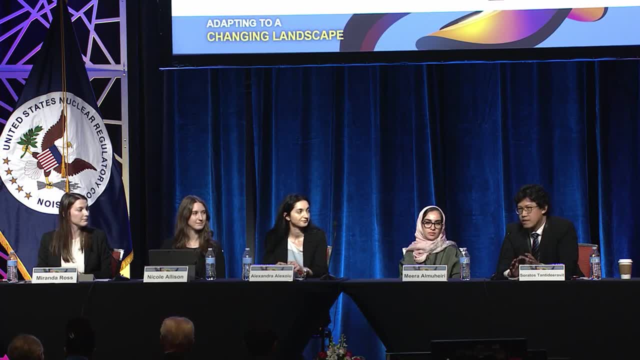 objective of our work, that's for the general aspect of being a civil servant. and then on the OAP. for the OAP we have, so the management. they always have the clear description of the roles and responsibilities of each of the department and each of the personnel. 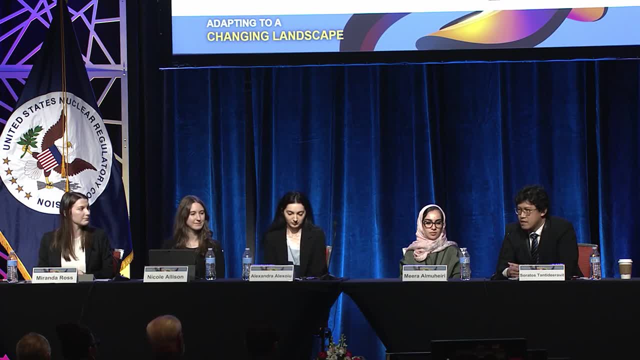 so that is kind of helped me understand the roles and responsibilities and helps me kind of know what to learn and what to improve myself on which of the expertise to build. thank you, does anyone else want to add to that? I think also adding to Sara to send, also agreeing with that. 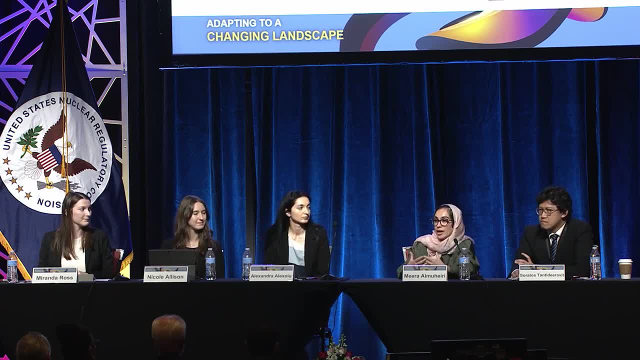 point is that we learn how we are relevant to the regulatory philosophy or regulatory world through training, systematic training, but then it takes an extra action from leaders to kind of tell us why we're learning, what we're learning and how we can use those learnings within our 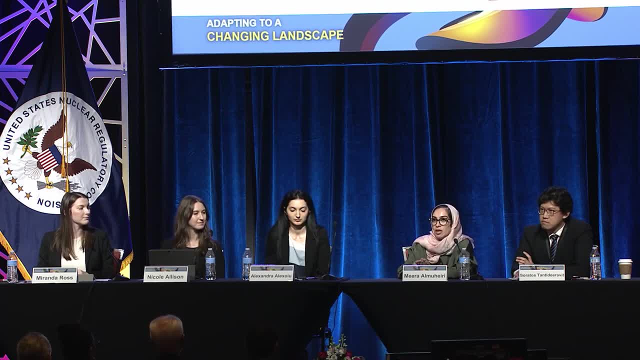 job, not only on the technical level, but also from a strategic level. so, for example, DJ Krister. he always walk around the offices and ask us: what are you doing? how can we elevate that within FANR? not only within your own divisions, our directors, they always 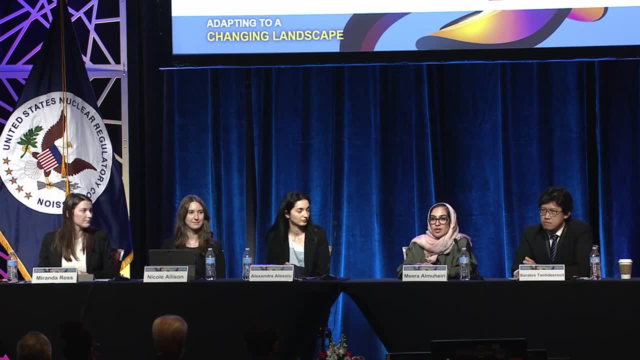 come to us and tell us we have these issues? how can we work on these issues and finding those connection between what we learn and our fairly new expertise to with regards to nuclear, and then looking into how things can elevate to work on the strategic level and having 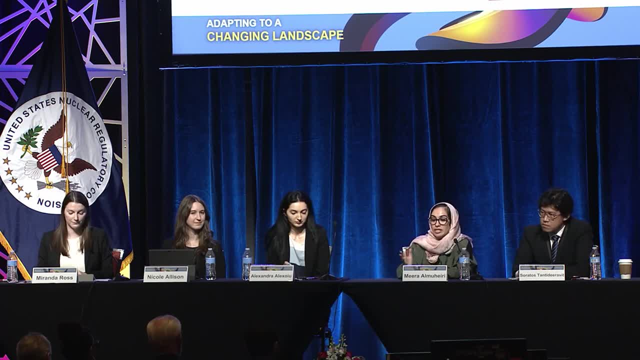 the more of the bottom up connection with our leaders is kind of making us feel connected to the world and making us understand that even the small things that we do on a daily basis, that we think they are routine, they're not routine and they're actually very important. 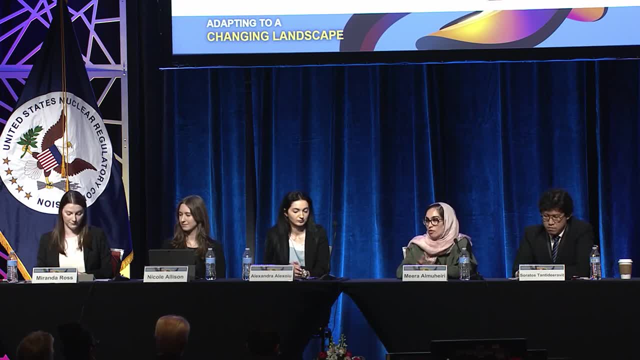 because they are eventually contributing to the bigger picture and the bigger goal of the organization. thank you. so, on a similar theme, what excites you about your future as regulators? and for this one, I'm going to ask you all to give an answer. so I'll start, and then we'll just go down the line. 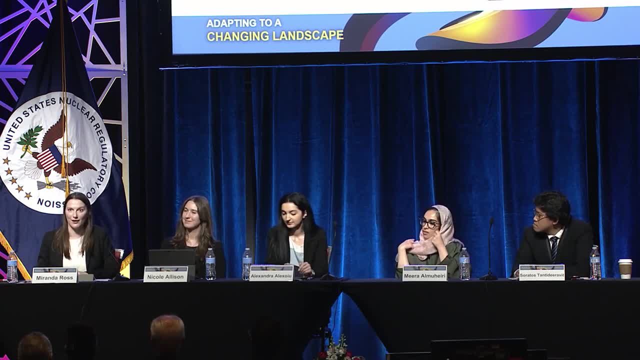 for me, the NRC's mission is something that over my last year and a half, I've really grown to feel more passionate towards what I did at the NRC, not really knowing what the NRC was and really understanding how we affect the nuclear power plants. 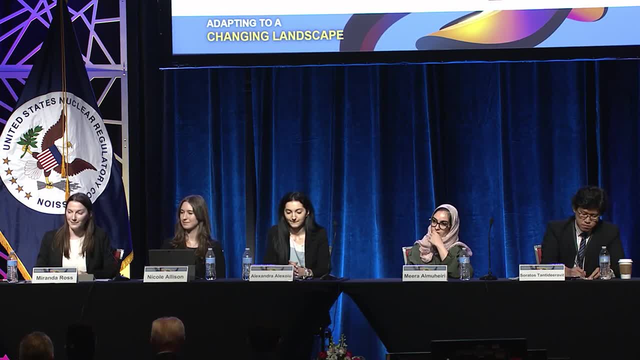 and materials in the US is something that has really grown my excitement about working here and I think it will continue to grow. thanks, Miranda. when I think about the future of my career as a regulator and where I am now and what really excites me- and again I think a theme- 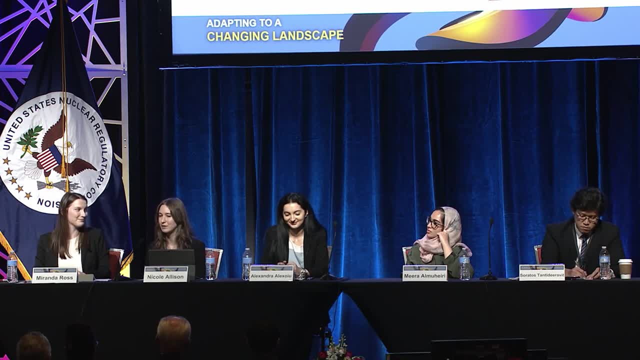 that's come up often throughout this conference in the last couple days is that we are really entering a new time, a new landscape for the nuclear industry. there are going to be big changes and there are going to be a lot of challenges that come along with that. 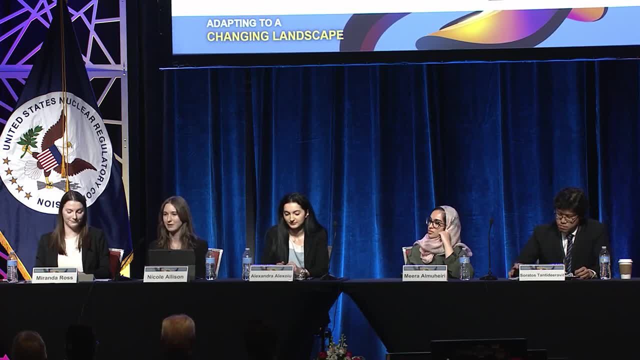 but it also calls forth, I think, a lot of creativity and a lot of questioning in terms of how our existing framework and our existing policies are going to apply in this new landscape, and the idea of solving those problems and facing those problems- maybe sometimes daunting- also very much excites me. 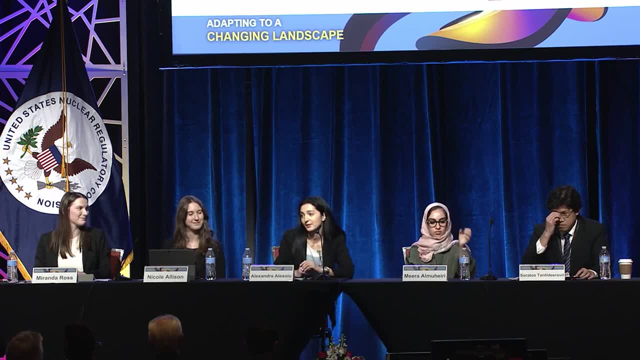 so I think it's about the impact, because within the institution we contribute to the fundamental safety objective, so more specifically, specifically the way in which we contribute to ensuring safety and security of nuclear facilities, which is vital for public health and environmental protection. so for me, I remember 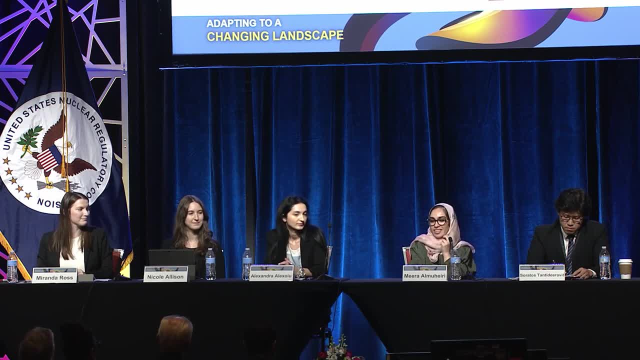 that every time I attend a training course, one of our experts would tell us: imagine if something bad happened in the nuclear power plant. how would you go back to your family and friends, knowing that you have contributed to this? and this question keeps resonating and keeps motivating me. 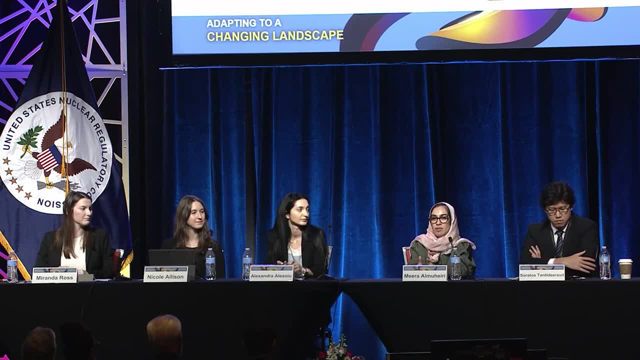 to look at my job not as a 9 to 5 job, but something that we really need to guard with responsibility, with commitment, because we are responsible for the safety and the security of the nuclear power plant, and I feel like this should be really the motivation. 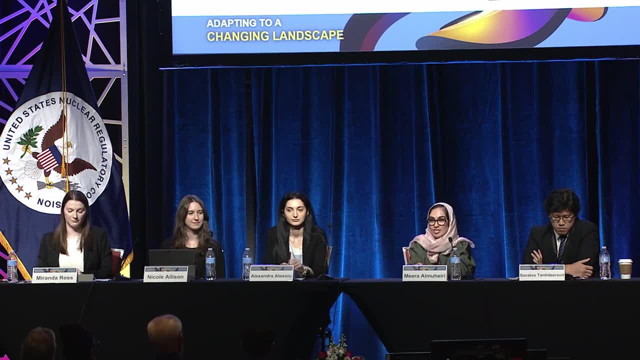 and the reason why we wake up and we decide to go and work as a regulator. so, yes, I would like to second what Meera said in her presentation, that a nuclear regulator is a very dynamic job and very international, and so, for me, I work in Thailand. 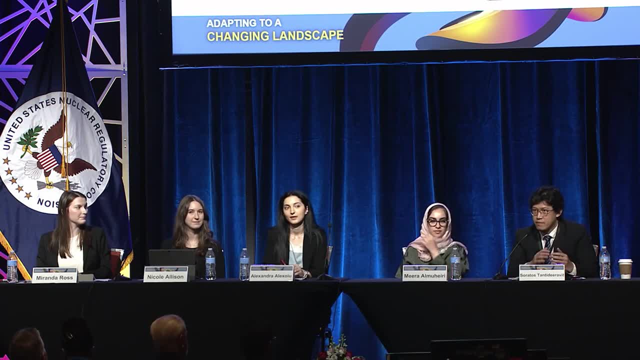 but it's not only the industry in Thailand that inspired me, but also I see what other countries are doing and I see the potential that this technology can be used in Thailand or we can learn so much from other countries. so that is the continuous learning for me. 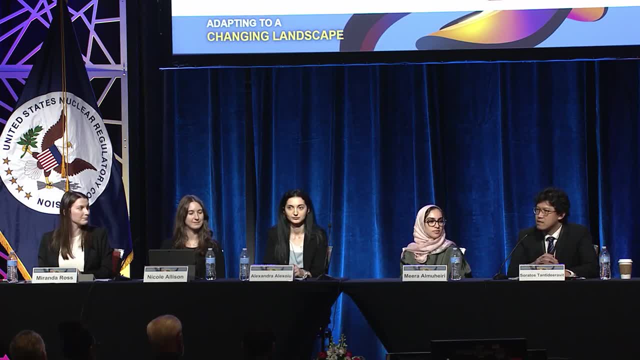 is one of the motivations that I enjoy this job, so it seems like there is a pretty similar theme there which is really great to see along that this one is going to be for Nicole. are there any changes in our regulatory culture needed to attract or retain young professionals that you can think of? 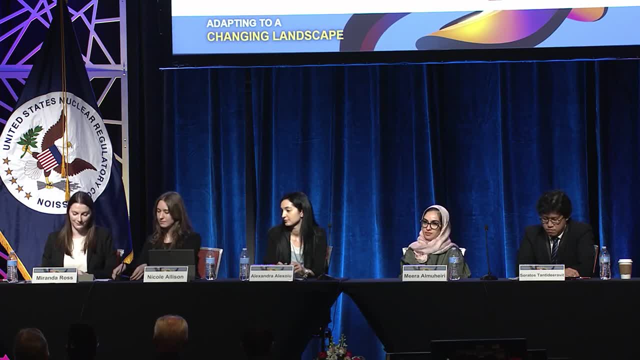 I would say- I am not sure if I would say the culture itself, but if I put myself back in my shoes as a university student finishing my third year, looking at a co-op or internship at, maybe, one of the power plants is what I imagined for myself. 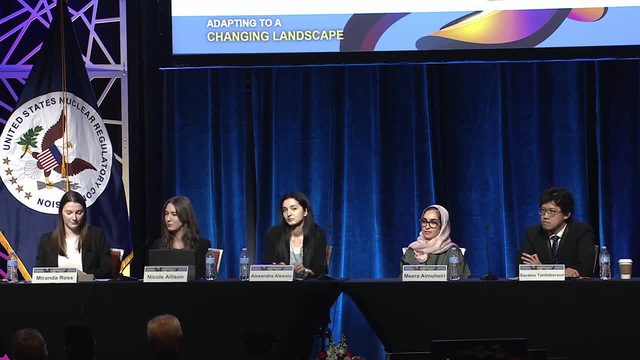 but where I ended up is actually the nuclear regulator, the Canadian Nuclear Safety Commission. what really spoke to me, and I think we could improve on in some ways, is what is sometimes maybe a lack of awareness or a lack of understanding in terms of the scope of work. 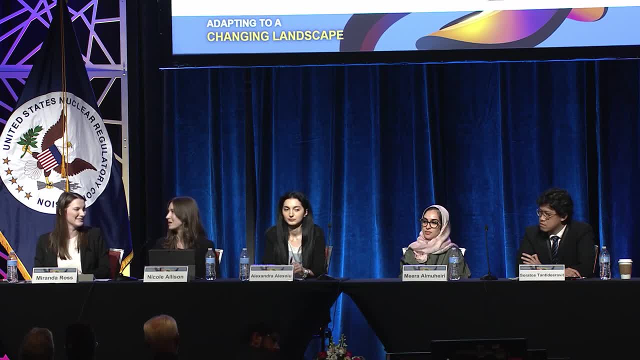 that a nuclear regulator performs. I feel like there are, in some cases, maybe a preconceived notion of what working for the regulator means or what it can't or can't encompass. but what really struck me as I joined the CNSC and I rotated through various divisions, 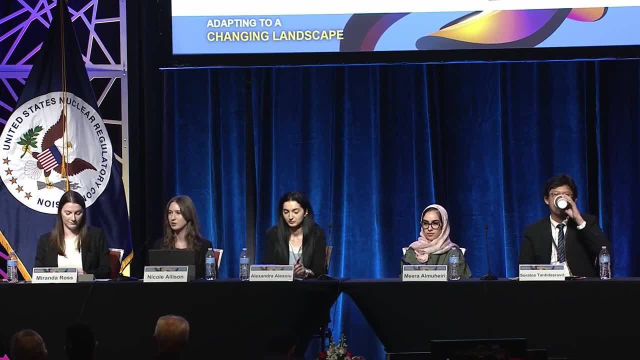 during my internship is that it is such a broad swath of research, of technical work, of where I am now, policy work combined with that technical knowledge. there is something for everyone, I think, and I think a big part of attracting and retaining youth or new staff going forward. 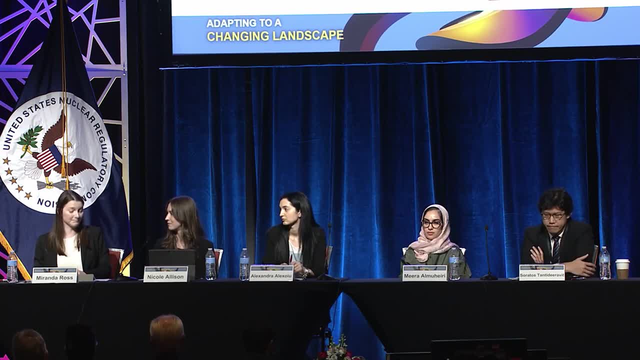 will be to improve what is a lack of awareness in terms of what this work encompasses. Thank you, yeah, I completely agree. I think that we need to, in all areas, really show that there's more to just desk work when it comes to being a regulator. so that's great to hear. 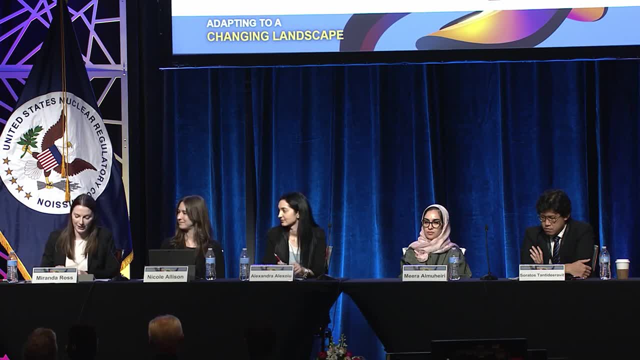 for this one. I'll leave it up to anyone who wants to jump in in your experiences. what are the best ways to facilitate knowledge transfer from older, more experienced employees? okay, I'll start then. so for me, one of the best things that I found was really just sitting down with more experienced. 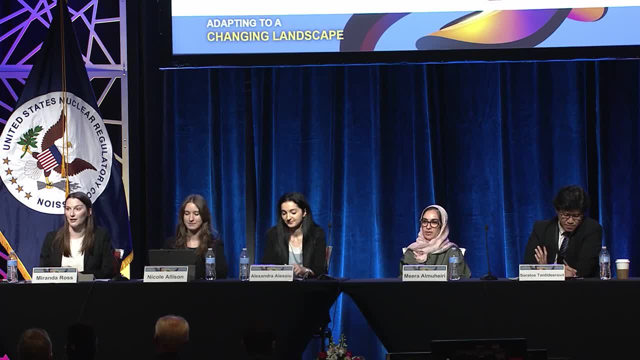 folks and just talking to them. so many people have a ton of stories about either plants that they were at when something happened or a materials site, and if you can just sit down and just get them to talk, you will learn a lot. and then what I like to do is: 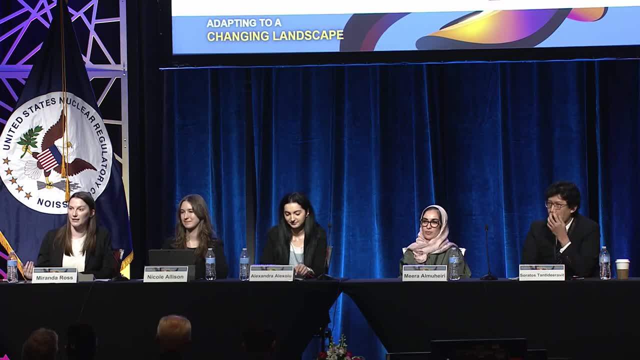 I take what I learn and we have an internal Wikipedia site for the NRC and I put that into that site so that way everyone has access to this knowledge, because if I'm the only one getting it, it's not helping anyone. so we need to really 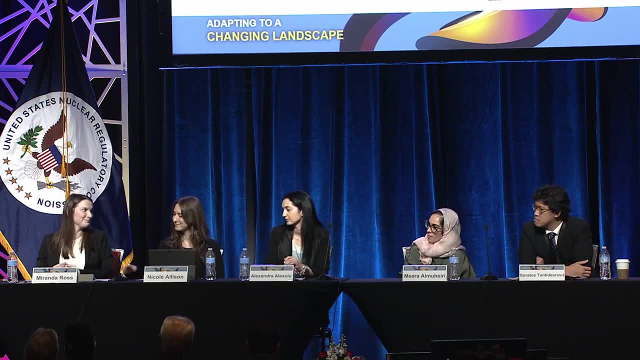 get it and then cement it somewhere. I agree with you fully. I think there's such a challenge when it comes to knowledge transfer, when we're talking about the knowledge that's in people's heads, that working level, understanding of how we do stuff, and the historical knowledge that comes along with. 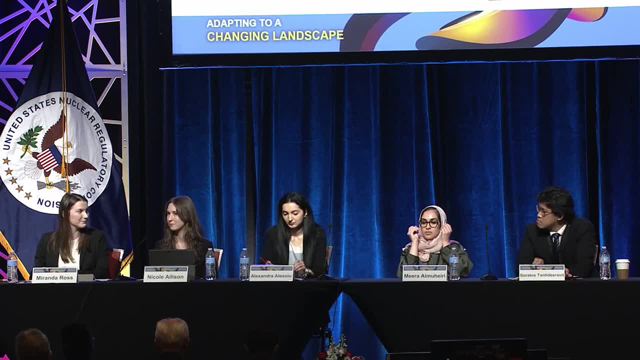 experience and it's very difficult to formalize that or capture that in certain ways. and I think, as you pointed out, one great way to do that is to sit down with those colleagues and sit and listen to their stories and listen to their experiences, another way which I touched on a bit in my presentation: 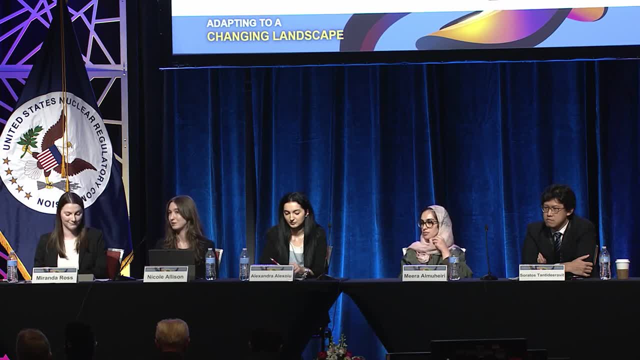 is. I really love working alongside those colleagues who have knowledge that I hope they do transfer to me, because I think it's in those settings where a lot of the idea of you don't know what you know comes out: knowledge and information that these people have that they don't even realize that they have. 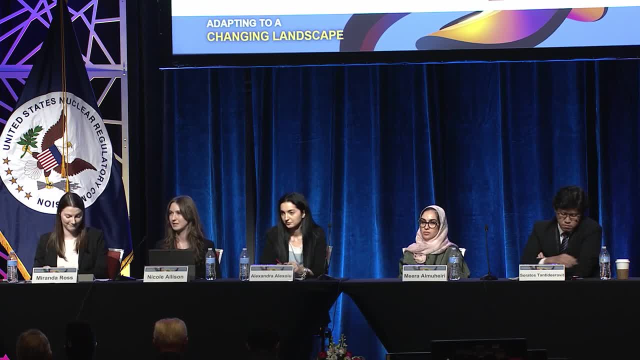 it's become so ingrained in part of their knowledge base that they might not even think in one setting to sit down and explain this. but as you're going through the work together and it comes up, they go. how do we explain that, right? Yes, so I think. 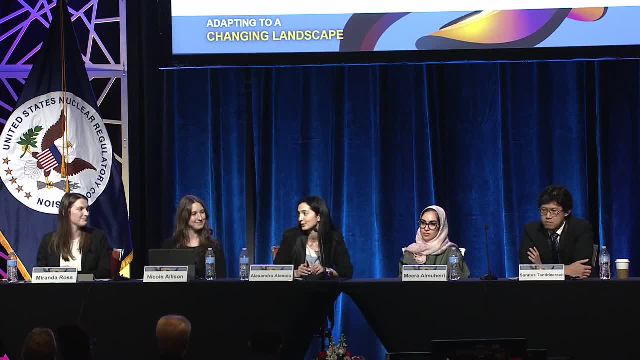 through the mentorship program. it's very important. you have to learn and to get familiar with your mentor, and also I think that the teamwork is very important and also in our case, we perform for the inspection. for example, we perform mixed group from different sections, so you can. 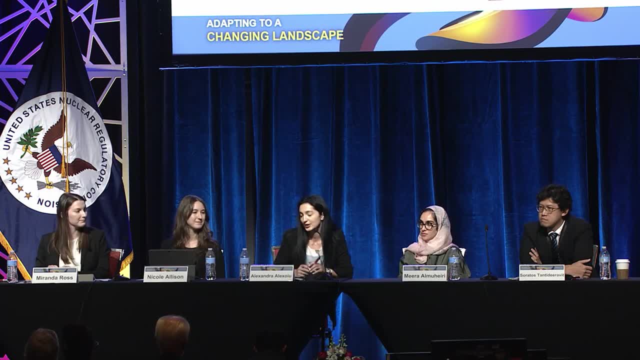 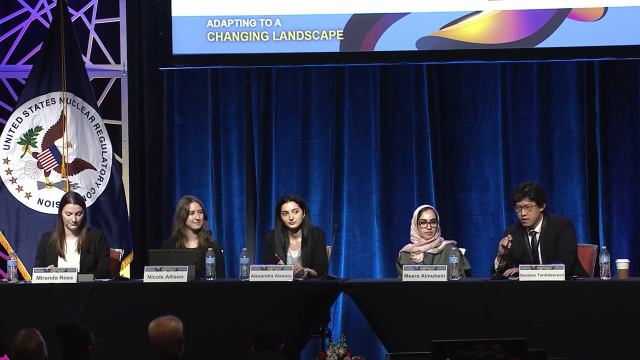 learn and get more experience from this. I'd like also to add: for the knowledge transfer. I think it needs the two sides to be committed to that: experts who are willing to teach and also new joiners who are willing to learn for it to be successful. so for me, 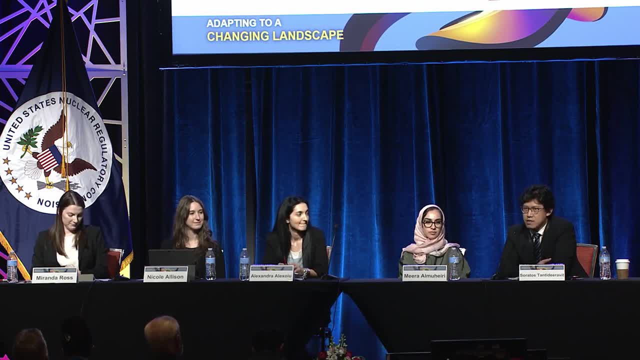 I believe that to be to become an expert, we need to constantly working on something, to really spend time with it and to have a coach to help us. but the most important thing for knowledge transfer from senior officer to young, I think it's the inspiration that they can provide, because 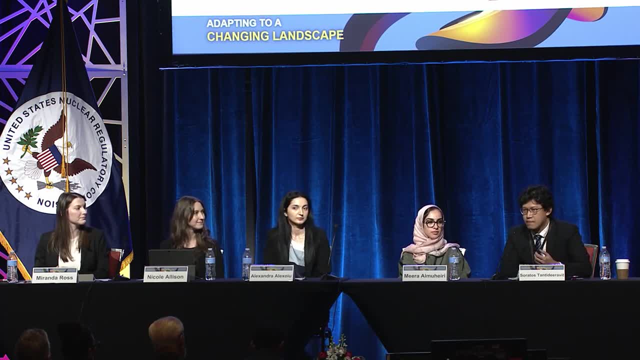 being the role model or being, yeah, telling their stories. that could inspire the younger generation to pursue more knowledge. So, on the note of knowledge management transfer, I'm not sure how many of you have remote work options, but if you do, do you feel that it has been? 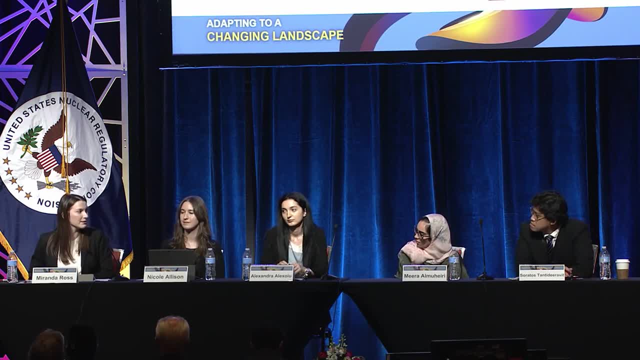 impacted with how you're able to transfer that knowledge management? Yes, certainly, although I mean for good and bad in some ways, of course. right, I mean there's that element of you know there's a lot of knowledge transfer. that just happens naturally when you're in the same place and you're talking to each other. 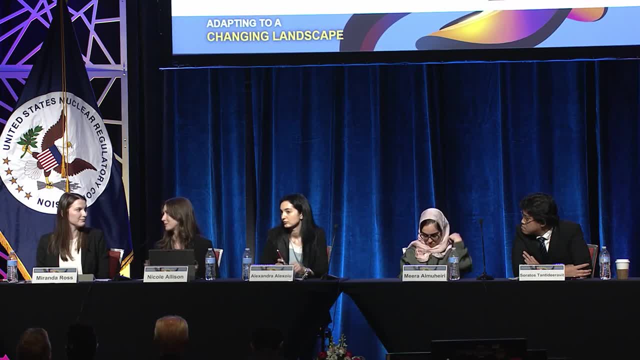 whether it's during work or over your lunch break, you're in the same place and you're chatting about things, right? I mean? one of the positives of remote work in this hybrid environment that we now live in is that it does make even events like this so much more accessible to, let's say, 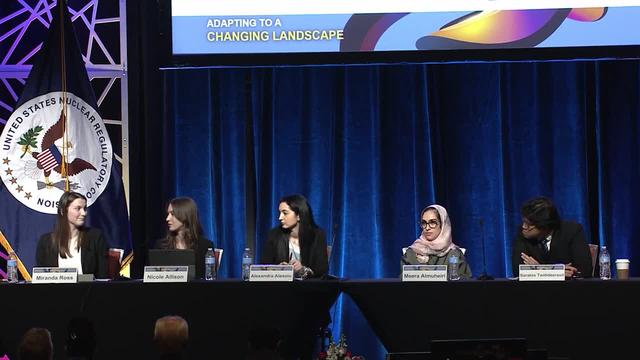 regulators who want to listen on this panel, but they don't have the resources within their organizations or their countries to send them all here. of course, right, but now we have the opportunity to share this more widespread- virtually, I mean even thinking within my team. more specifically, there have been processes that we've 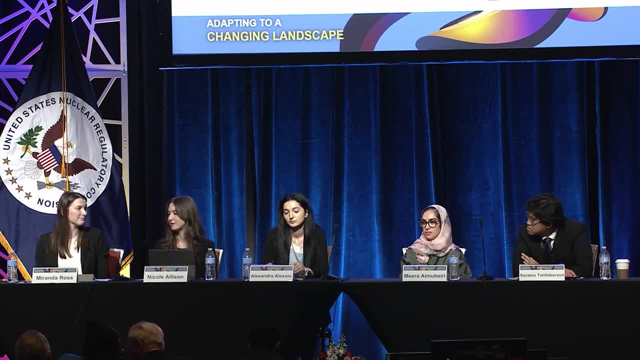 incorporated now in our day to day or our routine work. right on a weekly basis now we designate a one hour period where we all get together, all of the licensing staff come together and we talk about cases we're working on or challenges. we have questions. we have that we're hoping our colleagues 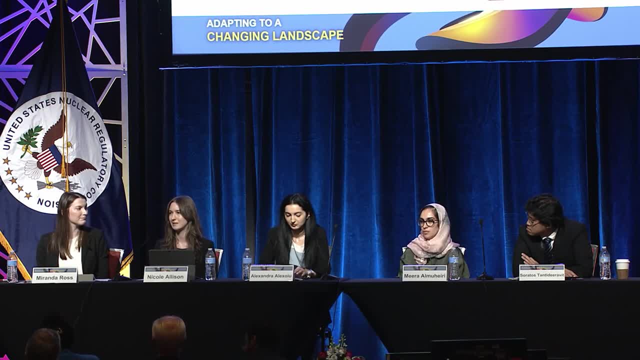 can help us answer, or even just explaining difficult cases, that I figured this out last week and this is how I did it right. so I think there are pros and cons to an environment like this and it's about finding those opportunities to take advantage of what pros there are. 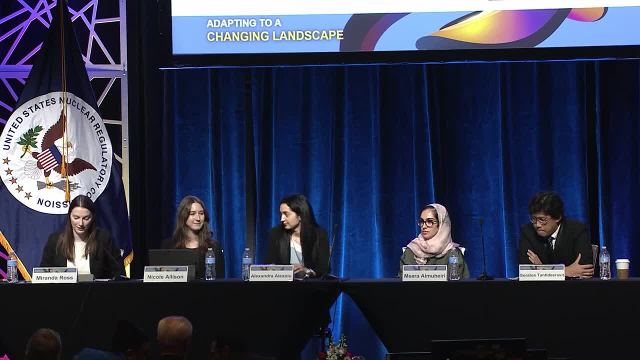 Okay, great, I think we have time for one more question, so I'm going to open this one up to everyone, because I really think it's a great question. if you could give your 17 to 18 year old self one piece of professional advice, what would it be? 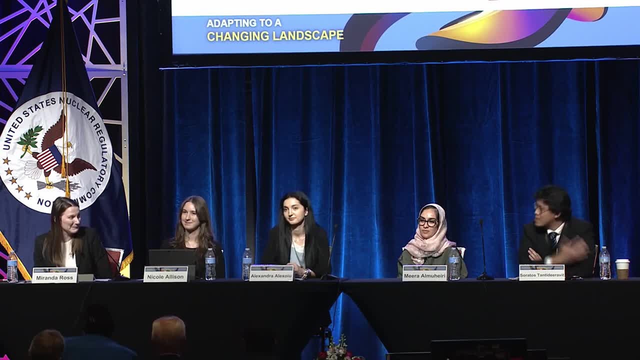 Sure, Okay. so for me, if, if someone wants to work as a nuclear generator, I would say that to have questioning attitude and to be able to ask the right question, direct question, but in a friendly manner, and that will help promote conversations, discussions, and I think we can get a lot of benefit. 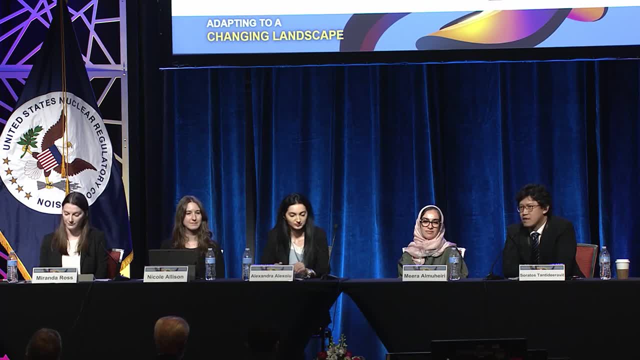 from exchanging ideas, yeah. and to be able to learn from experience or mistakes, from your mistakes or other people mistakes to help improve you know, lesson learned and safety: yeah. Should I go next? Yeah, anyone who wants to jump in on this one? I think I would tell my younger. 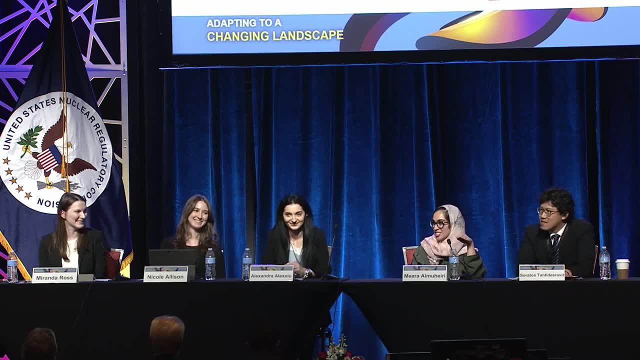 self, relax, everything will be okay eventually. I think we stress a lot, maybe trying to find out what is our passion, what are we good at and are we making the right decisions or not, and I think what we really need to focus on: exploring things that make us happy. 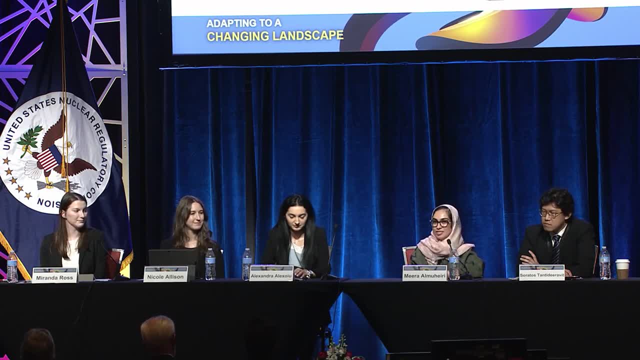 whether it's a class, a major, a profession. if you think that this is something you want to explore, go ahead and explore it. if you failed at it, that's okay. you have so many other things to try, so be open, enjoy the journey and everything will be okay at the end. 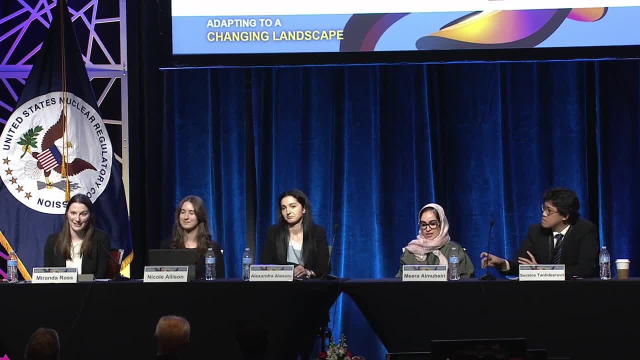 Alright well, at this point we're at the end of our session, so I just want to thank our presenters for your presentations and the really insightful conversation that we were able to have today. I know that I took a lot out of it, and I'm sure everyone else did too.